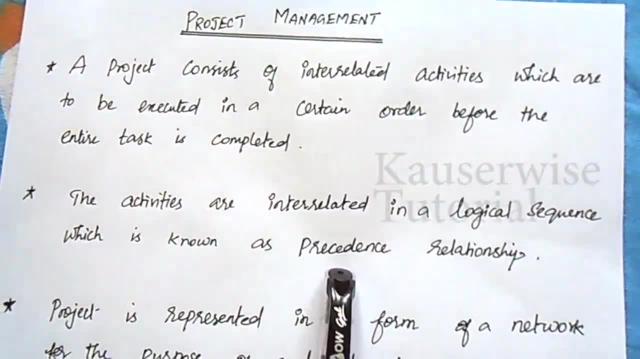 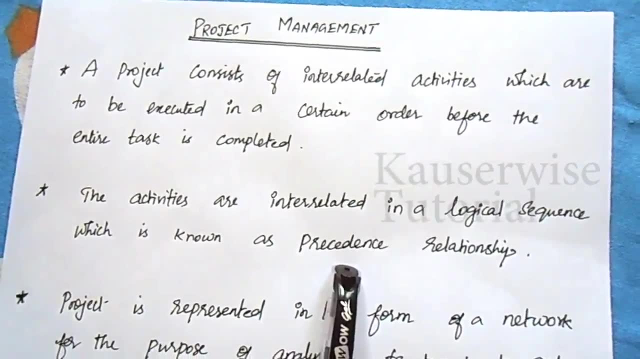 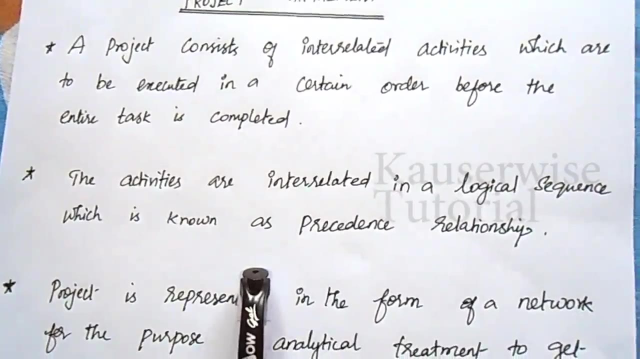 as president's relationship. President's relationship means, for example, if you take one particular project, it has five activities, For example A, B, C, D and E. So after completing A, that is the first task. first activity is A. After completing A, then you will move on to B, So here, so after completing, 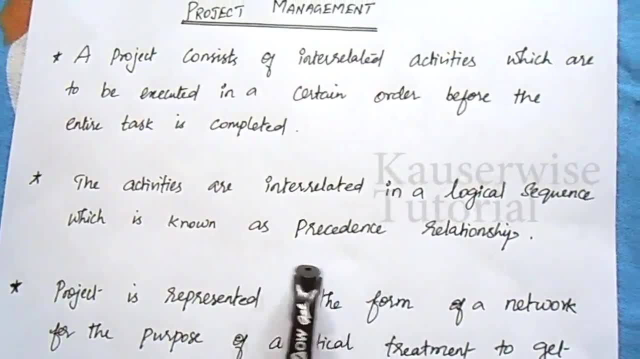 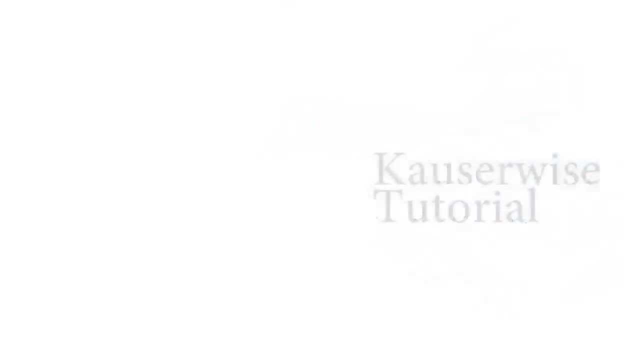 A, only you can able to move on to B. Here we have a relationship between A and B. That relationship is called president's relationship. So this we will see. with the example. A project is represented in the form of a network for the purpose of analytical treatment, to get. 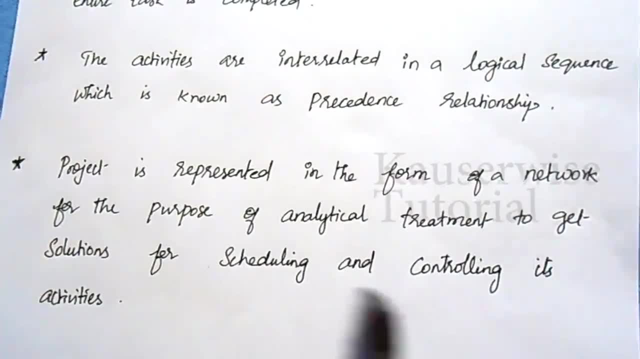 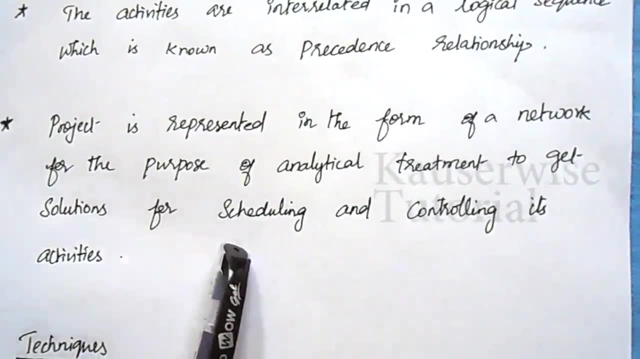 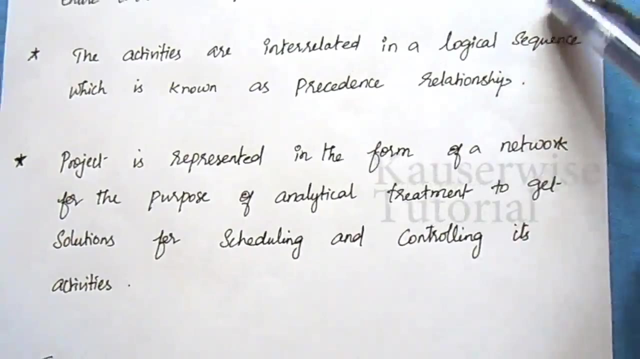 solution for scheduling and controlling its activity. A project represent in a network form in order to prepare or find the solution for scheduling and controlling its activity, So we need to apply network method. So these are the basic concept of project management. In this project management it has two. 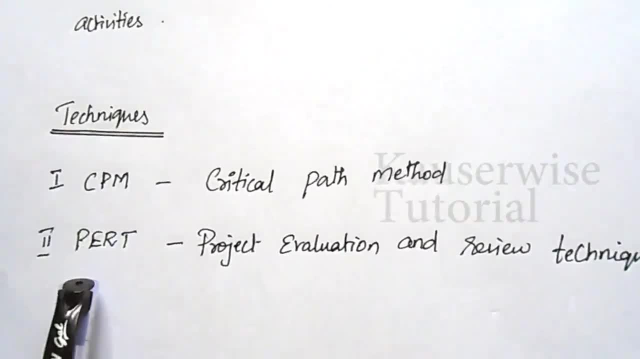 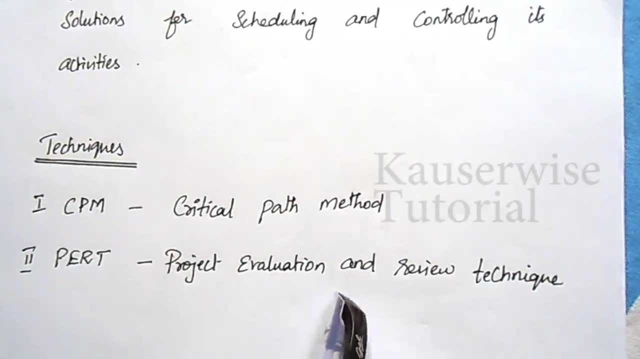 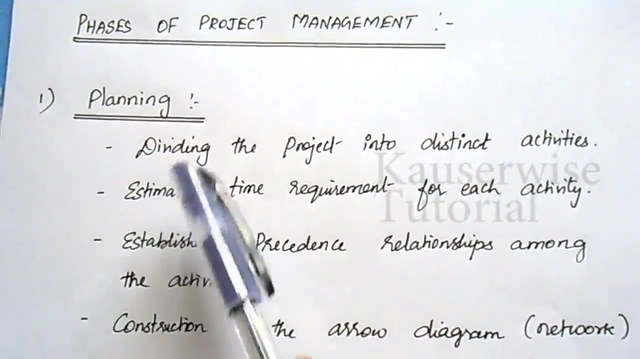 basic techniques. First one is CPM and second one is PERT. CPM means critical path method- and the second technique is project evaluation and review technique. Next one is phases of project management. So it has three phases: The first one is planning, second one scheduling and third 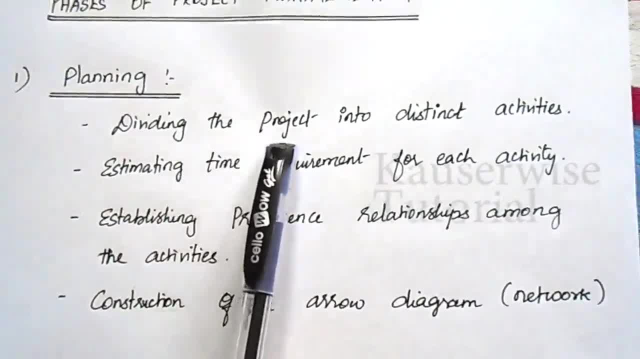 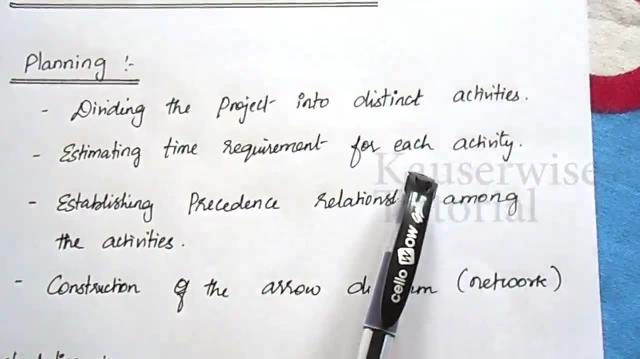 one controlling, So under planning, dividing the project into distinct activities, and second one estimating the time requirement of the project. So the first one is planning, the second one for each activity. So how much time is required to complete each and every activity that we have? 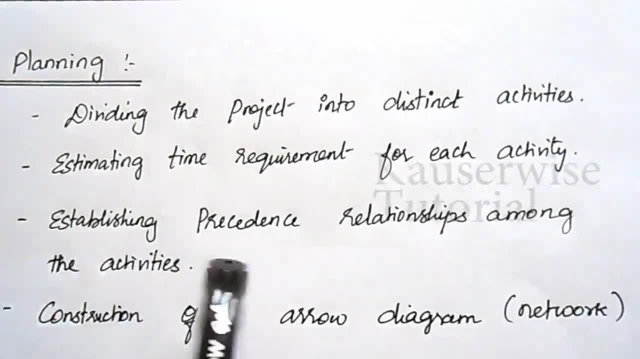 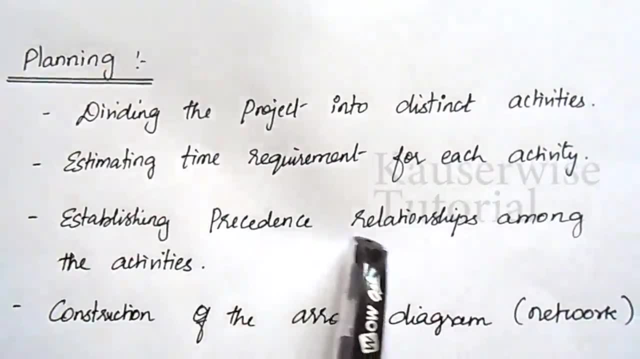 to decide in advance. Next one: establishing president's relationship. The president's relationship is very, very important, So we need to establish the president's relationship among the activity. This we will see with the help of problem. And the last one is construction of the. 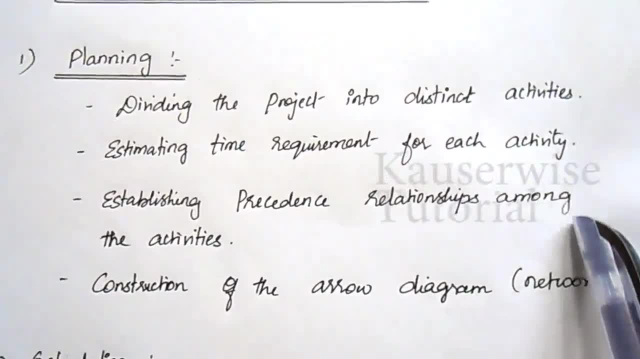 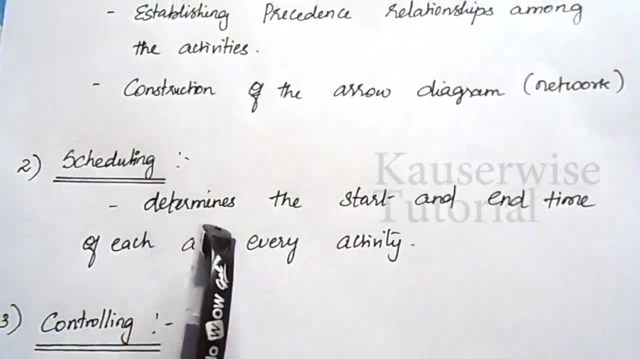 arrow diagram, that is network. So these are the different parts in planning activity And the next one is scheduling. So the first one is planning, the second one scheduling and the third one controlling. So after planning, the next thing you need to schedule, which determines start and 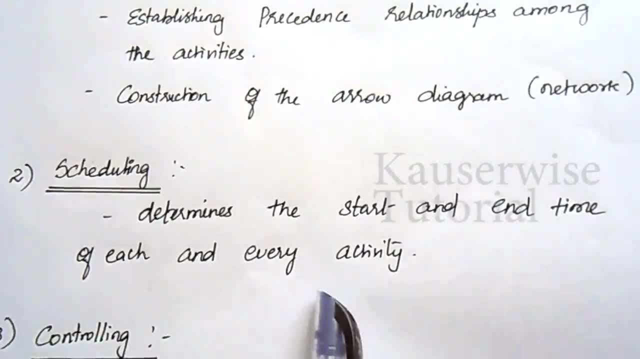 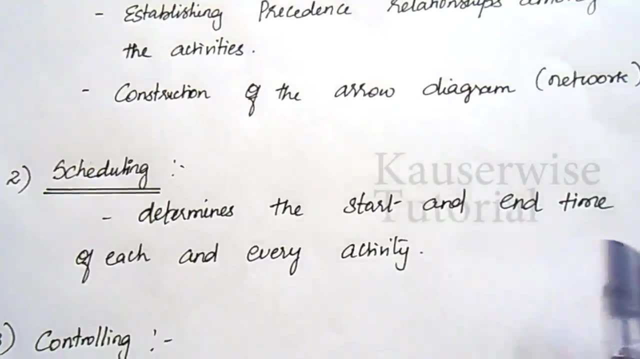 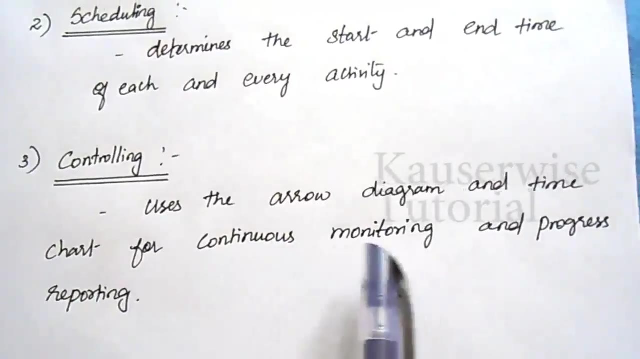 end time of each and every activity. So you have to determine the starting time of each and every activity and you have to determine the end time of each and every activity. is called scheduling, And the third phase is controlling. Uses the arrow diagram and time chart for continuous monitoring. 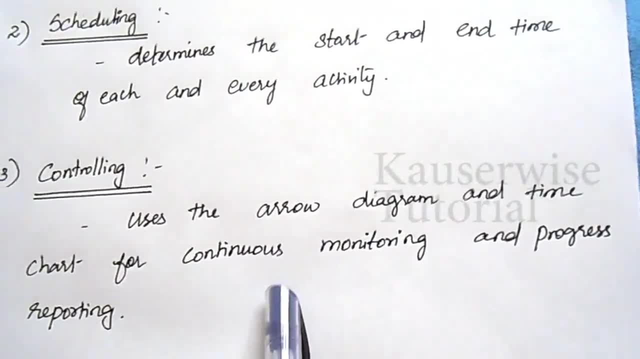 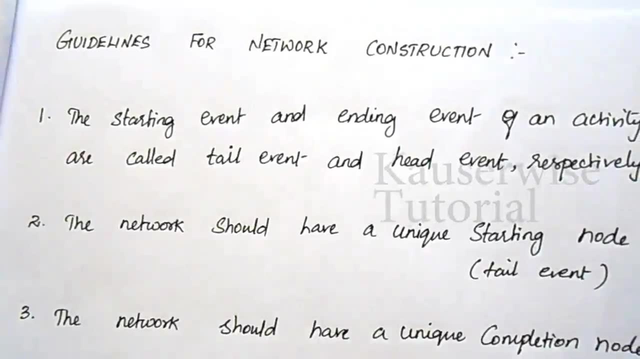 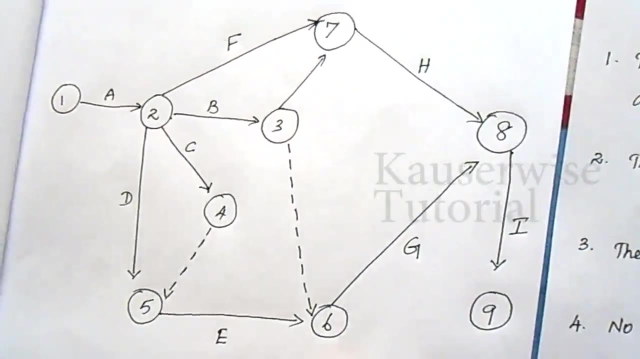 and progress reporting. So this is also one of the phase which comes under project management, that is, controlling. So these are the three phases of project management. Now let us see the guidelines for network construction. Here we have one model: network construction. With the help of this model. 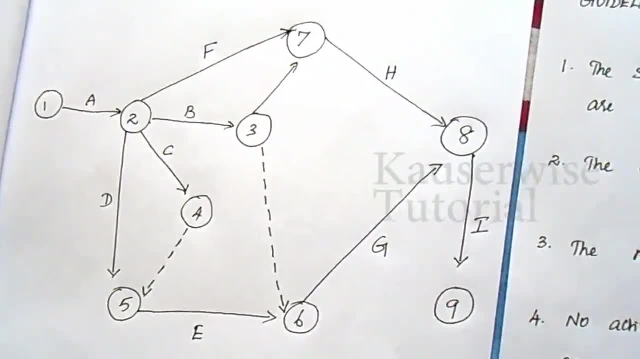 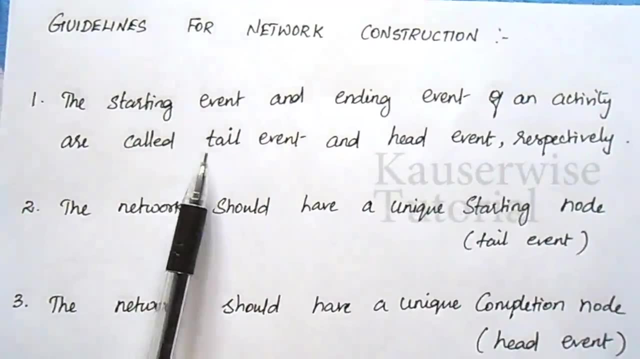 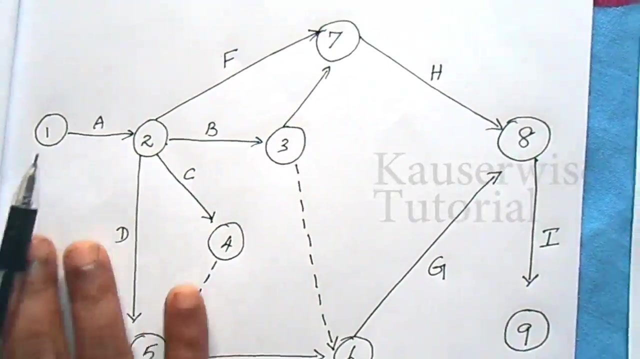 we are going to learn guidelines for network construction. See the first guideline. the starting event and ending event of an activity are called tail event and head event respectively. Look at the module. This is the network construction. Here we have the starting event and ending event of an activity. So we have the starting event and ending event of an activity. 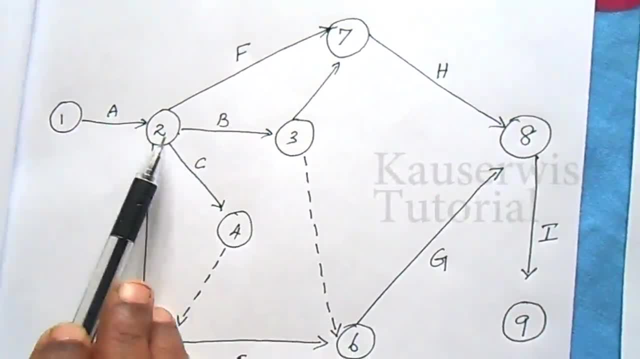 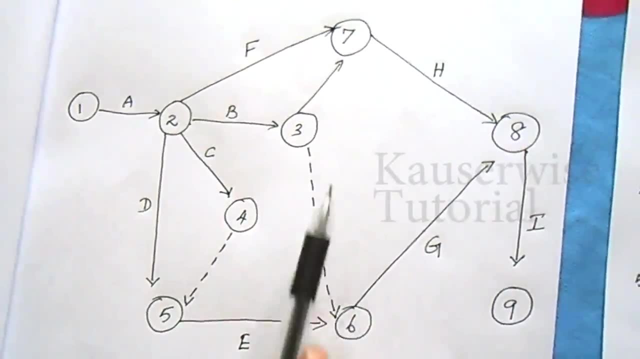 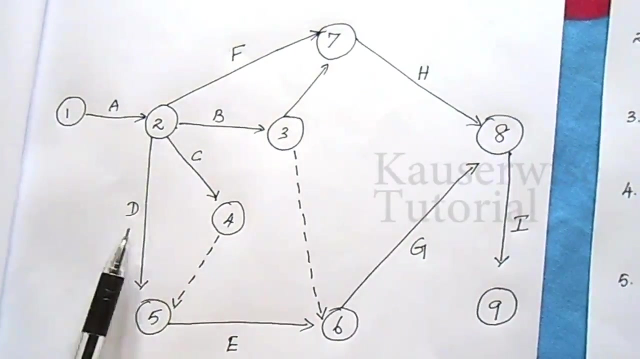 We have a different activities. So these are the things are called node Node 1, node 2, node 3,, 4,, 5,, 6,, 7,, 8 and 9.. So these are the activities: A, B, C, D, E, F, G, H, The last activity. 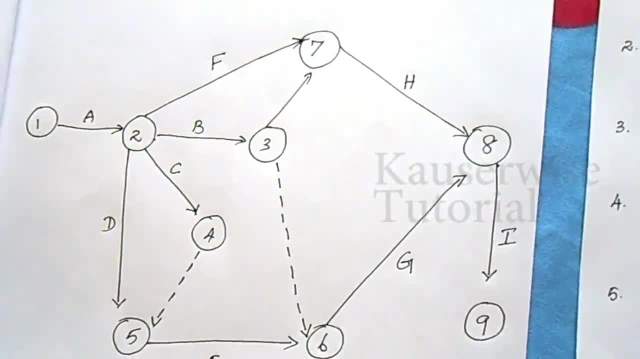 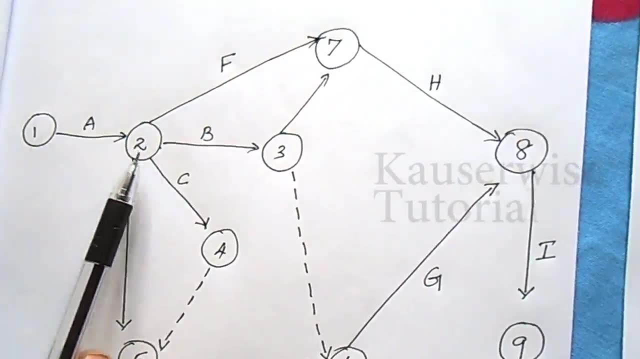 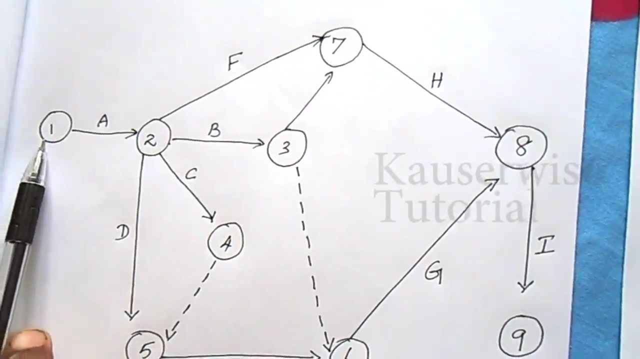 is I. So these are the different activities in the network construction. Okay, so the first point is The first guideline is: the starting event and ending event of an activity are called tail event and head event. The first one is called tail, The completing event, the completion event, is called head event. 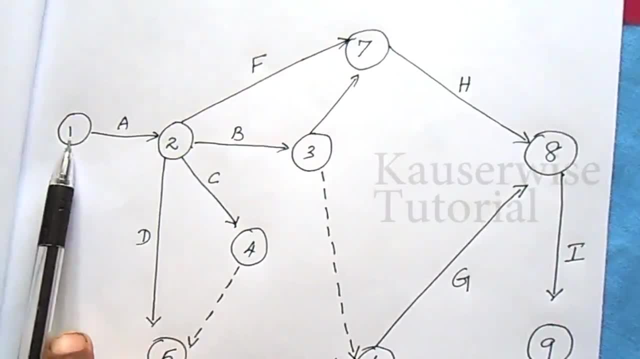 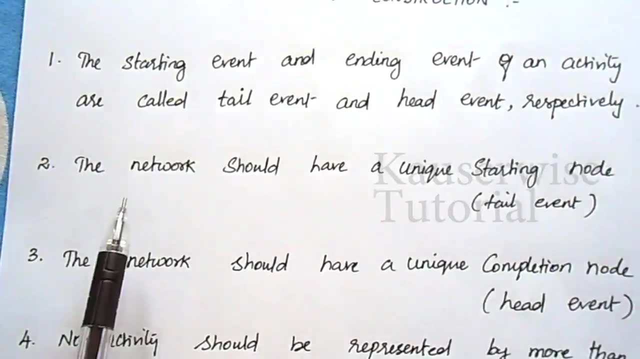 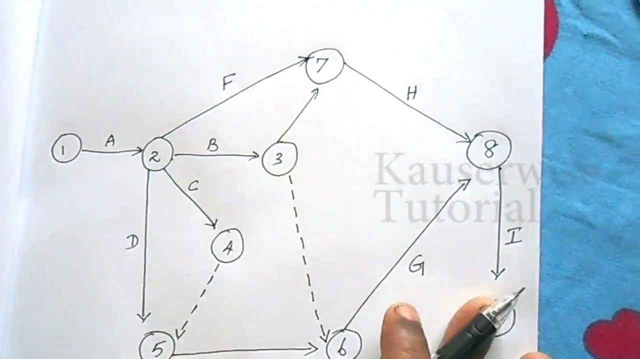 So, in order to complete the first activity, we need to have two nodes, one and two. This one is called tail, This one is called head. Second one: the network should have a unique starting node, That is, tail event. For each and every activities we need to have a unique tail event. 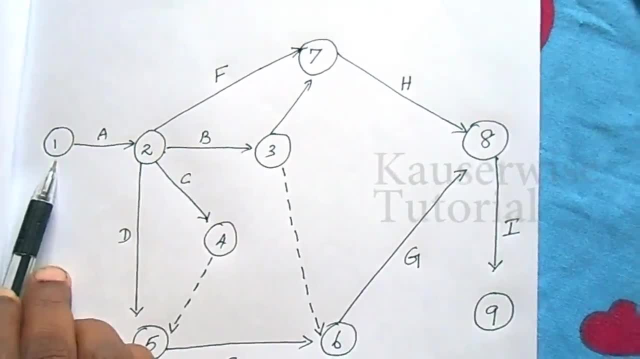 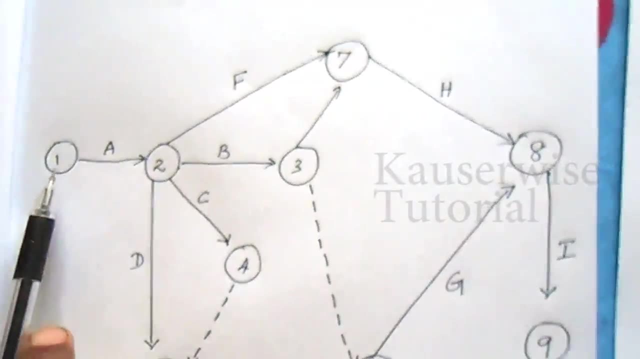 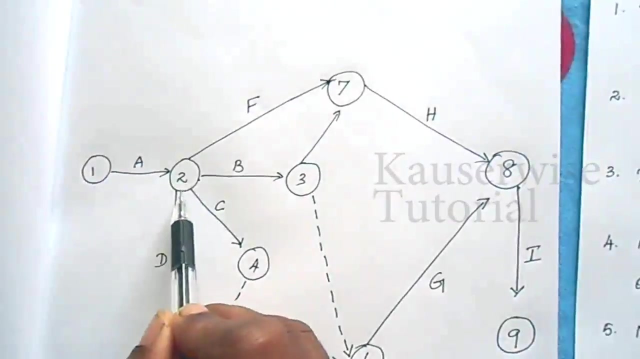 Tail event means the starting event is called tail event. The network should have a unique completion node That is head event. See for activity A. this is a tail event. This one is head event. For each and every activities it has tail event and head event. 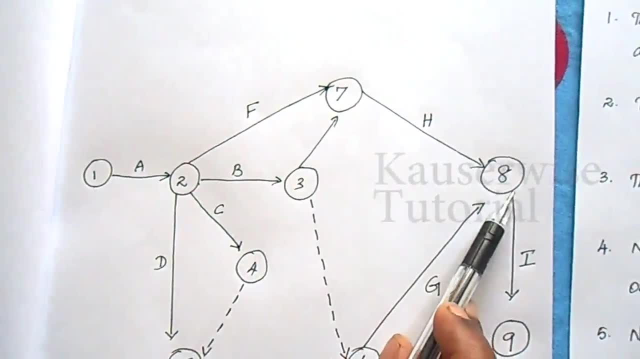 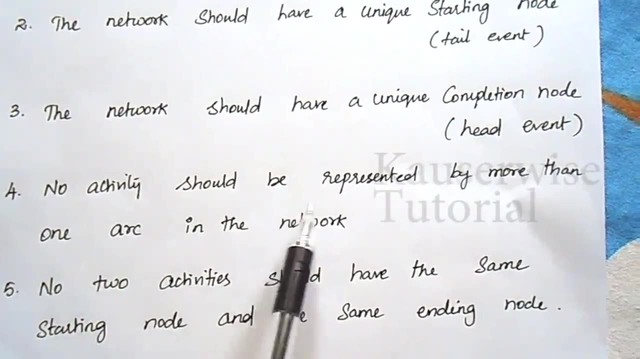 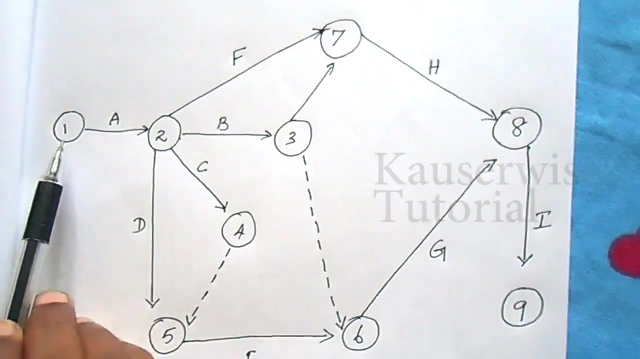 Tail event and head event. Tail event and head event. The starting node is called tail, The ending node is called head, Next one: no activity should be represented by more than one arc. Arc means activity in the network. See for each activity. it has two nodes. 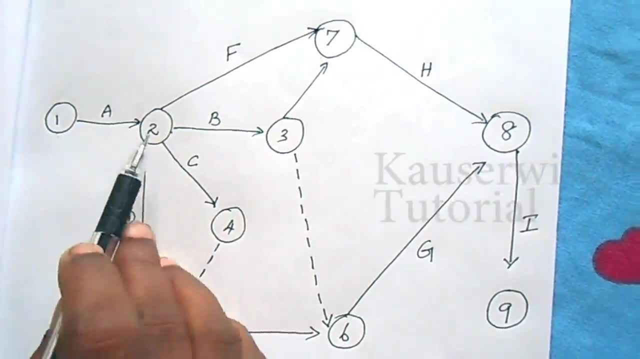 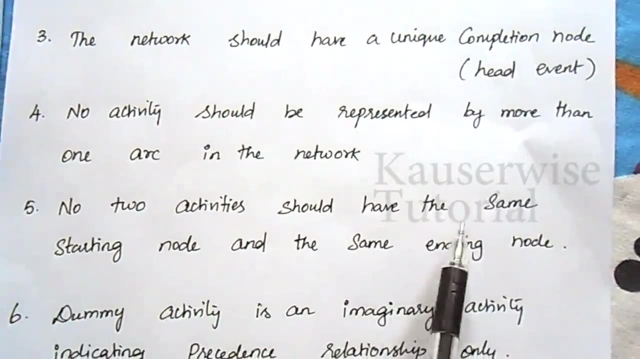 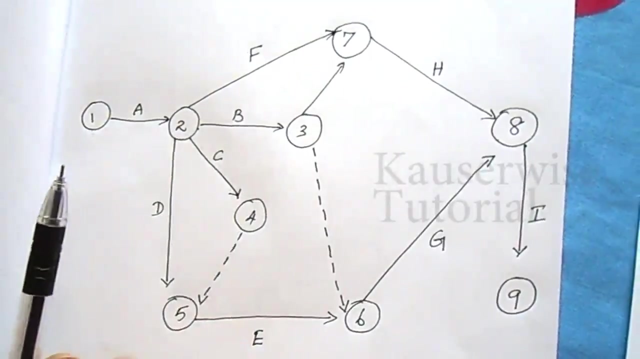 There will be no activity should be represented by more than one activity. So for each thing we will have only one activity, Next one. no two activities should have the same starting node, The same ending node. Look at the network. There will be no two activities which start in the same node and which ends in the same node. 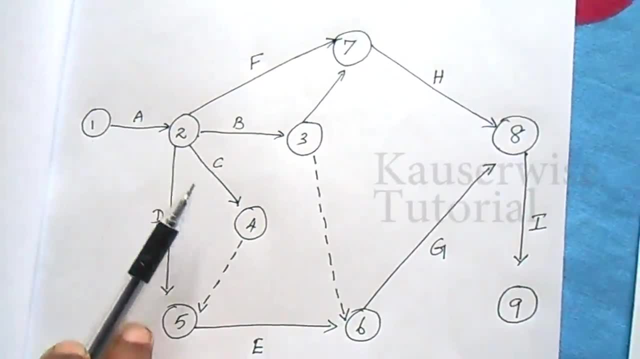 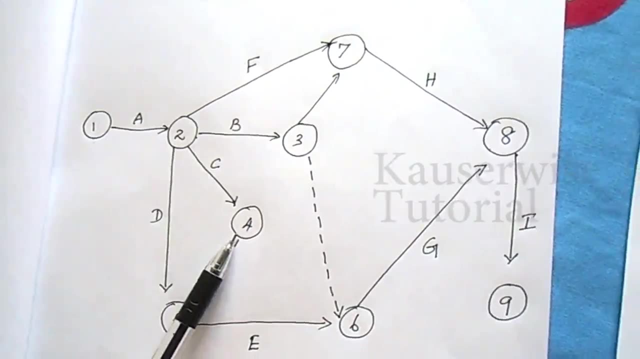 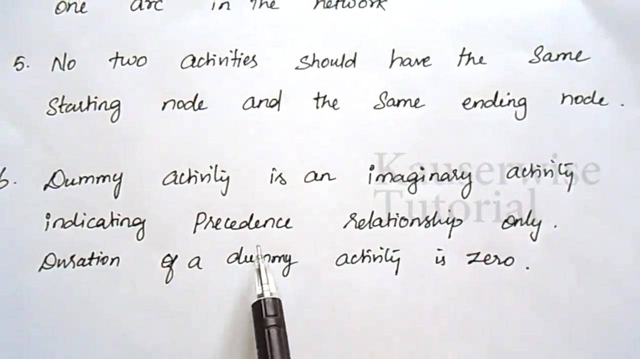 For each and every activity there will be a unique starting point and unique end point. So there will be no two activity which start in the same place, which ends in the same place In the last one. dummy activity is an imaginary activity indicating precedence relationship only. 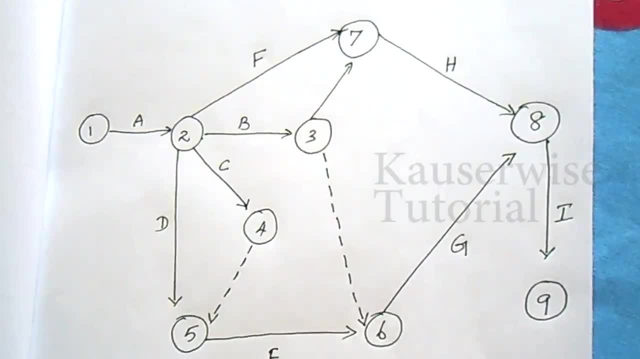 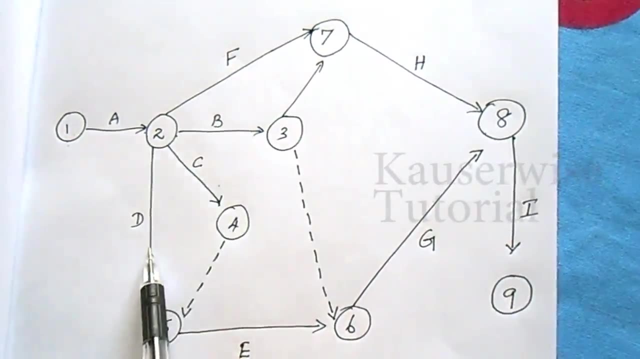 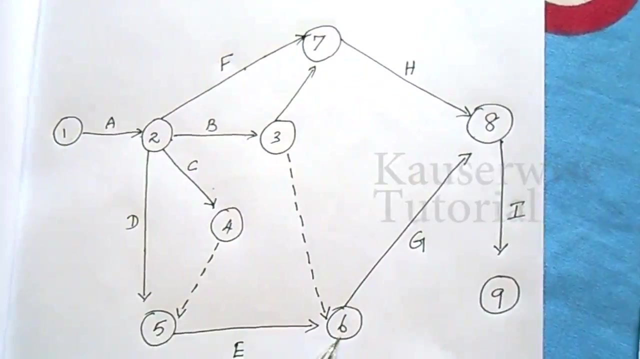 So duration? So duration of a dummy activity is zero. Look at the network: After completing activity A, then only we will move on to B, C, D and F. Okay, in the same way, after completing 4,, 5, then only we will move on to 6.. 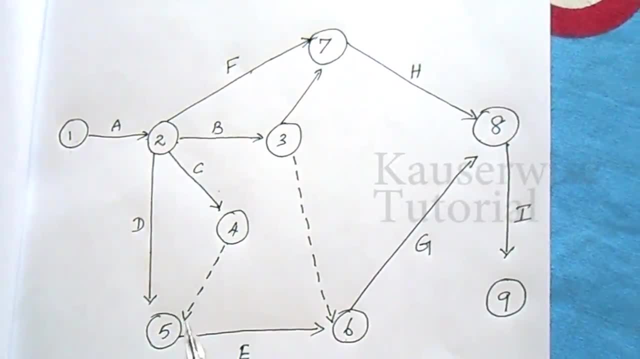 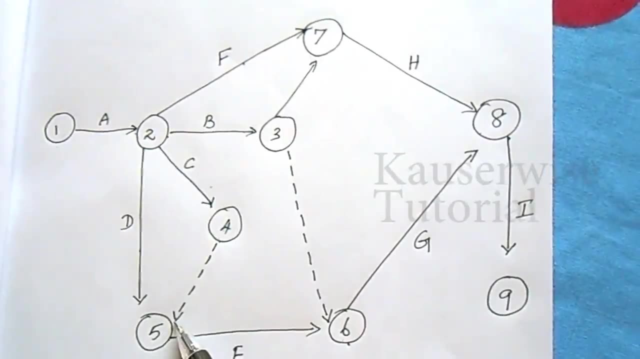 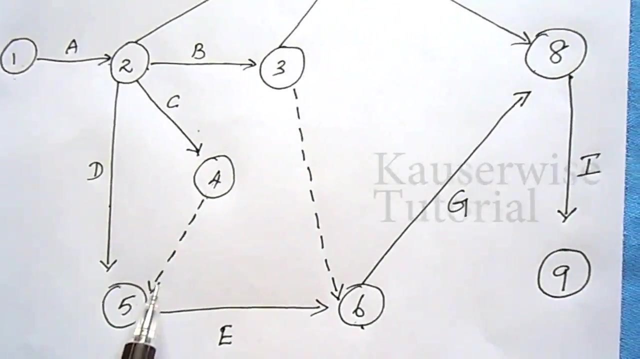 So here we have a precedence relationship that is 4,. 5 is a precedence relationship for the 6th activity. So we have a dummy activity. So for dummy activity, Dummy imaginary activity, there will be no duration for this. See, this imaginary activity indicates precedence relationship only. 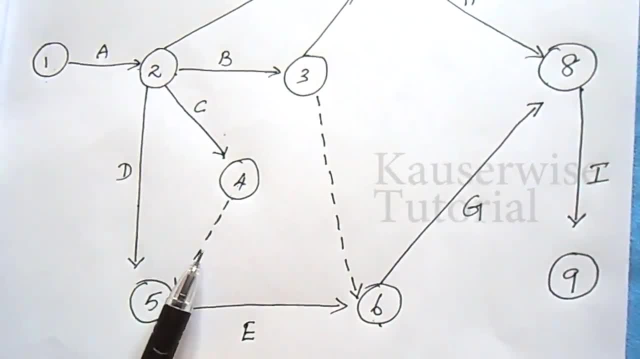 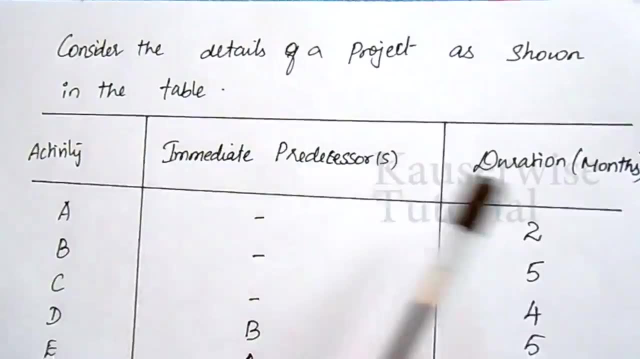 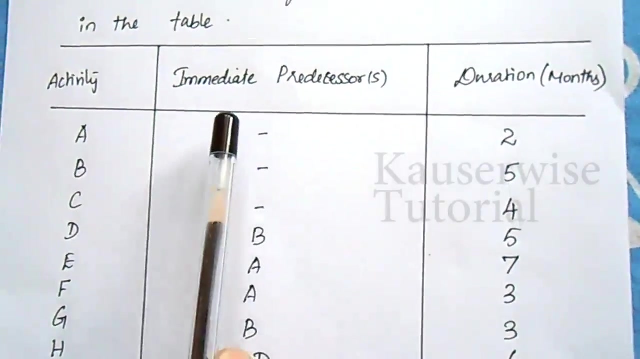 So there will be no duration for this dummy activity. The duration is zero only Let us see the problem. Consider the details of a project as shown in the table. Some information is given regarding the project, So these are the different activities. These are the informations regarding immediate predecessors. 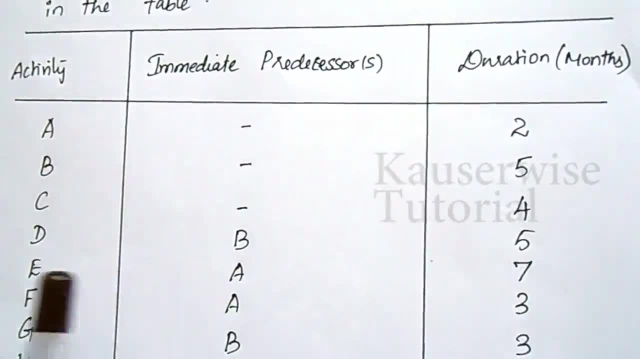 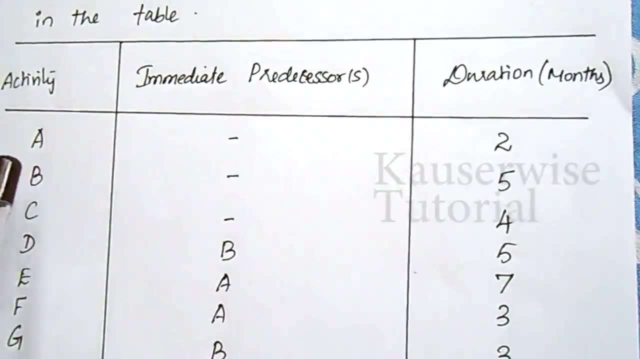 That is, after completing this activity Only you can able to start this activity. and after completing this you can able to start this activity. And this one is duration For each activity. these are the duration. So these are the three. informations are given. 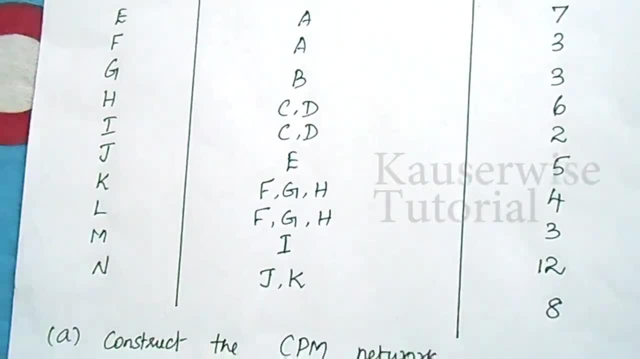 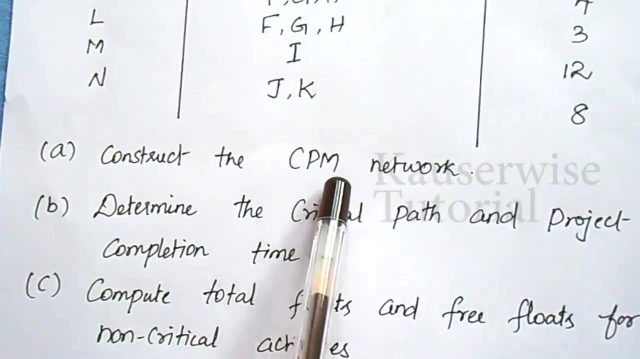 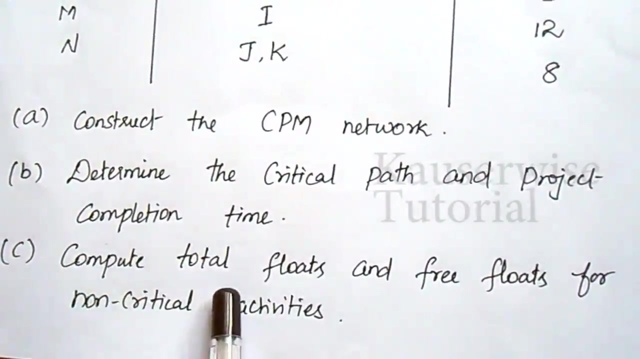 Activity, immediate predecessors and durations. Now, with this information, they ask you to construct the CPM network. CPM means critical path method And second one determine the critical path and project completion time. And the last one isло compute total floats and free floats for non-critical activity. So these are the questions. 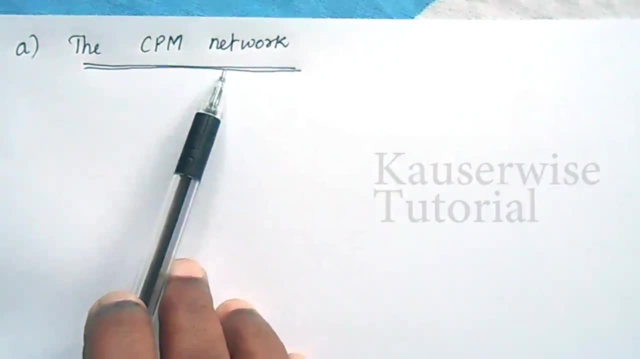 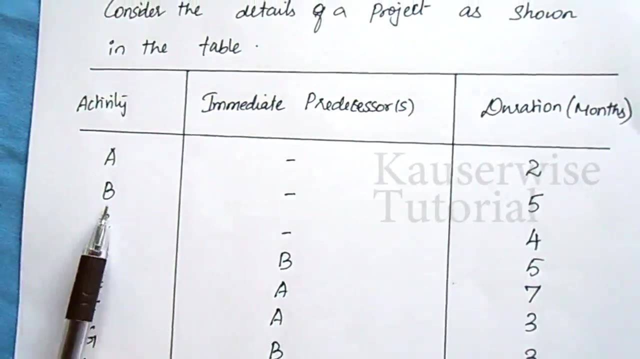 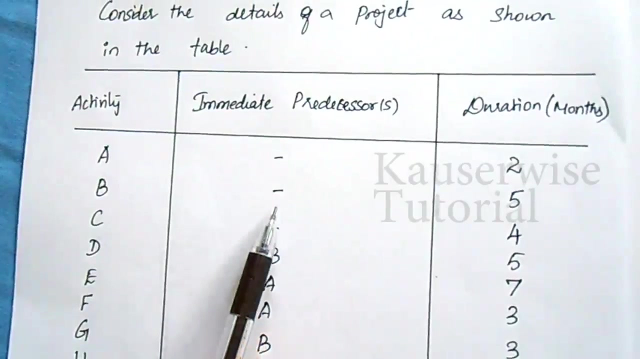 they have asked from these informations. First let us see how to construct the CPM network. Look at the problem. See the first activity for A, B, C. So these are the three activities without any immediate predecessors. So there will be no predecessors. Directly you can start. 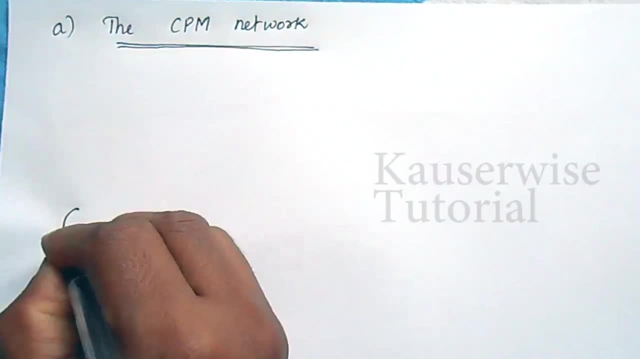 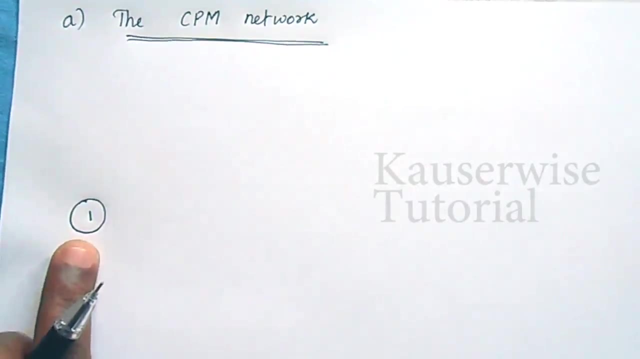 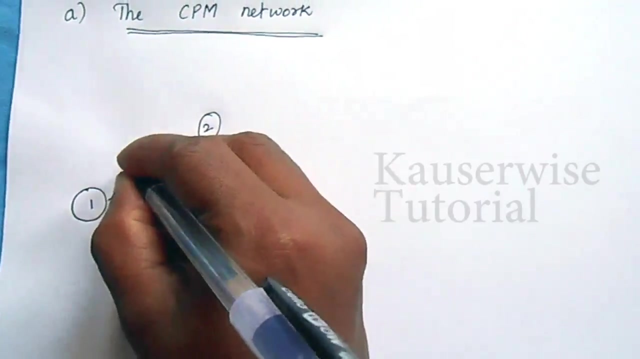 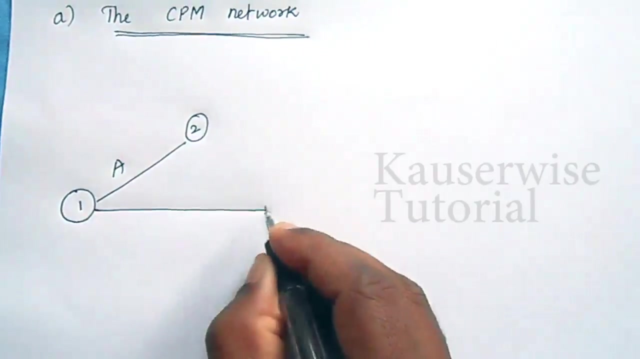 three activities: A, B and C. Node 1. For each activity we need to have two nodes, Okay, so first activity is A, without any predecessors for activity A, and then activity B, also no predecessors, So directly you can start from here. Activity B: 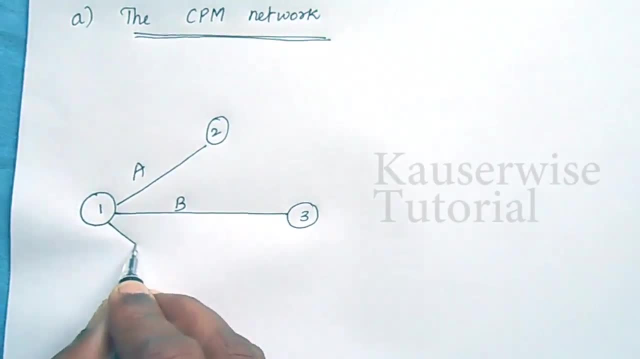 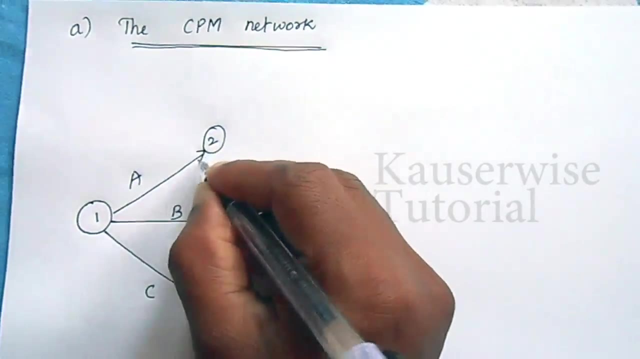 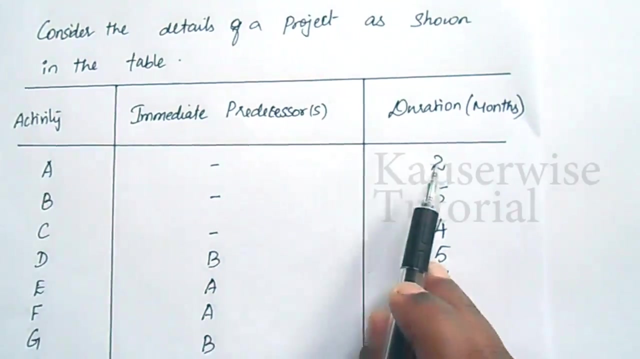 Then activity B, Then activity B, Then activity C, also no predecessors, So directly you can start activity C. So activity A, activity B, activity C. Now write the duration for each activity: For A two months, For B five months, For C four months. 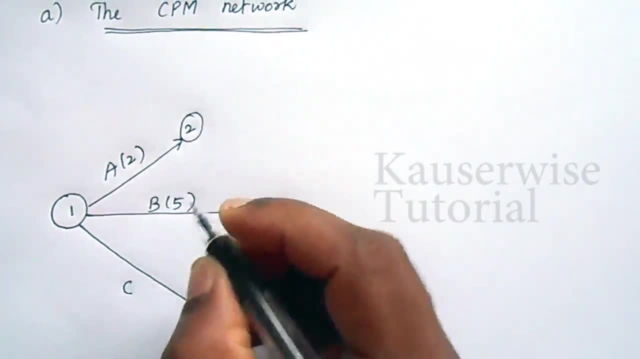 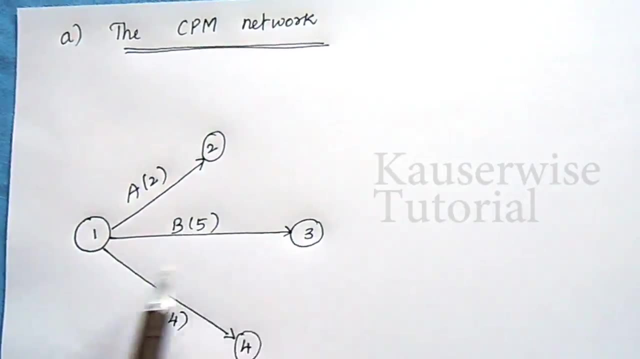 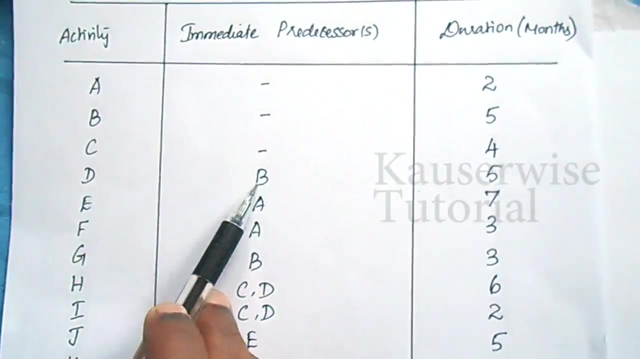 A two months, B- five months, C- four months. We have started three activities: A, B, C, B, C, A B C. Next one, that is D. Okay, but here predecessor information is given, that is, B is immediate predecessor for D, which means: 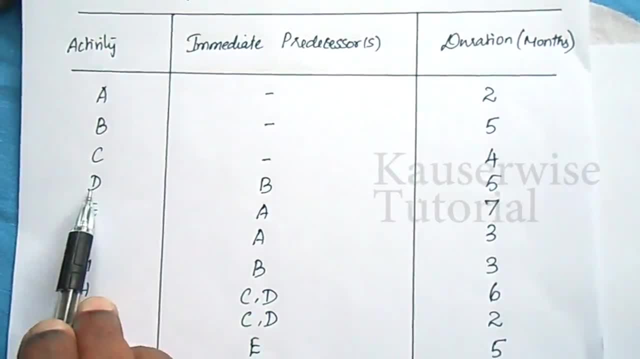 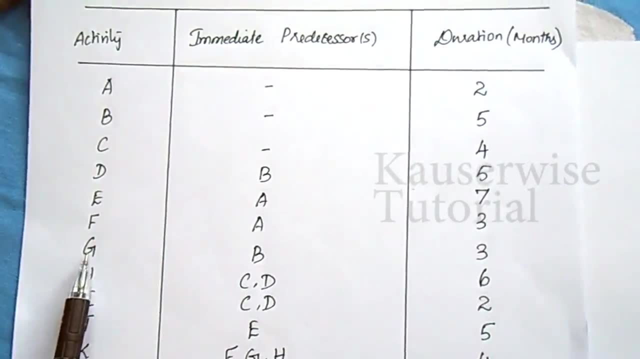 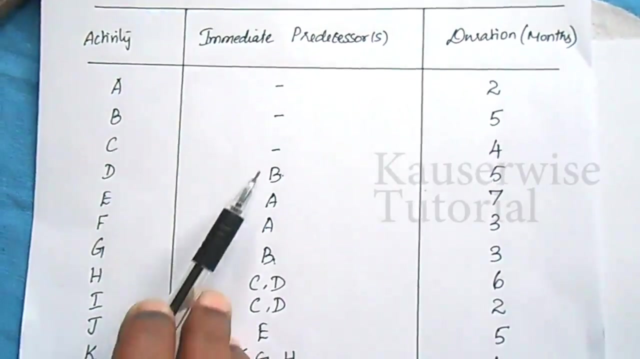 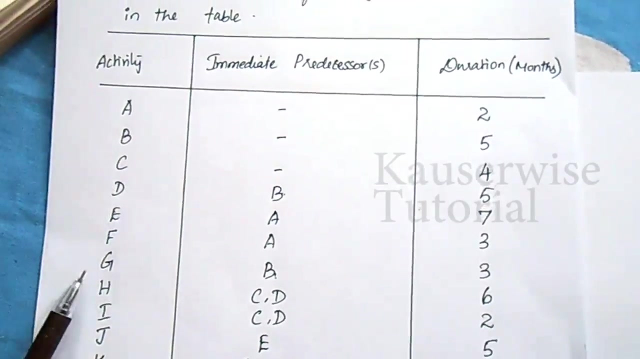 after completing B only you can able to start D. Okay, in the same way, one more B also is there. So B is immediate predecessor for G also. So which means, after completing B, you can start D as well as G. B is immediate predecessor for two activities, that is, D and G. These are the two activities which can start after completing B. 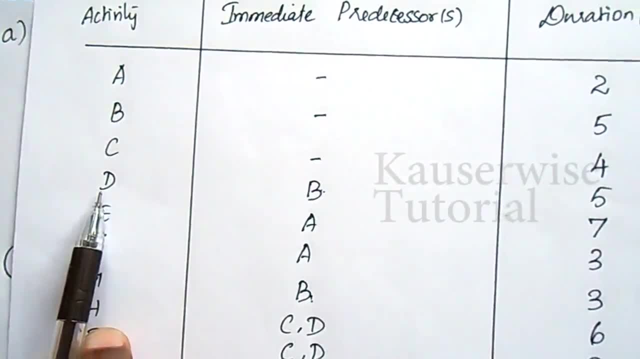 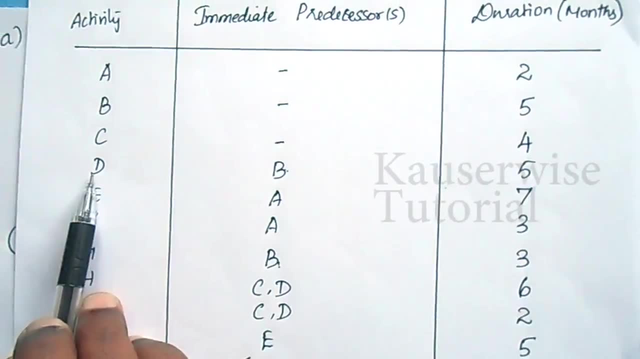 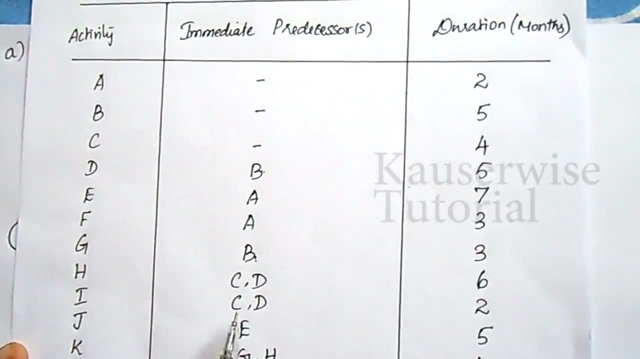 Before you draw activity D, just check whether D ends individually or it ends with any other activity. For that you have to verify immediate predecessors. Look at this activity here: C, D. It's immediate predecessor for H and C- D is immediate predecessor for I, which means 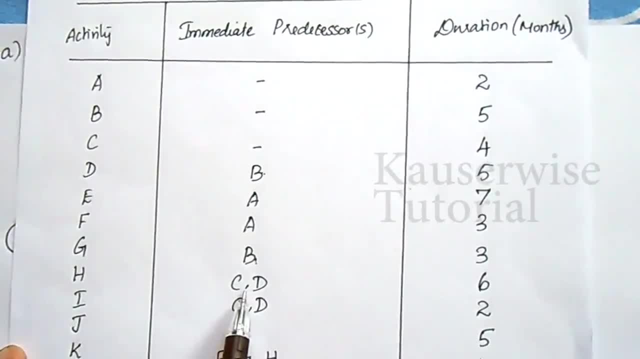 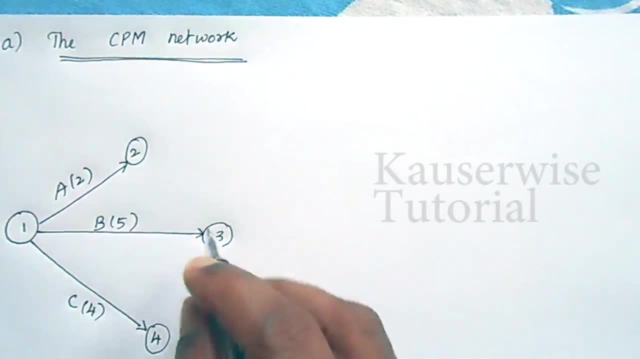 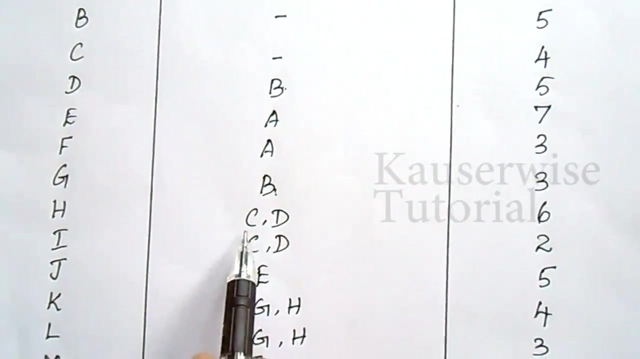 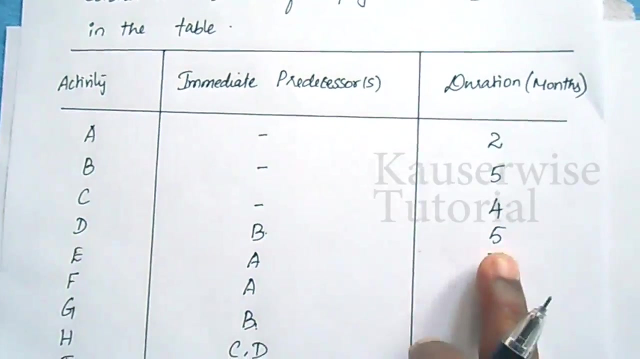 C and D. both the activities ends in a same place. So now you have to start from B and ends with C. B ends here. No, So now you have to start D. D starts from here and ends with C, C and D. both the activities are ends in a same place. D Duration: Look at the duration Five. 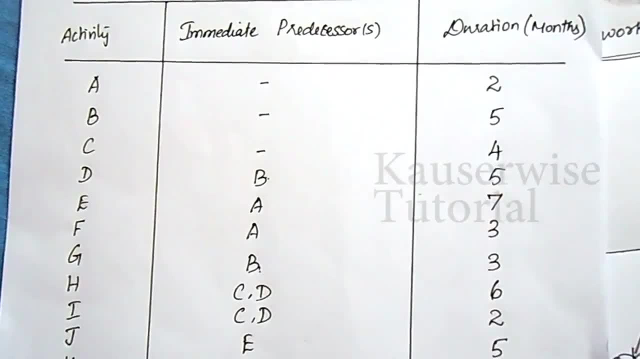 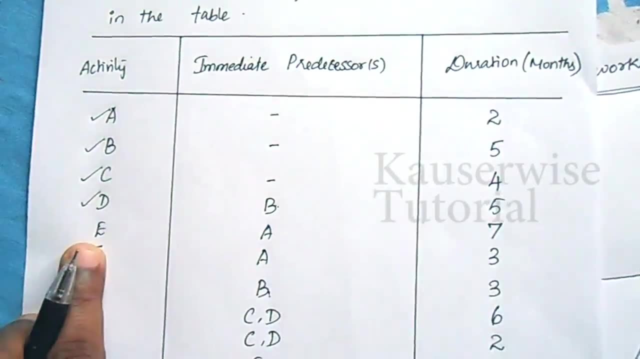 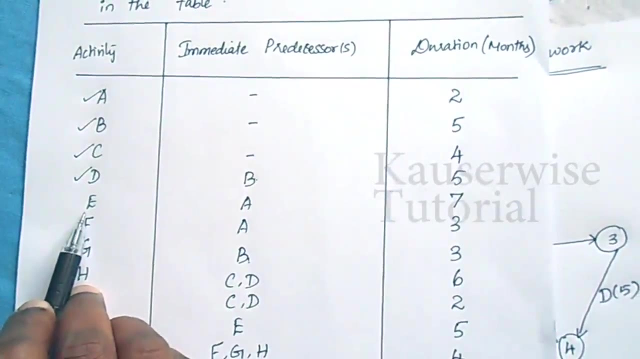 months. So far we have done network for activities A, B, C and D. Now you have to draw E. So before you draw the network, just see whether the particular activity is immediate predecessor for any other activity So that you can draw a network. 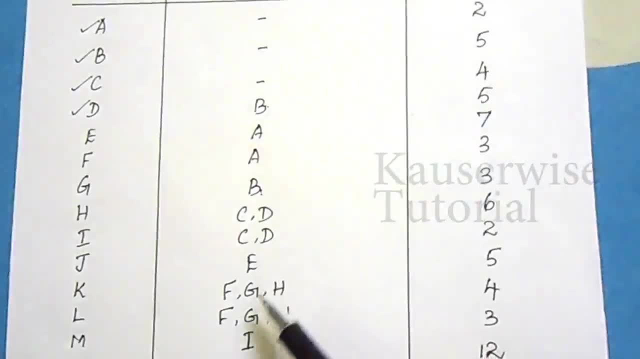 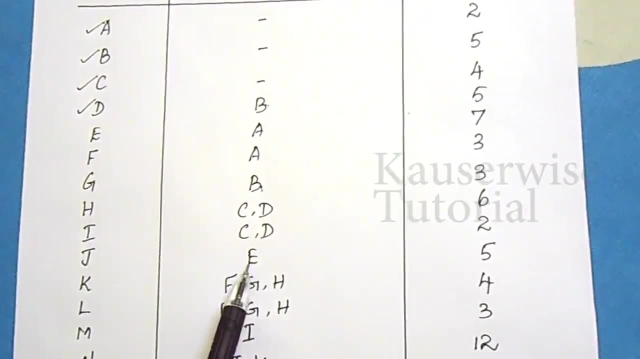 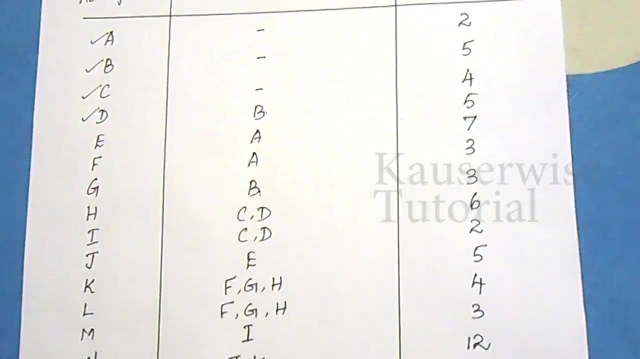 individually or you can find the exact direction. Yes, E is there, So E is immediate predecessor for G, But it is an independent activity, It ends separately. Okay, So now you can start E, But where E starts, Where A ends, So A ends here. Here you can start E. 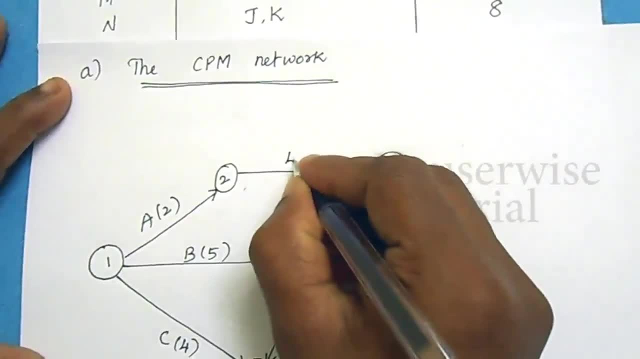 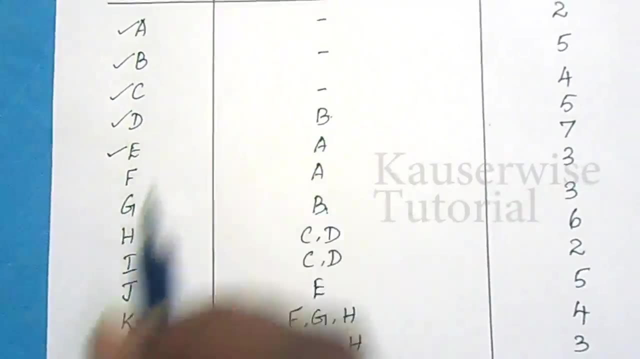 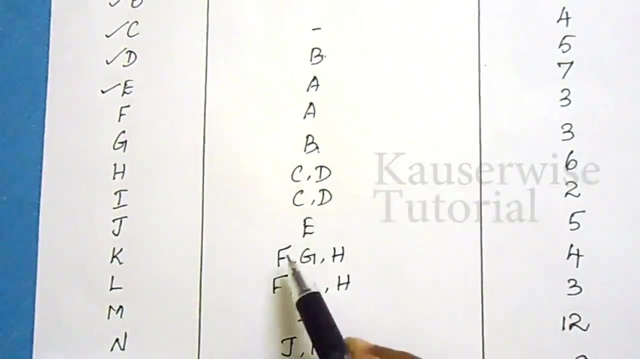 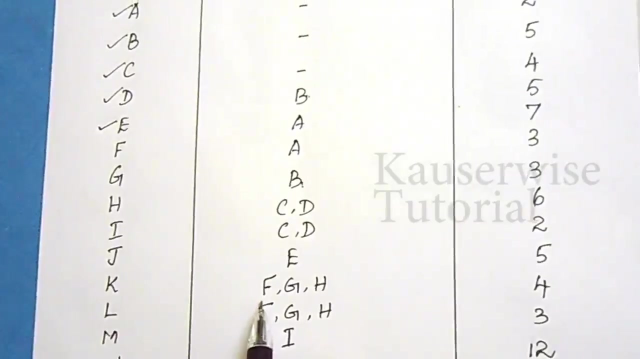 Node number five: E. Duration: seven months. E is over. Then move on to next activity, F. Just check: F is immediate predecessor for any other activity. Yes, So F is immediate predecessor for K as well as for L. F is not an independent activity. Why? 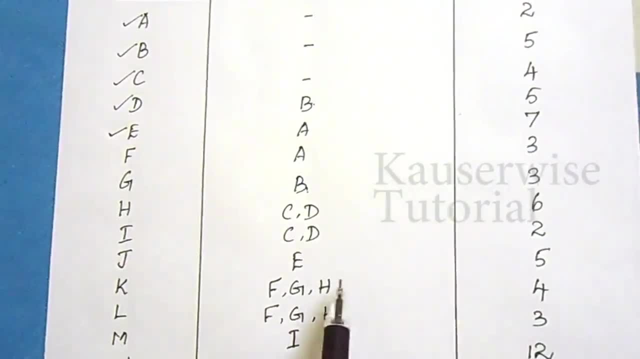 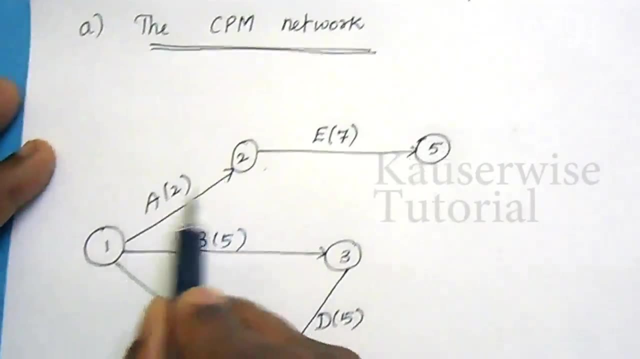 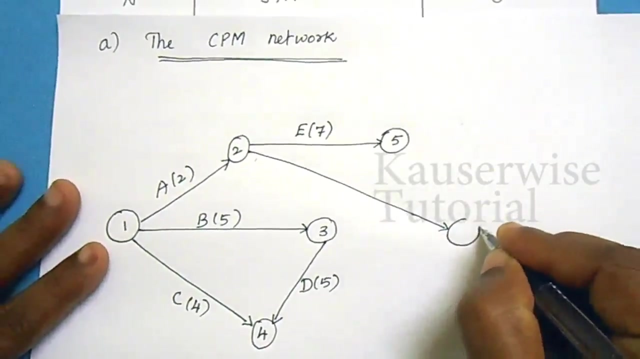 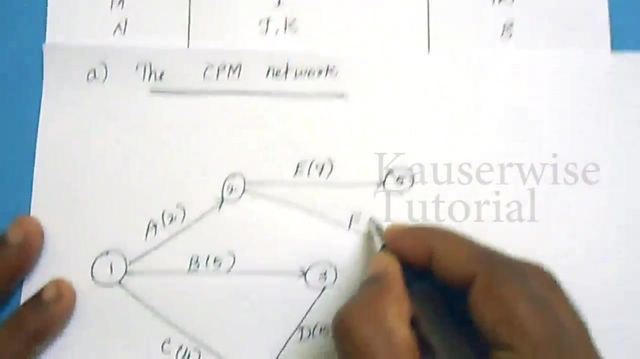 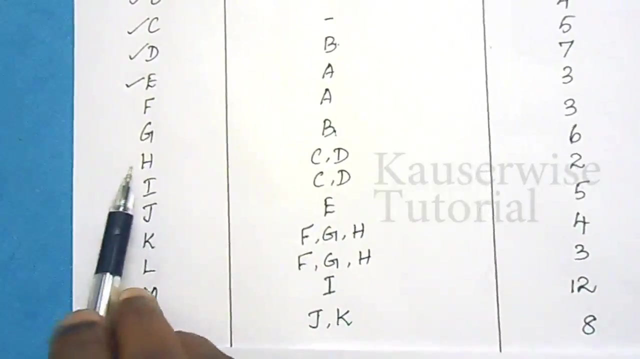 Because it ends with some other activities In single node. F, G and H ends in single node, But F starts where A ends. A ends here, It starts from here. F, Duration, Three At the same time, G. So G also ends in same node. H also ends in same node, But where it. 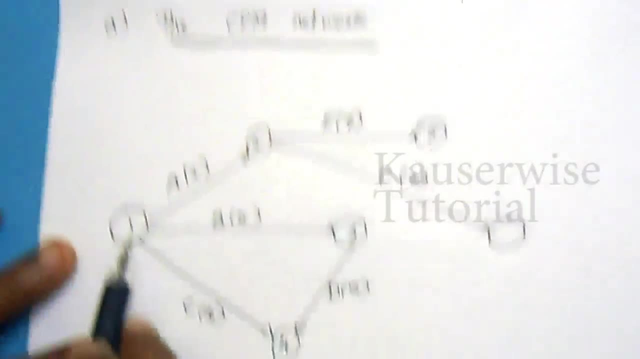 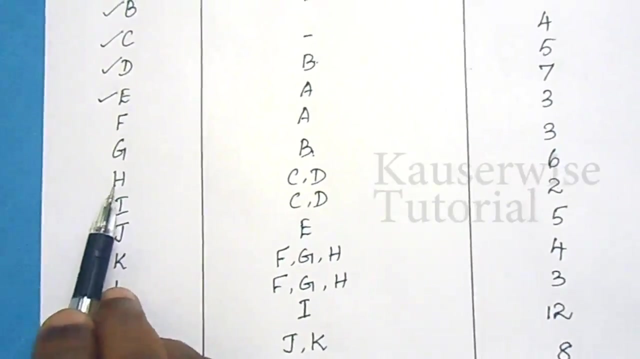 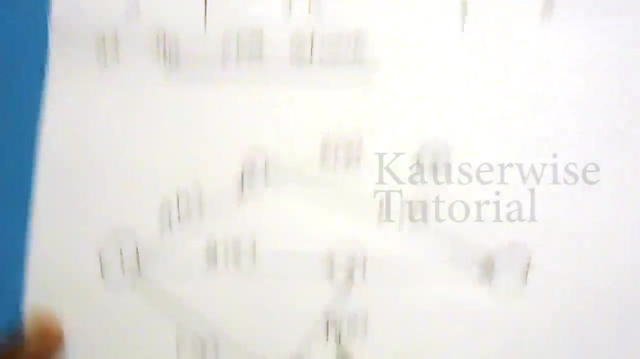 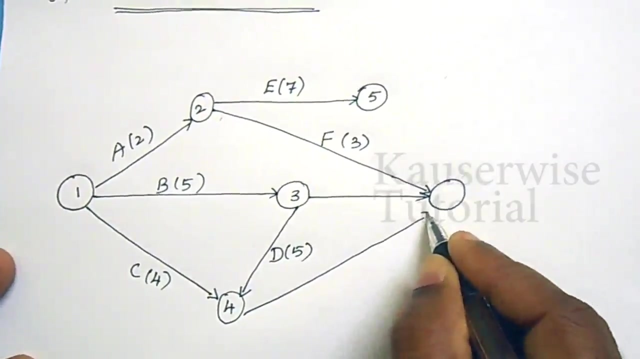 starts. G starts where B ends. B ends here, So it starts from here and ends with same node. And look at the next activity, H. So H also ends in same node, But it starts where C and D ends. C, D ends here, So it starts from here and ends in same node. So this one is G And this one is H. 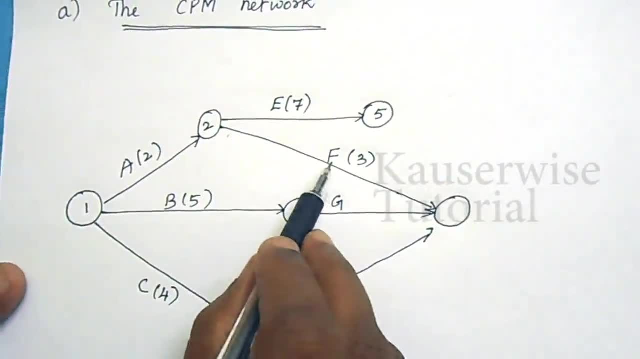 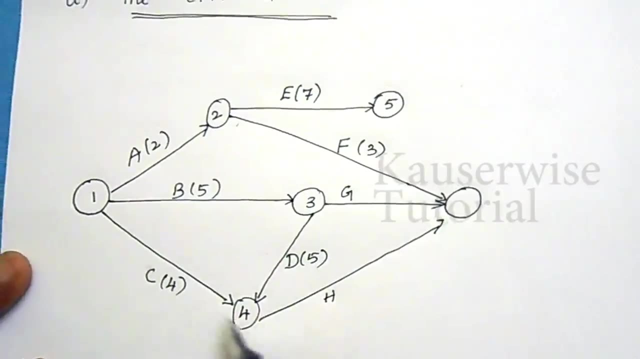 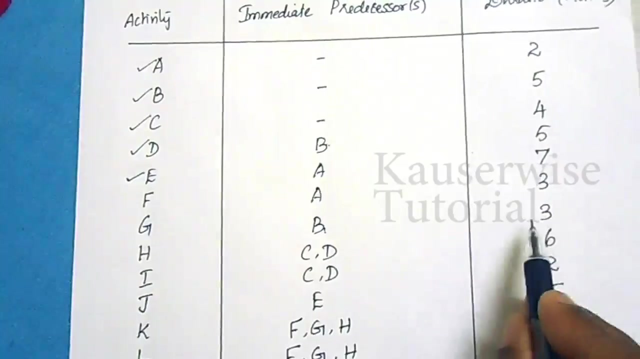 So these are the three activities. This activity starts where A ends, This activity starts where B ends And this activity starts where C, D ends. These are the three activities ends in same node. Now write the duration for G, For H: six months. 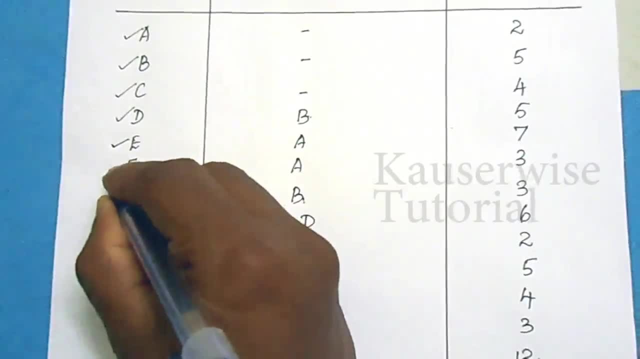 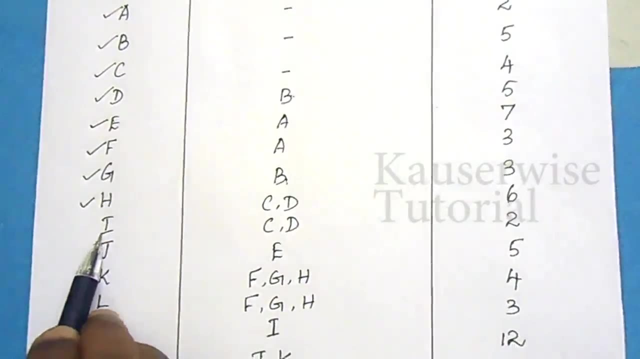 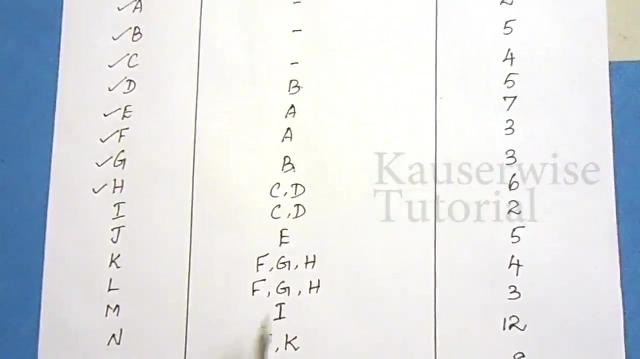 Node number six. So we have done F, G and H. Now move on to the next activity I. So just check whether I is an immediate producer for any other activity. Yes, I is an immediate producer for activity M, But it is an independent activity. It starts alone. 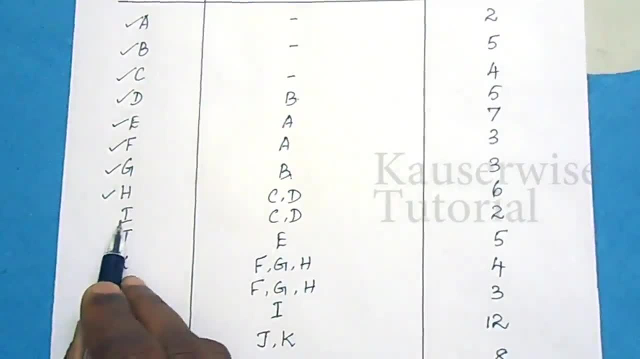 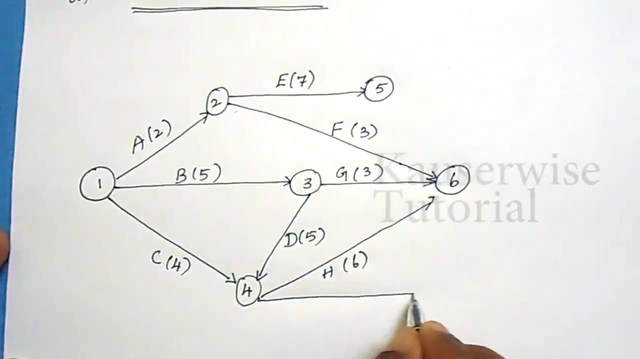 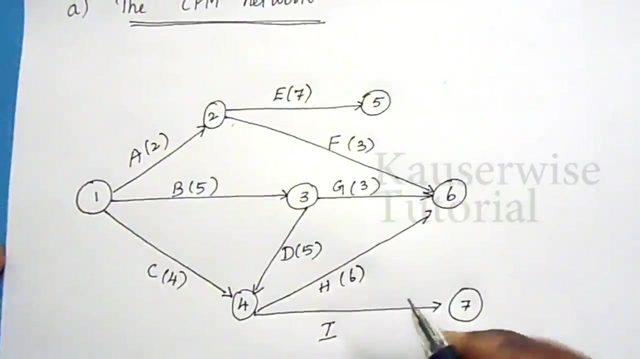 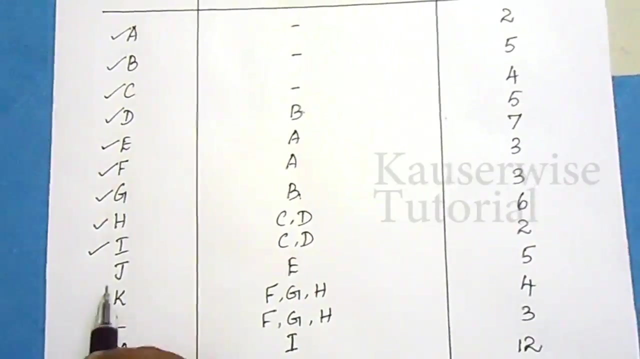 But where I starts, Where C D ends, I starts. So C D ends here And I starts from here. Node number seven: I Look at the duration: Two, Two months I is over. Then J Look at the immediate producer. 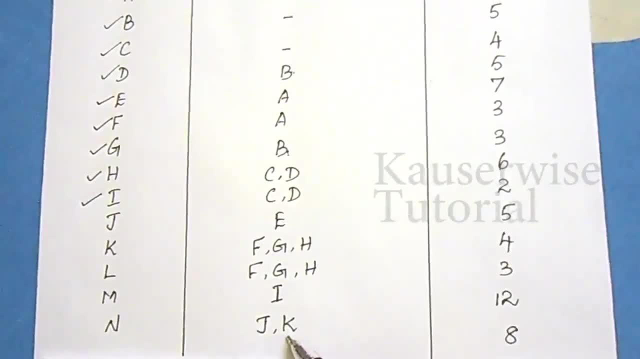 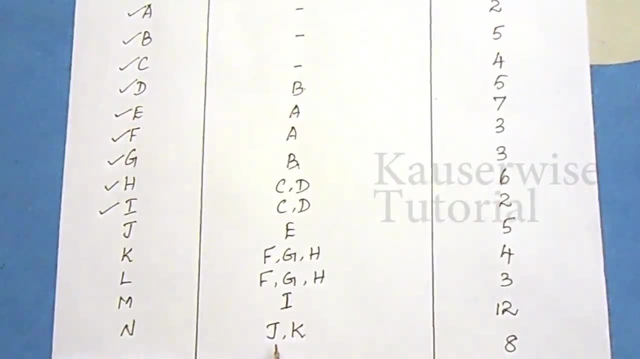 Yes, J is there, So J- K ends together, So J is an immediate producer. It is there for activity N. It is not an independent activity, It is a dependent activity. Why? Because it ends with some other activity, So J starts where E ends. 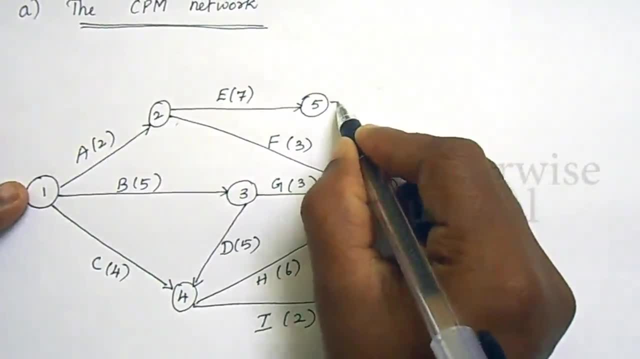 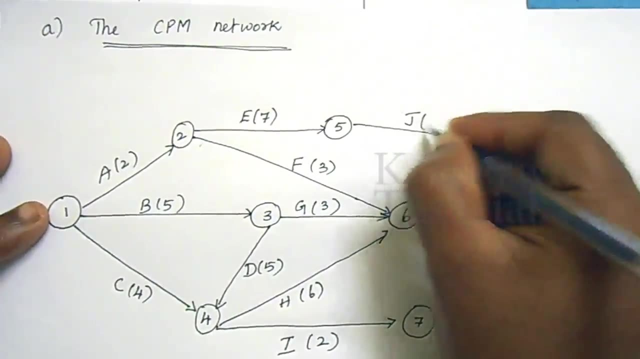 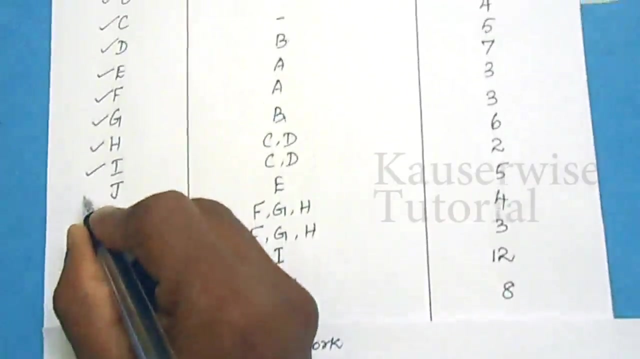 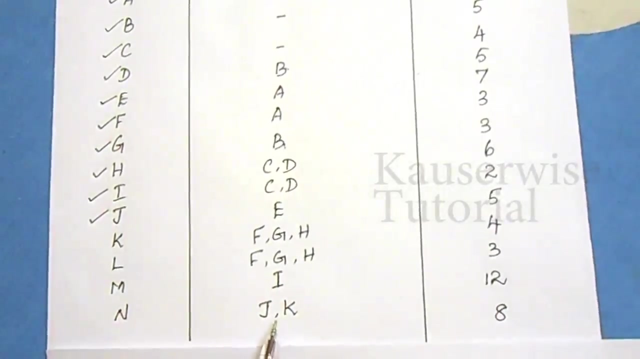 E ends here, So J starts from here. Duration: Five months Duration Over Then K, So K is an immediate producer for activity N, But it ends with J. So now only we have drawn J, No Node number. 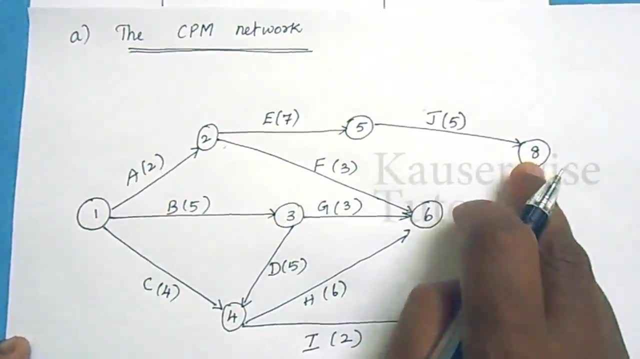 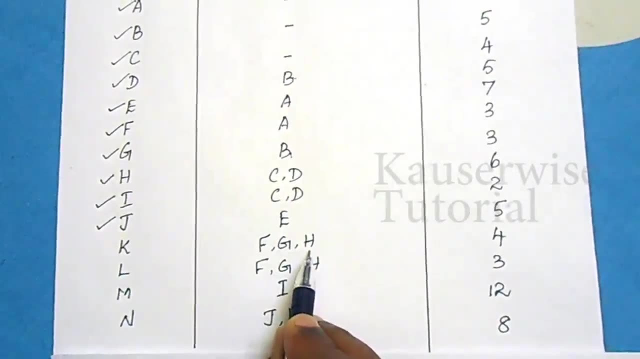 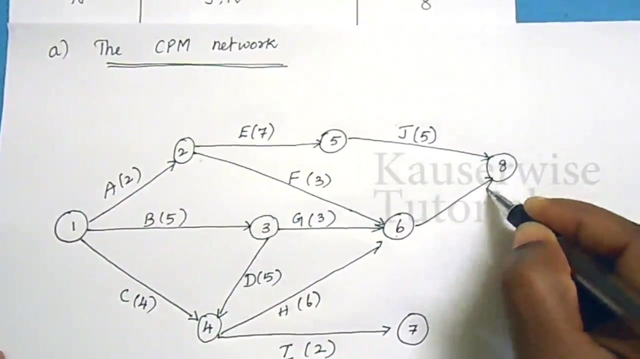 Node number eight. So J ends here. K also ends here, But K starts from where K starts, where F G H ends. F G H ends here. So K starts from here and ends with J. Duration For K Duration: Four months. 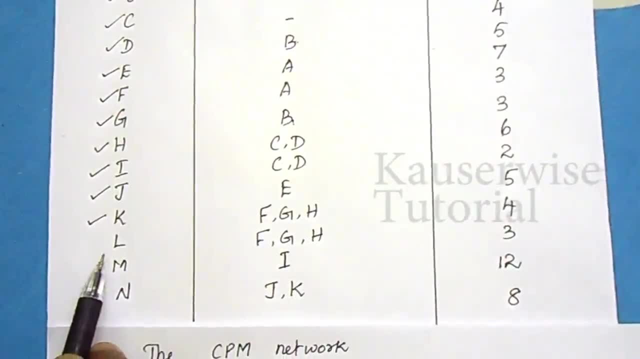 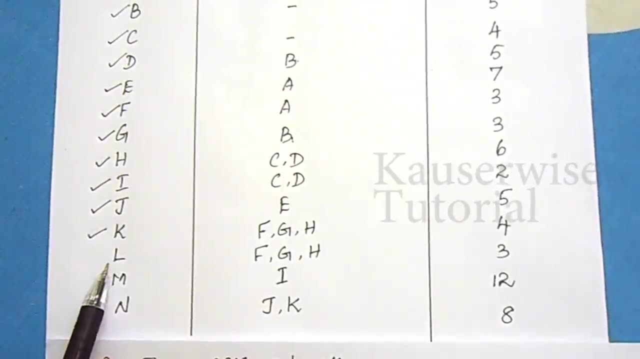 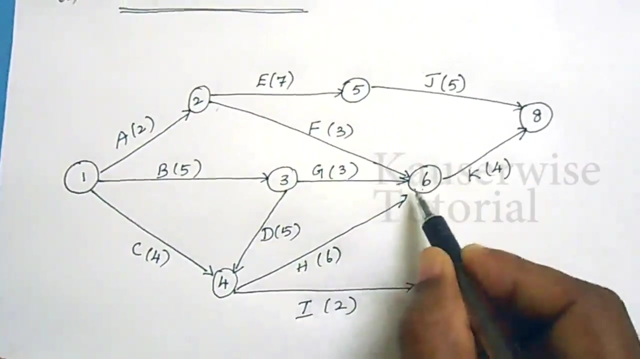 Now move on to next activity, L. Just check whether L is an immediate producer for any other activity. No, L is an independent activity, But it starts where F G H ends. F G H ends here. L starts from here. 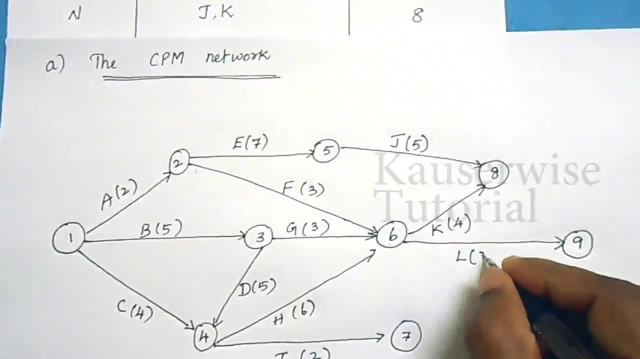 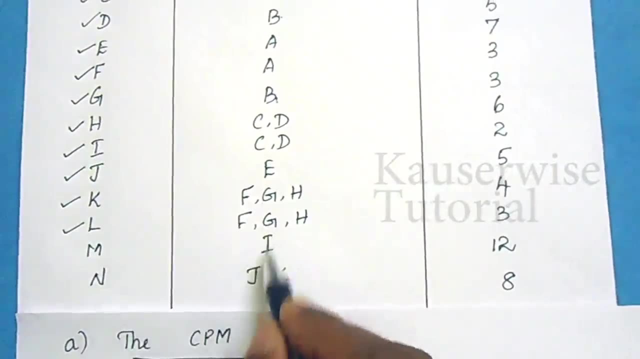 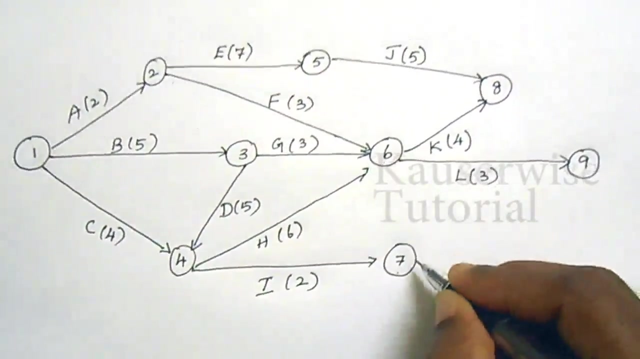 But ends individually. Node number nine Three. Next one, M, So M also independent activity. Why? Because it's not an immediate producer for any other activity. So it starts where I ends, So I ends here. It starts from here and ends in the last node. 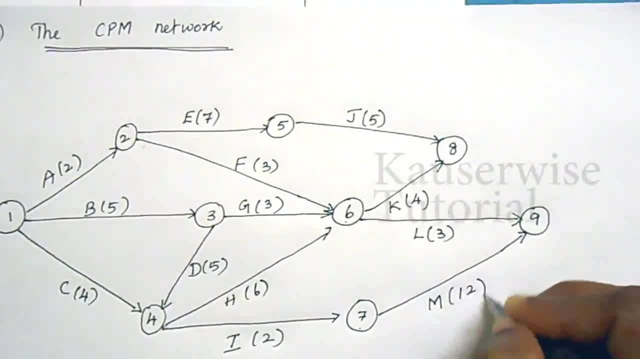 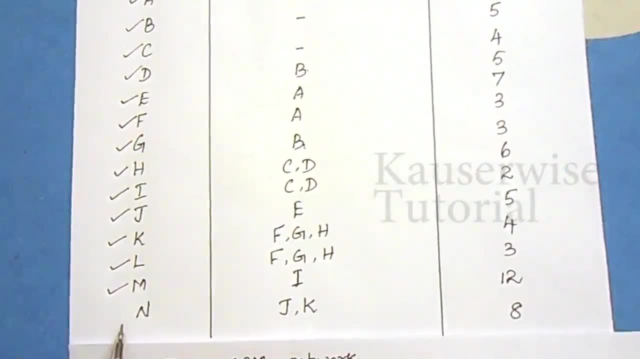 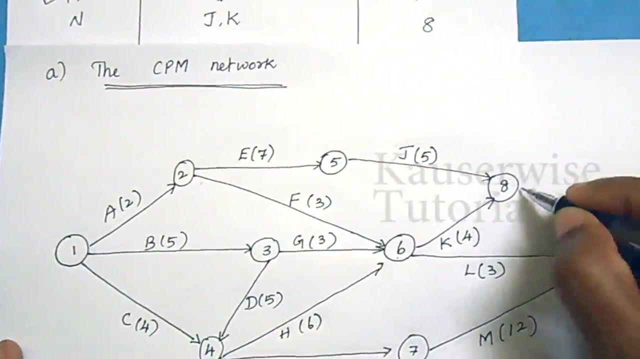 That is M Duration: Twelve months In the last one, N. So N also is not an immediate producer for any other activity. It is a last activity And it starts where J K ends. J K ends here. It starts from here and ends here. 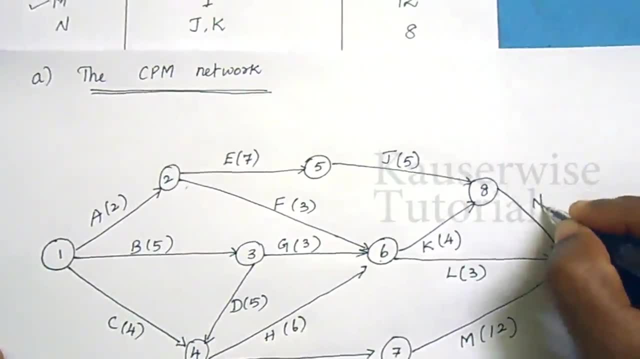 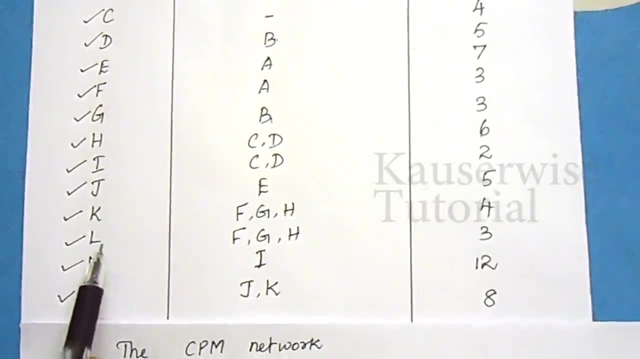 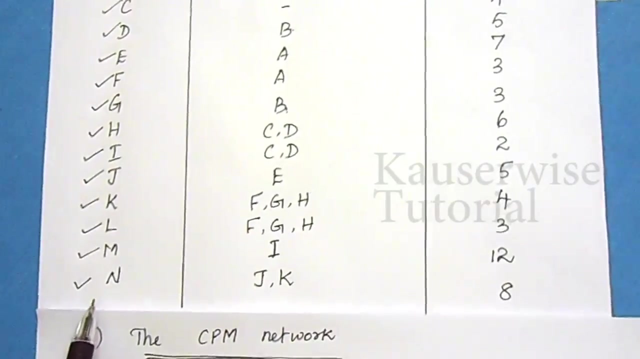 Nine is a last node. Duration: Eight, Eight months. Look at these three activities: L, M, N. So these are the activities which is not immediate producer for any other activities. So these are the activities called as ending activity. So three activities ends in same node. 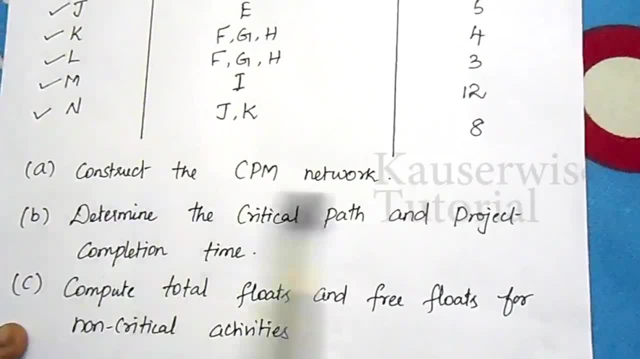 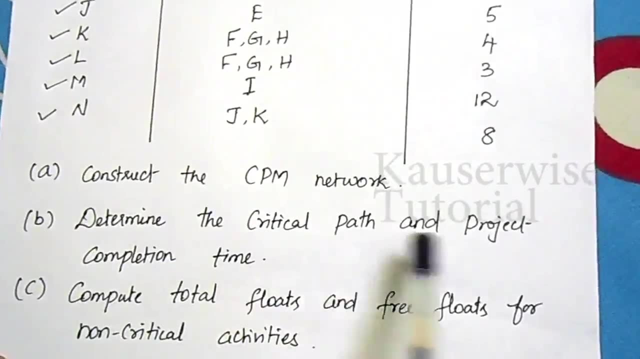 This is the procedure to draw CPM network First. one is over. That is, construct. the CPM network is over. Now move on to next calculation, That is, determine the critical path and project completion time. Now let me explain what is the meaning of critical path. 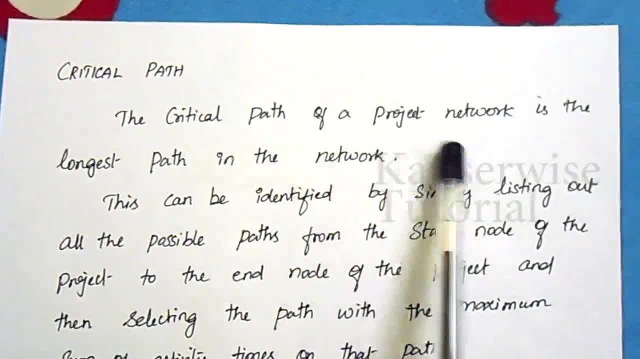 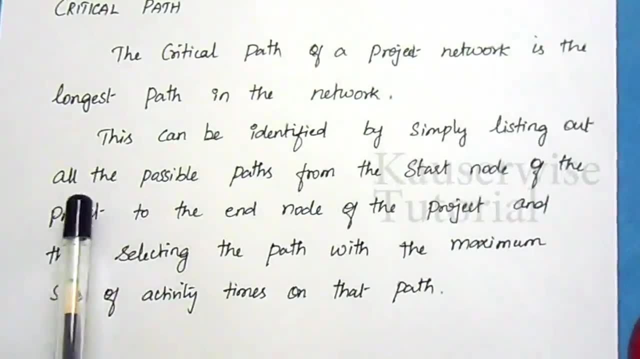 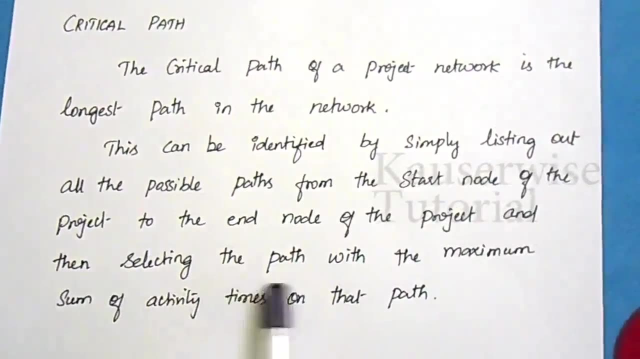 See. critical path means the critical path of the project network is the longest path in the network. So this can be identified by simply listing out all the possible paths from the starting node of the project to the ending node of the project And then selecting the path with a maximum sum of activities on that path. 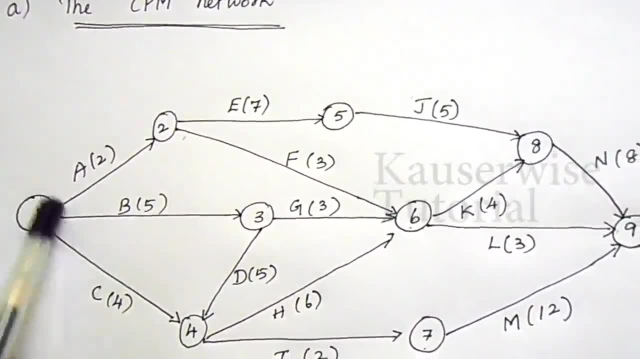 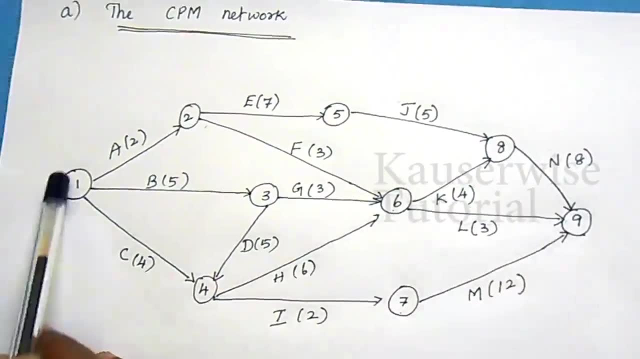 See. look at the network Here. node 1 is a starting node and 9th node is a ending node. Okay, So just find out the paths, which starts from 1 to 9. Node 1 to 3.. Then 3 to 6.. 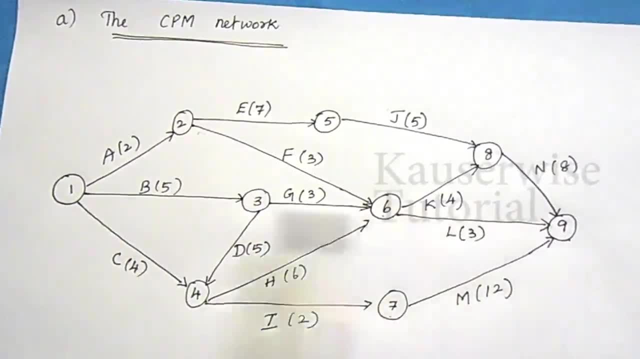 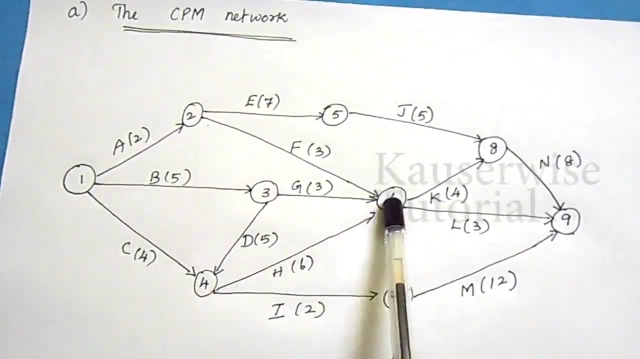 Then 6 to 9. Starts from 1 and ends with 9.. Okay, So this is one of the possible path, And look at the next one: From 1 to 4.. 4 to 6. And 6 to 9.. 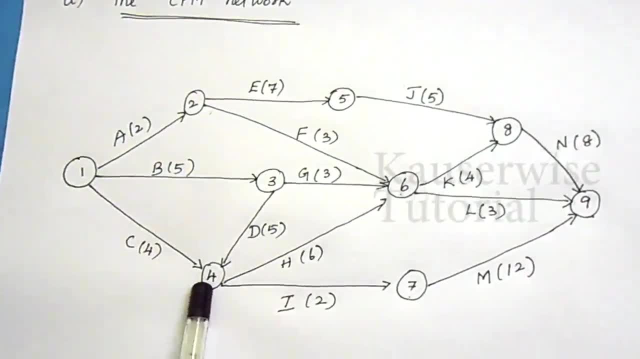 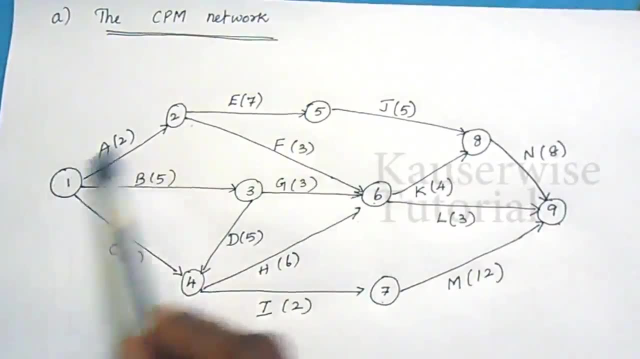 Also one of the possible path. And next one: 1 to 4.. 4 to 7. And 7 to 9.. Then 1 to 2.. 2 to 6.. 6 to 9.. Then 1 to 2.. 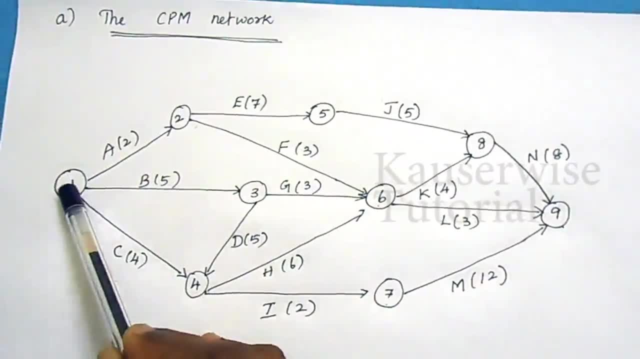 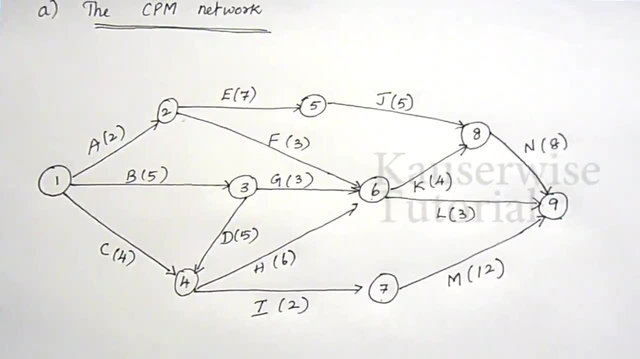 2 to 6.. 6 to 8. And then 9.. Then 1 to 2.. 2 to 5., 5 to 8. And 8 to 9.. These are the various possibilities, which starts from 1 to ends with 9.. 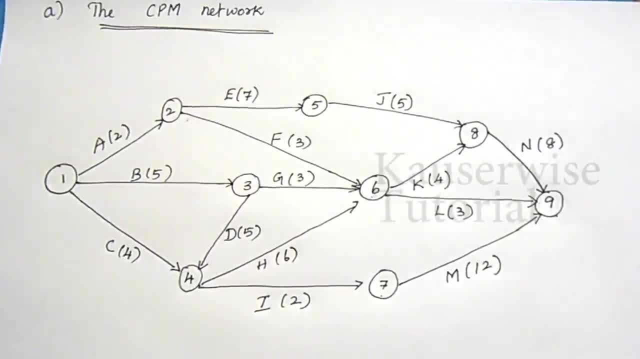 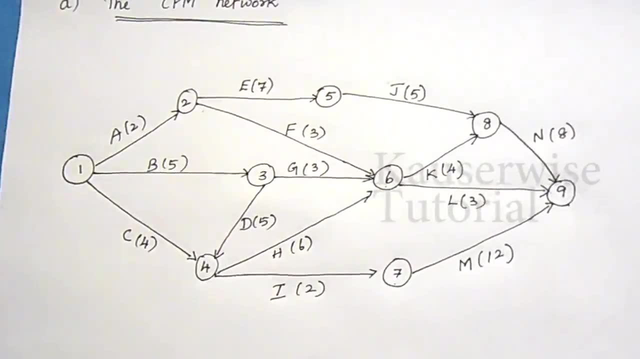 So now you have to find out which path is a maximum duration, So which path is a critical path. So, in order to find out the exact critical path, we have to follow certain rule. There are two phases in order to find out the critical path. 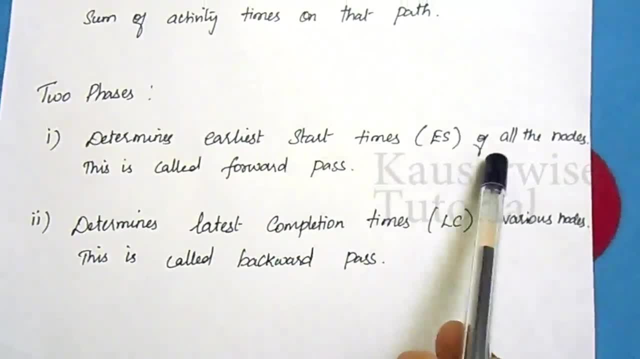 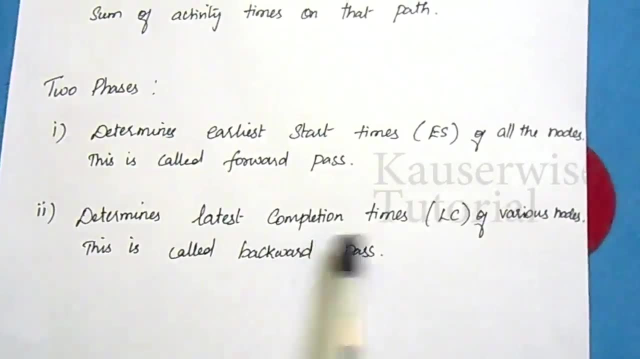 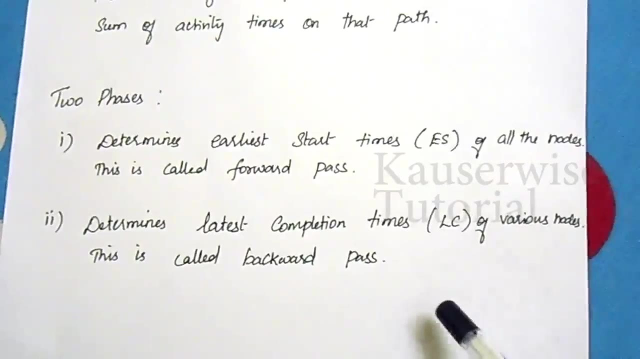 First one is determine earliest start time for all the nodes, So this is called as forward pass. And the next one is Determine latest completion time of all the nodes. This is called as backward pass. So these are the two phases. We need to find these two things in order to find out the critical path. 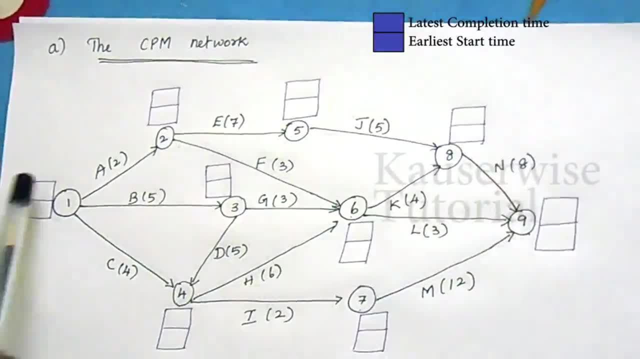 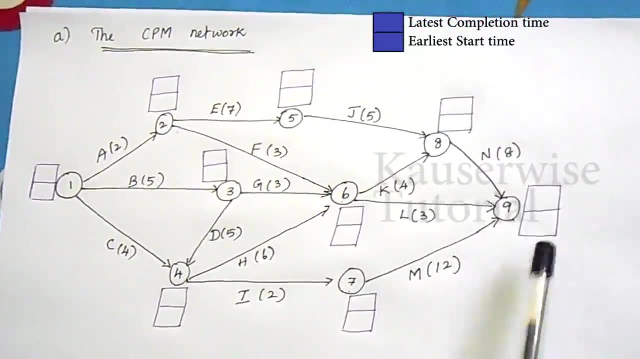 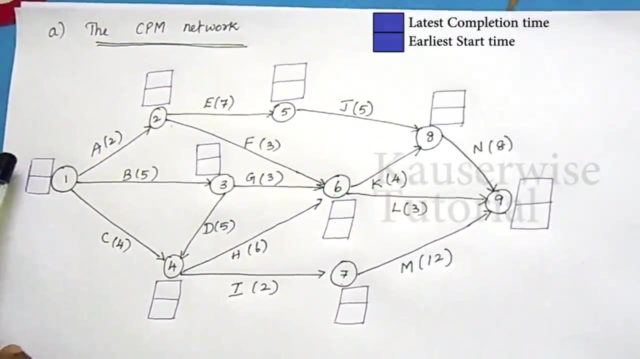 For each node we need to have two squares: Upper square, Lower square. Okay, So these two squares is very important for each and every nodes. The lower square stands for earliest start time And the upper square stands for Latest completion time. 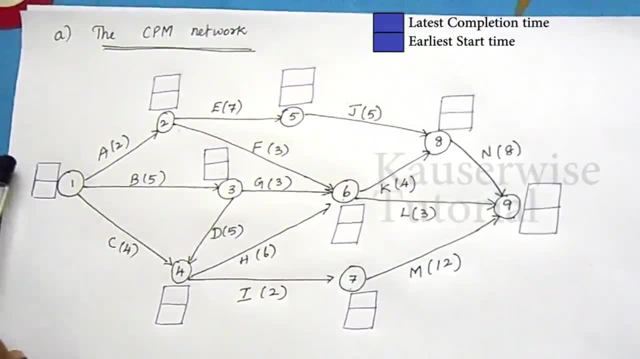 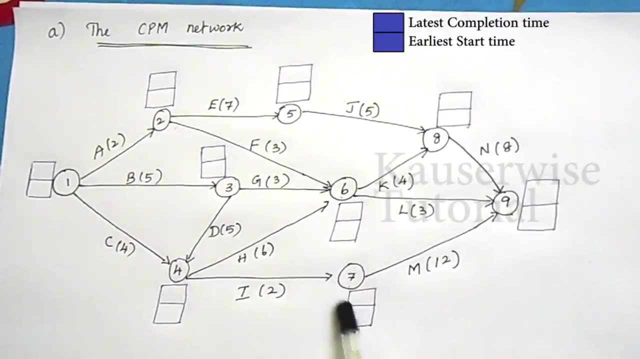 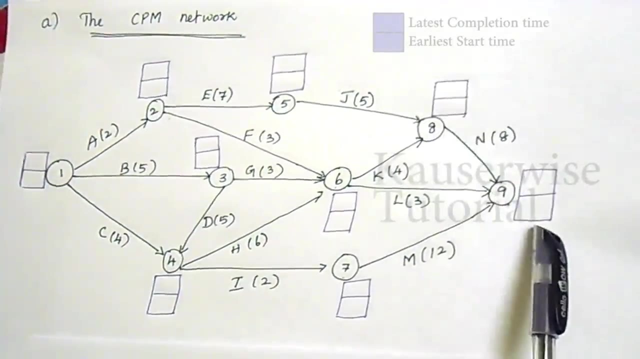 So you need to find earliest start time and latest completion time for each and every nodes. For that only I have drawn a blue color square, upper square and lower square. Now let us see how to calculate earliest start time for each and every node. 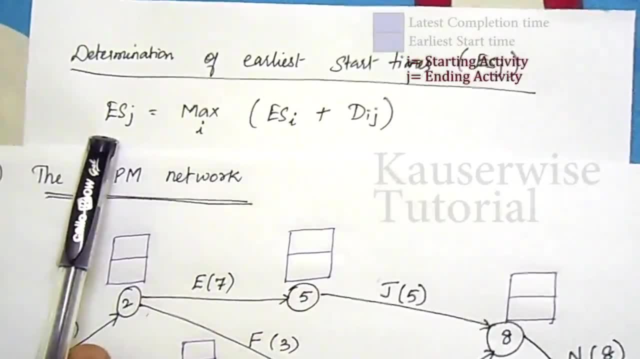 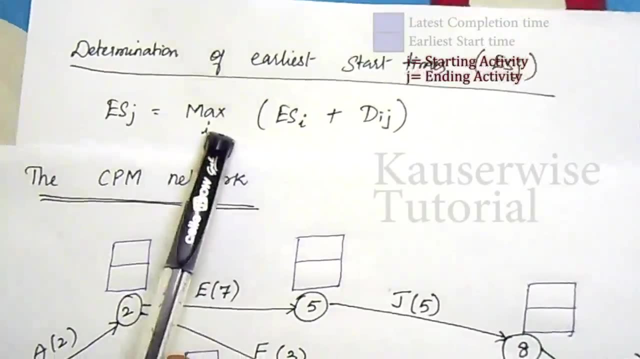 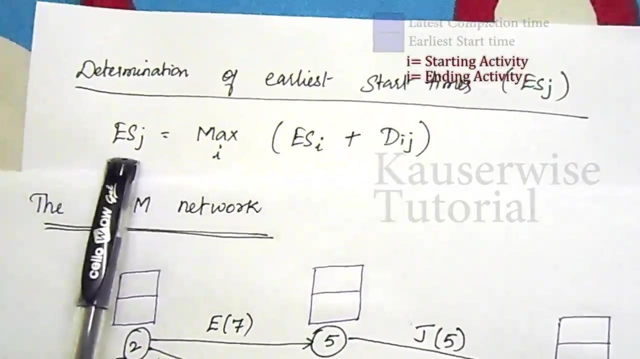 Look at the formula to determine earliest start time. So earliest start time of J- J stands for ending activity, I stands for starting activity. So maximum of earliest start time of ith activity plus duration, So you will be getting earliest start time of ending activity. 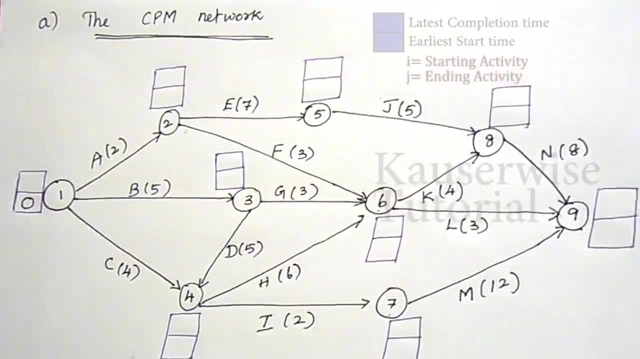 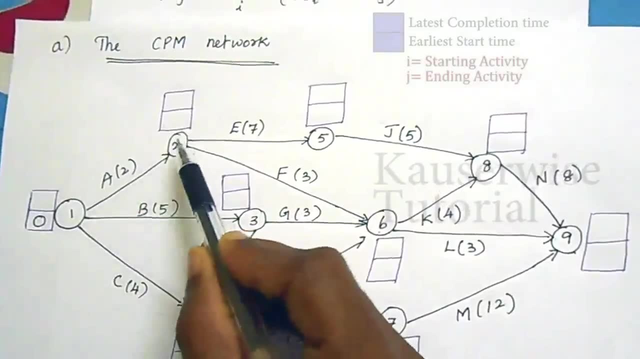 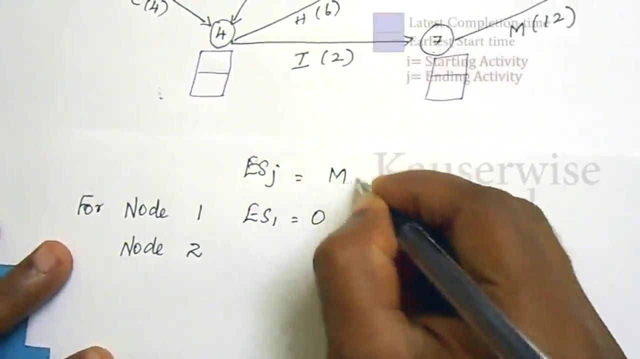 So now I'm going to show you how to apply this formula. Okay, So earliest start time of first node is always zero. Okay, Now you have to find out the earliest start time for node two. Okay, Look at the calculation. Early start time of J is equal to maximum of I. 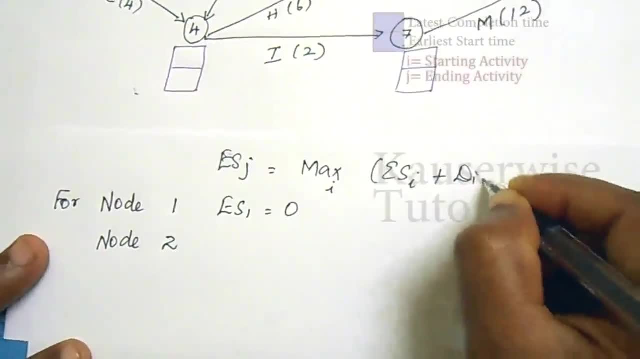 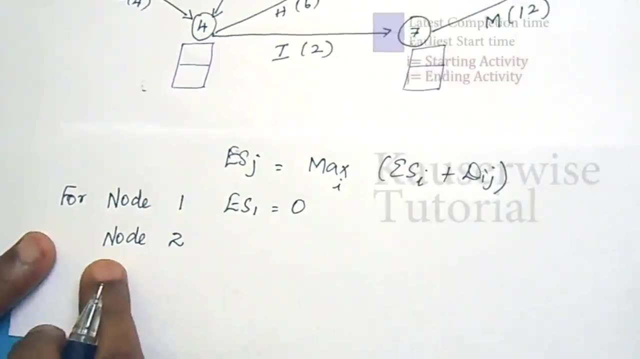 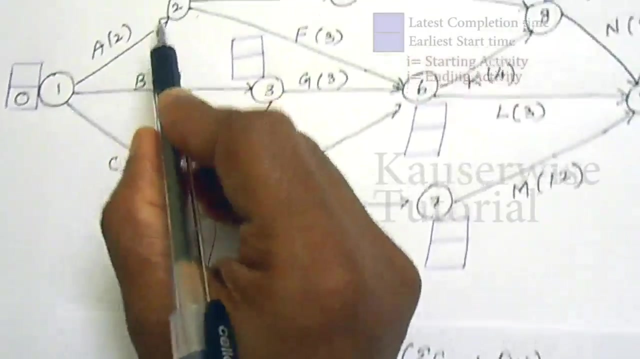 That is earliest Start I plus duration. Okay, So for node one earliest start time is always zero. Now you have to find out the node two. For node two, earliest start of I, I means for node two, which one is starting node. 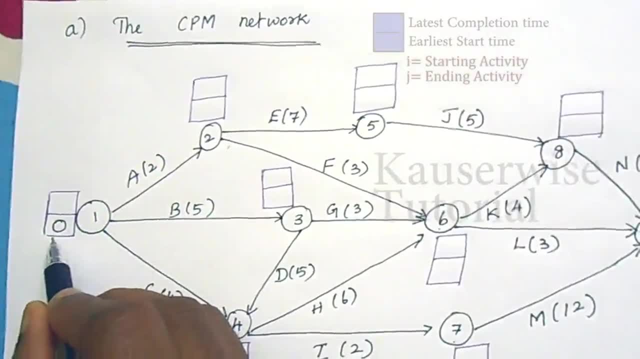 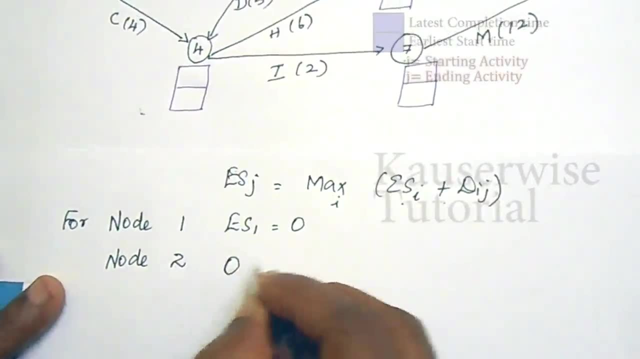 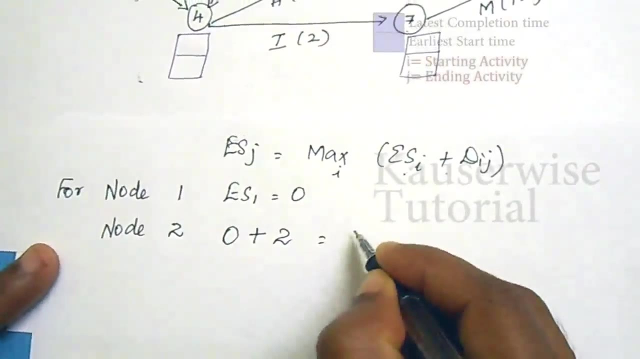 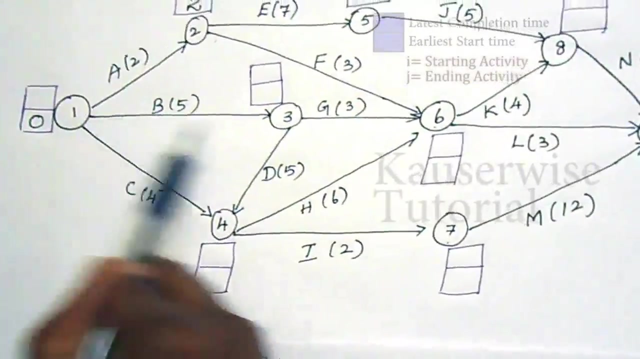 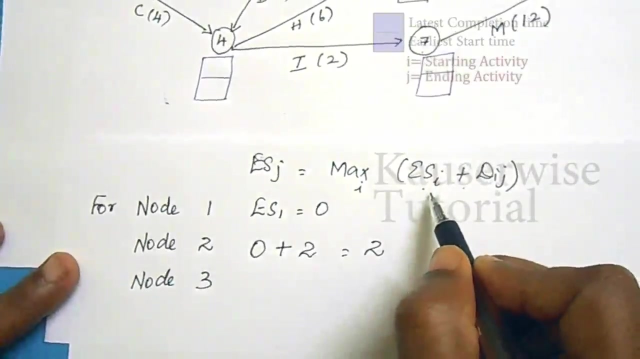 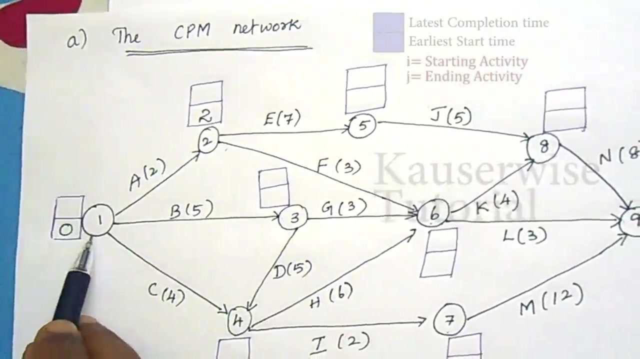 One is a starting node, Starting node. time is zero. Earliest start time is zero. So earliest start time of starting node plus duration: Zero, Zero. So for node two, earliest start time of starting node plus duration two: for activity, a duration is two, two answer two. so earliest start time of node two is two. in the same way for node three, same thing earliest start time of starting node plus duration. so for three, three is the ending node. which one is starting node? one is a starting node, starting node. earliest time is zero. 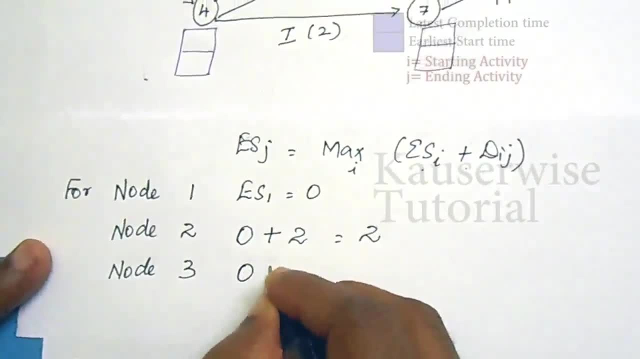 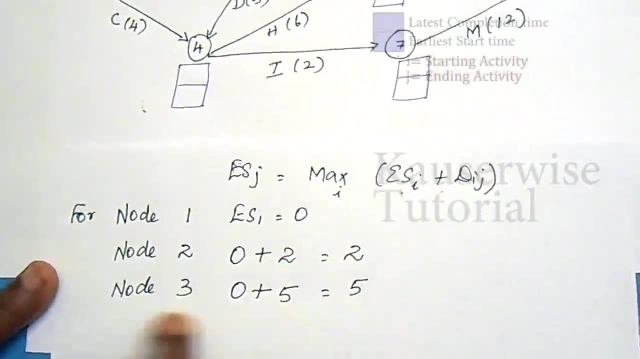 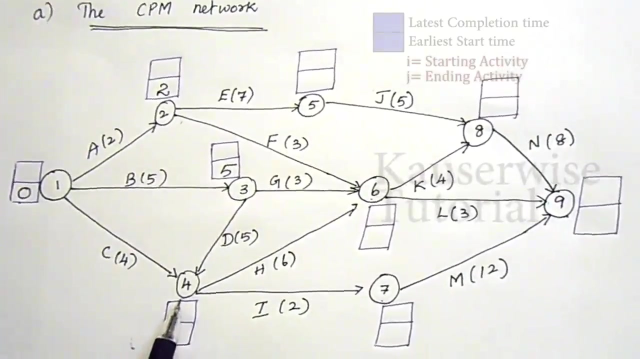 Okay, So for node two earliest start time is zero. Zero plus duration five. So five is the earliest start time for node three. Now for node four. here we have two options. One is starts from one to four and three to four. 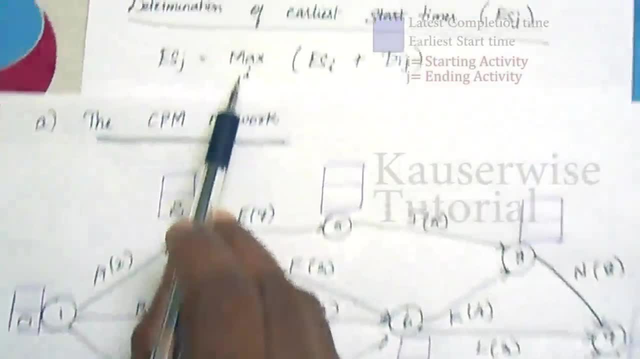 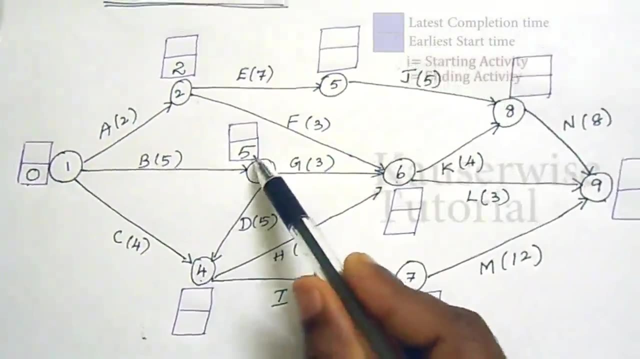 So two options are there Now. here you have to find out the maximum value. So for the forward pass we have to find the Maximum value. So previous one: starting time is five plus duration five, total ten. Look at the other option. 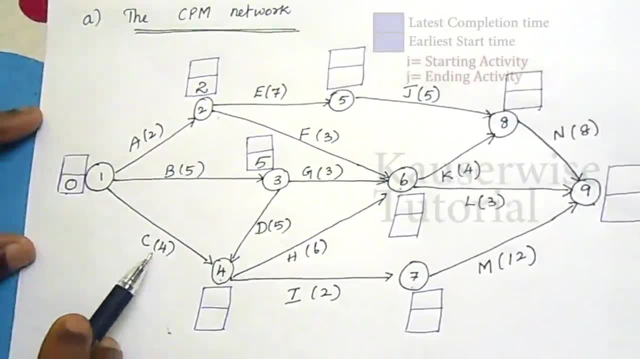 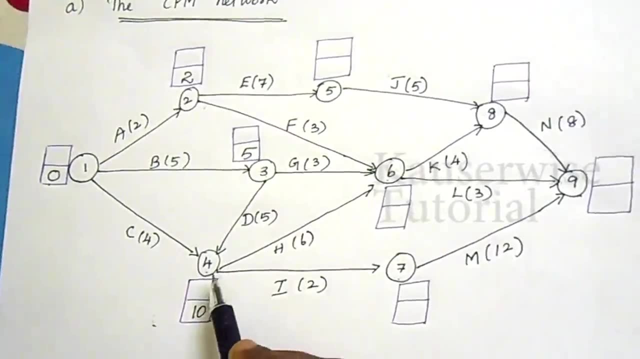 The starting node is one node, So starting time is zero plus four, four. So which one is maximum value? Ten is a maximum value, So we have to put only maximum value. Next, fifth one, So fifth one. for node five. only one options are there. 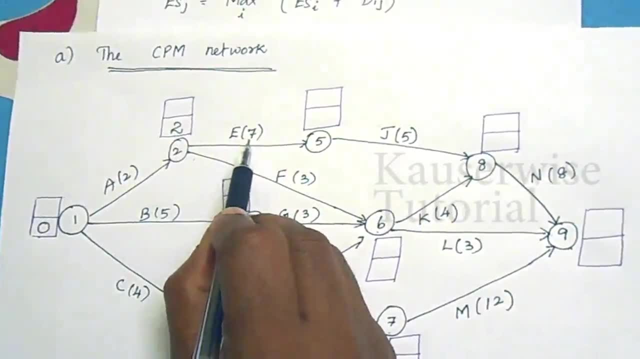 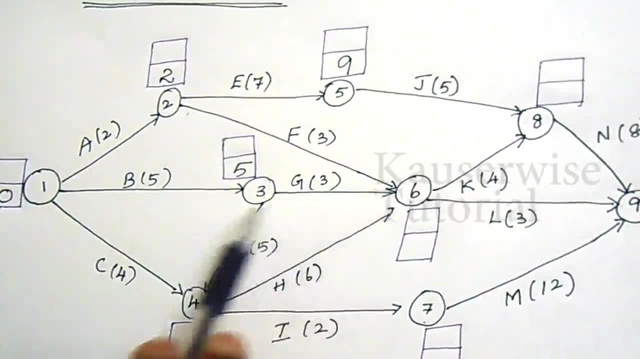 That is the previous one. starting time two plus duration seven, So nine. Look at the sixth node. Here we have three options. The first one is two to six and three to six, and last one four to six. So here you need to pick the maximum value. 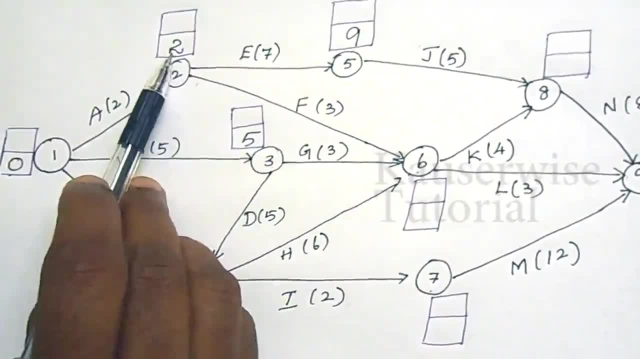 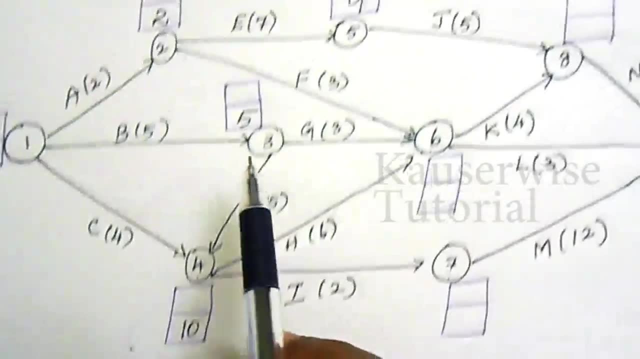 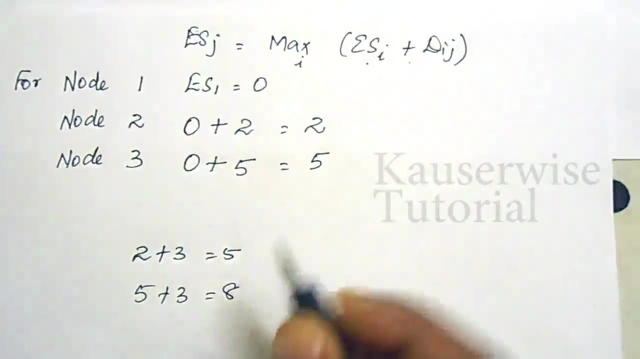 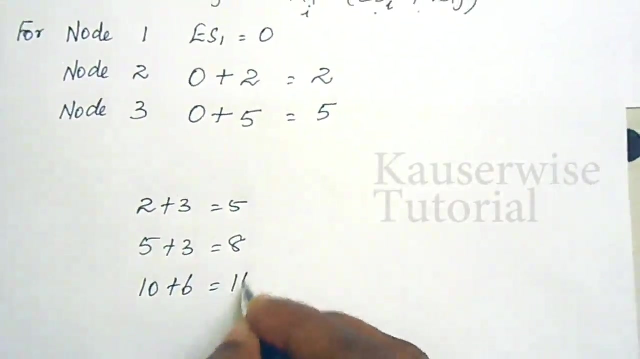 Look at the first option, Two to six. here Starting time is two plus three, five. And second option: starting time is five, five plus three, eight. Third option: Four to six, Timing ten plus six. So which one is maximum value? 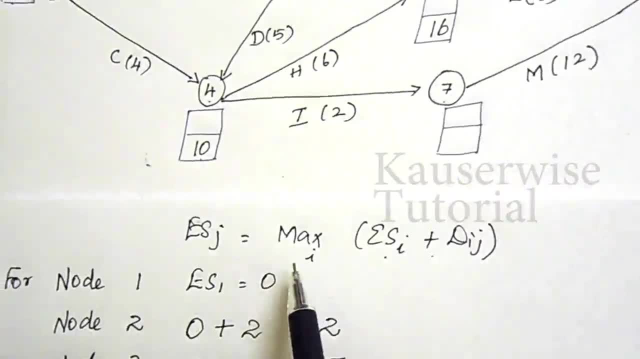 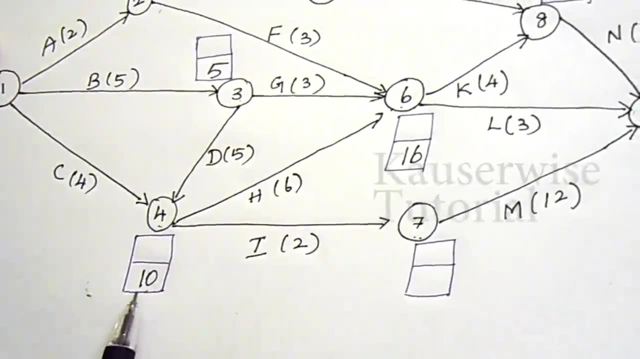 This one is a maximum value, So put 16.. So we need to find the maximum value. Look at the seventh node. Here we have only one option. The starting time is ten plus two twelve. The next node is eight, So here we have two options. 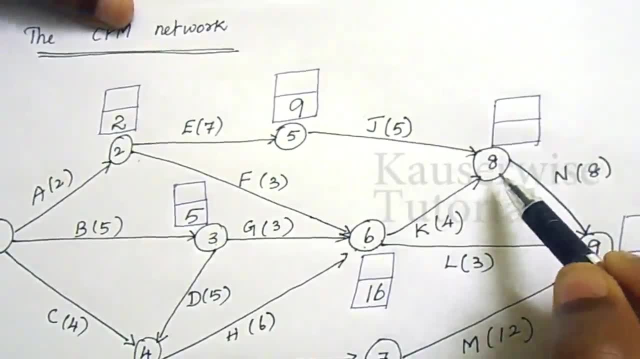 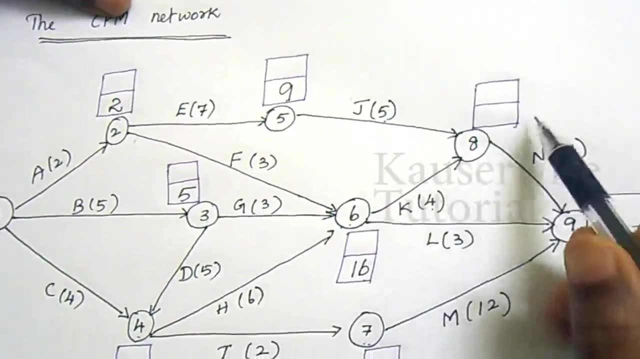 One is five to eight, Another one is six to eight. Now we have to pick the maximum value. So nine plus five, fourteen, sixteen plus four, twenty. So which one is maximum? Twenty is the maximum. Then look at the last node. 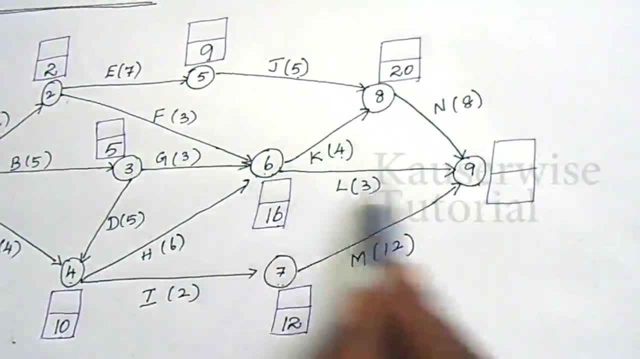 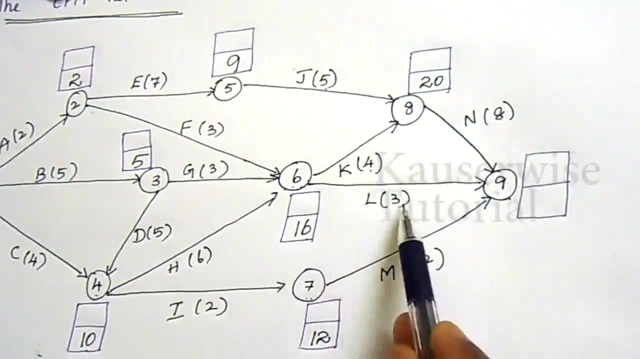 Here we have three options. One is eight to nine, six to nine and seven to nine. Here you have to pick the maximum value: Twenty plus eight, twenty-eight, sixteen plus three, nineteen, twelve plus twelve, twenty-four. So which one is maximum? 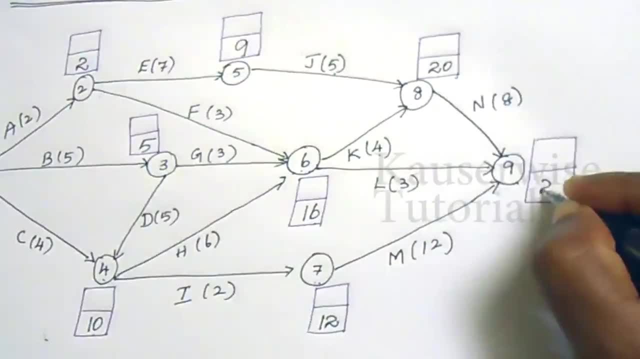 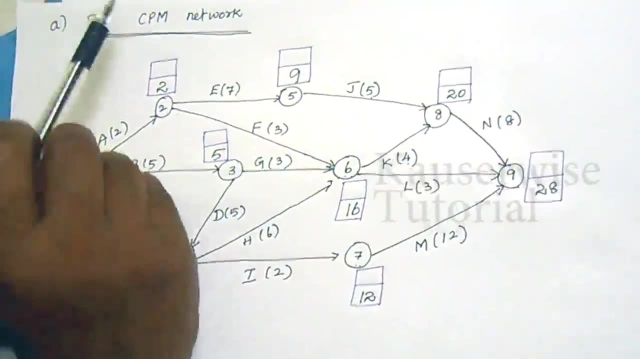 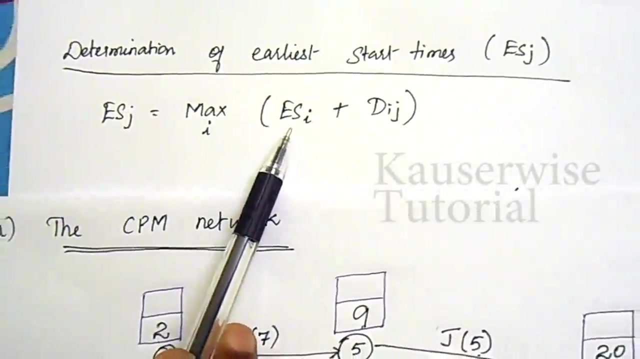 Twenty-eight is the maximum, That is twenty plus eight. twenty-eight, We have got earliest start time for each and every activity. according to this formula, Earliest start time of ending activity is equal to maximum of earliest start time of earliest one, That is, starting node plus duration. 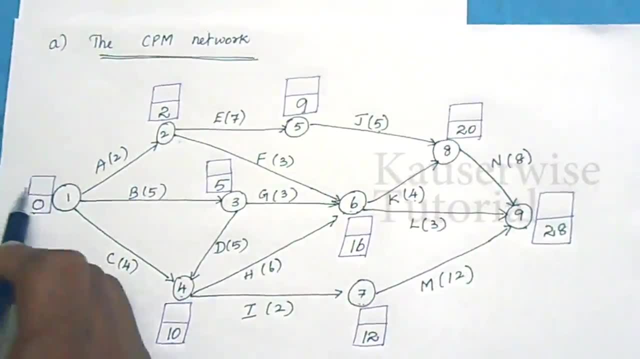 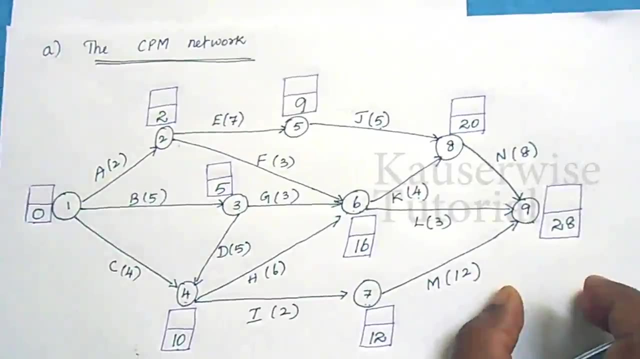 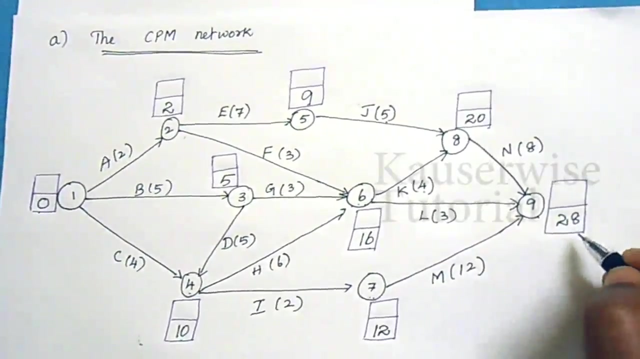 Now we need to find the latest completion time for each and every node. Okay, For this calculation you have to start from the ending node. This type of calculation is called as backward pass. For the last node, ninth node, Latest completion time is always is equal to earliest start time. 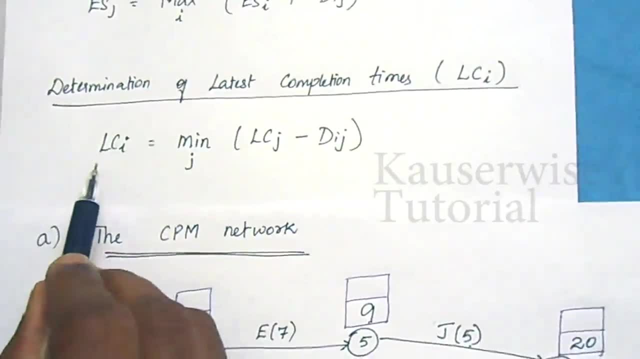 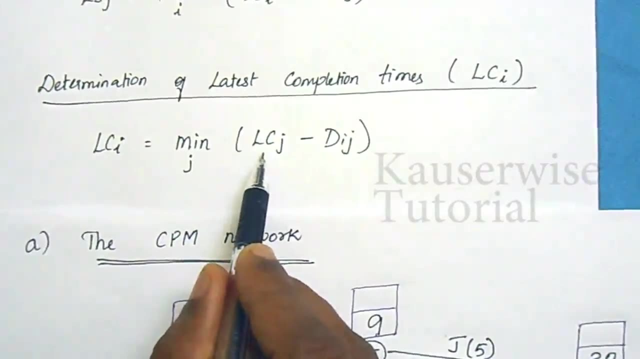 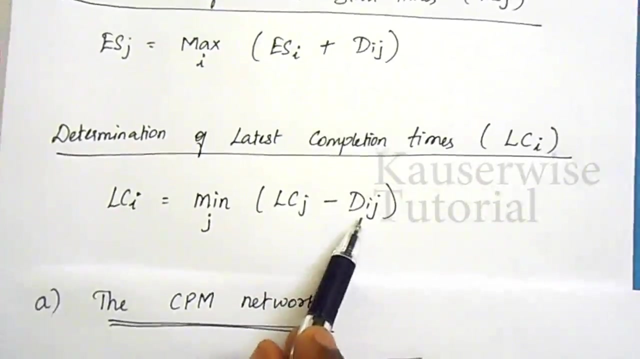 That is twenty-eight. Look at the formula: Latest completion time of i- i represents starting node- is equal to minimum of latest completion time of j minus duration. In the previous we have added the duration node. Here we need to subtract the duration from the latest completion time of jth activity. 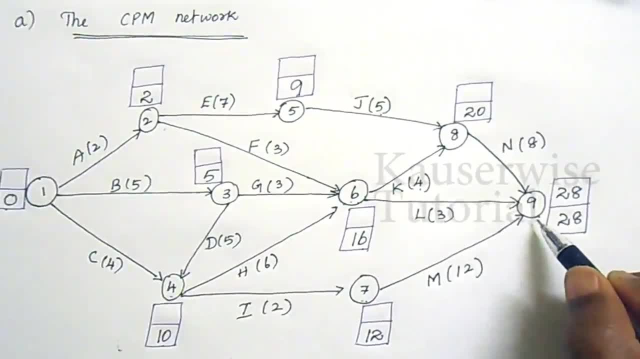 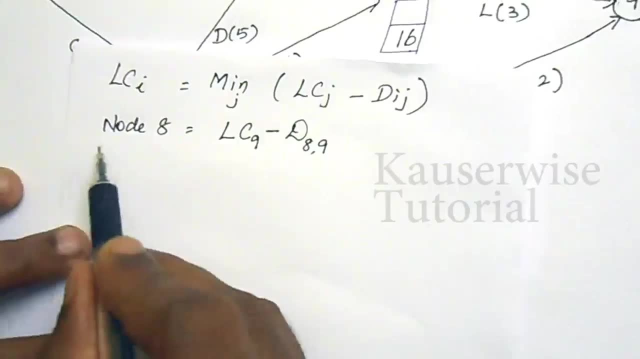 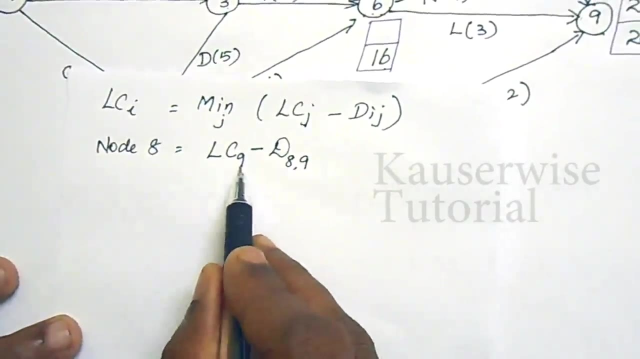 j represents ending activity. So we have calculated Latest completion time for 9th node. Now calculate latest completion time for 8th node. For node 8, latest completion of ending activity. j stands for ending activity, So ending activity is 9 minus duration of 8, 9.. 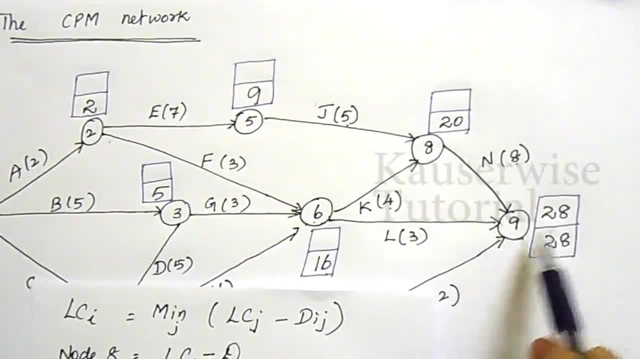 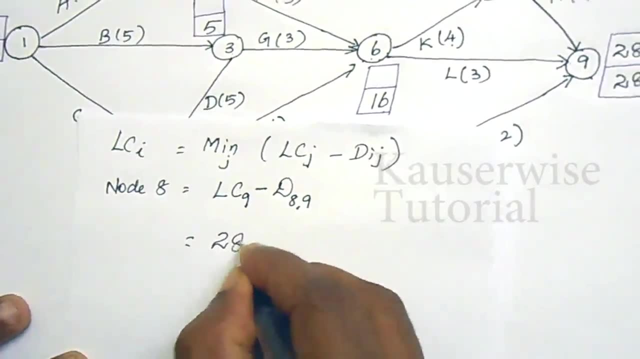 So 8, 9 duration is 8.. Ending activity: latest completion time is 28.. So latest completion time of 9th node is 28.. Minus duration of 8th node, 8 and 9.. 8 and 9 duration is 8.. 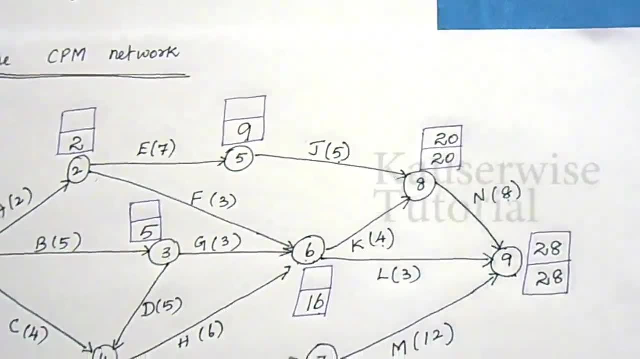 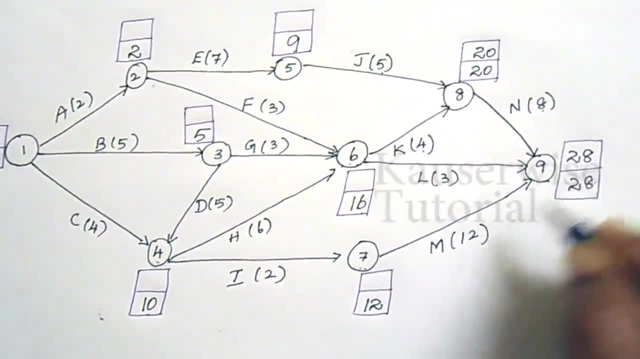 Answer 20.. In the same way for node 7.. Latest completion time of 9th node is 28 minus duration 12. You will be getting 16.. Look at the 6th node. Here we have two options. 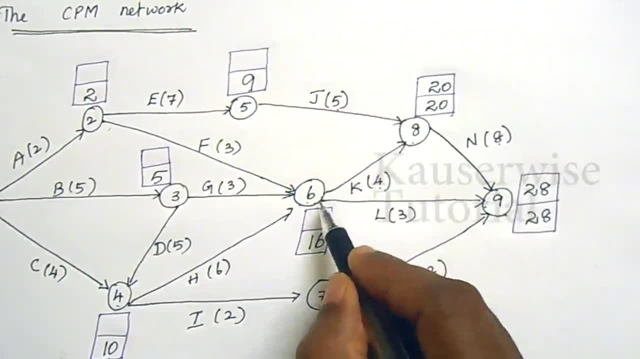 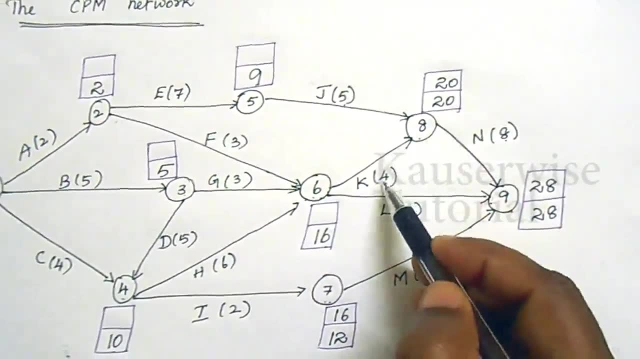 One is 9 to 6 and 8 to 6. Here you need to pick the minimum value, That is, 28 minus 3. 28. 25. 20 minus 4. 16. So which one is minimum value? 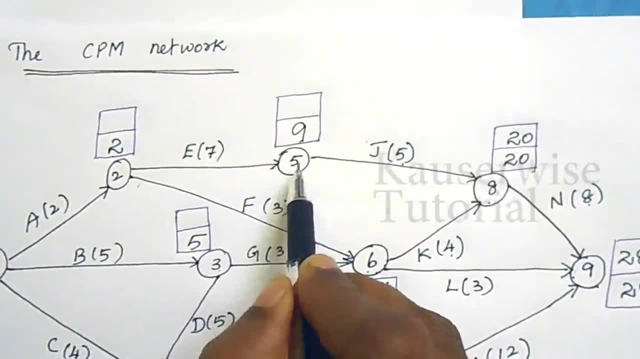 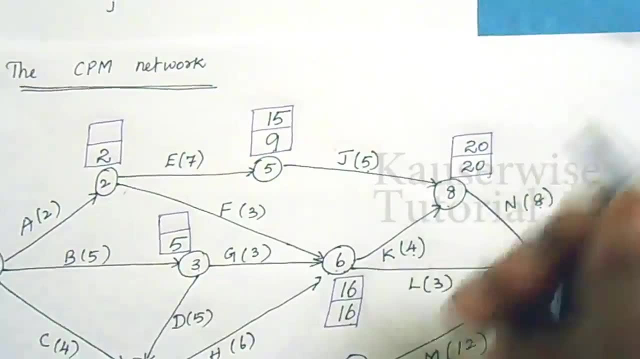 16 is the minimum value. Look at the node 5.. Okay, The earliest completion time of ending activity is 20.. Minus duration 5., So 15.. Then node 4.. For node 4, we have two options. 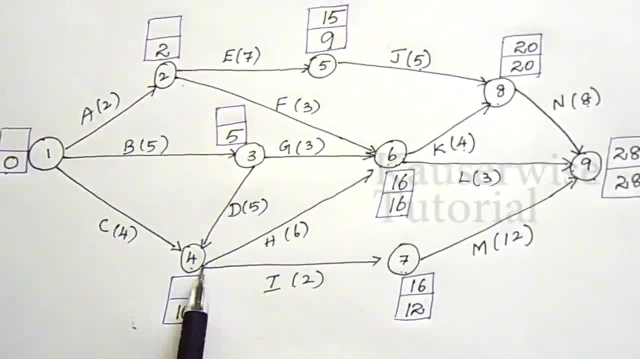 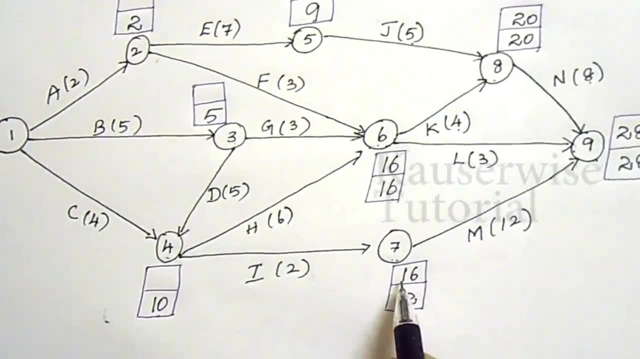 One is 7 to 4 and 6 to 4.. So two options are there Now. here you have to find out the minimum value. So look at the first option. The latest completion time is 16.. 16 minus 2 is 14.. 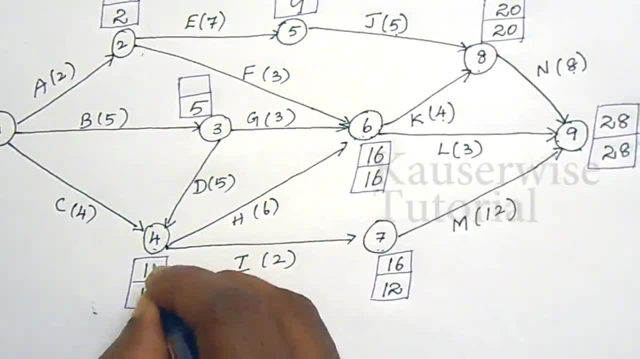 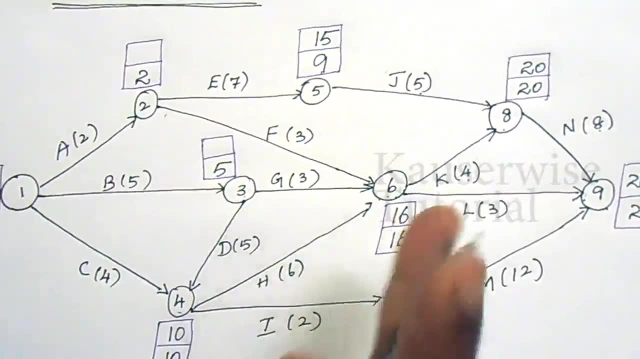 And here 16 minus 6 is 10.. So which one is least? 10 is the least value. Okay, Next node 3.. Look at the node 3.. Here also we have two options. One is 3 to 6 and 3 to 4.. 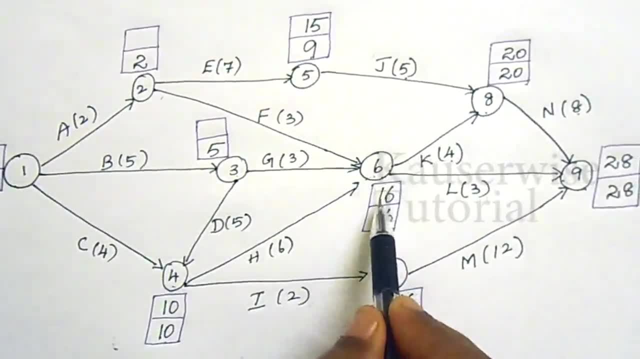 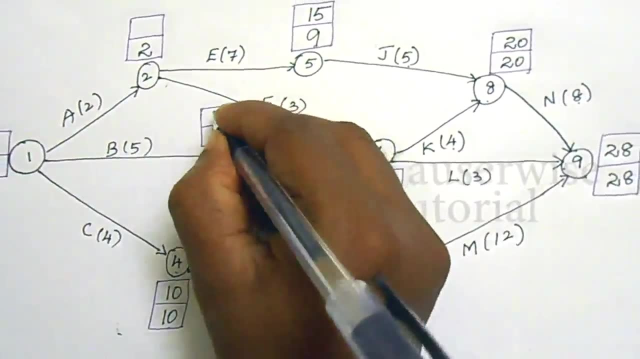 Now we have to pick the minimum value For the first option. 16 minus 3 is 13.. 10 minus 5 is 5.. So which one is least value? 5 is the least value. Okay, Now move on to the next node, 2.. 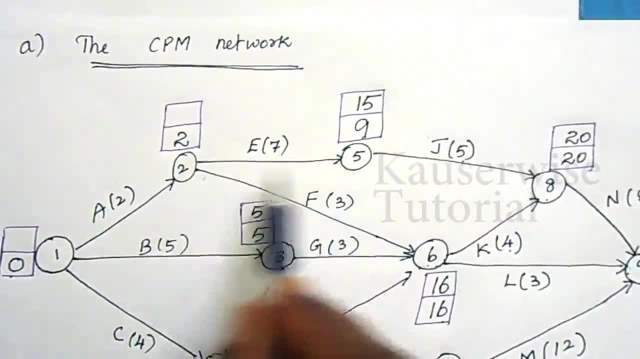 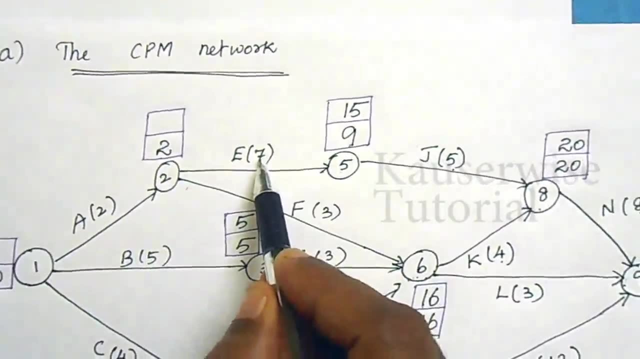 So here again we have two options. One is 5 to 2 and 6 to 2.. So two options are there. Just pick the minimum value: 15 minus 7, 8.. 16 minus 3, 13.. 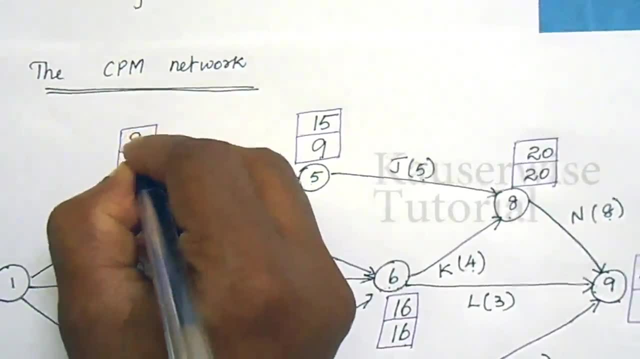 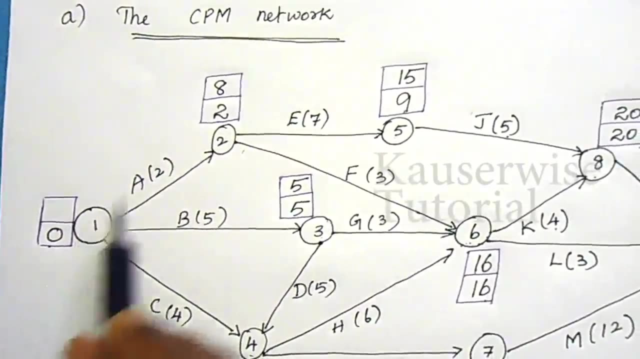 So which one is least? 8 is the least value. Move on to the last one, That is, node number 1.. For node 1, we have 3 options: One is 2 to 1,, 3 to 1, and 4 to 1.. 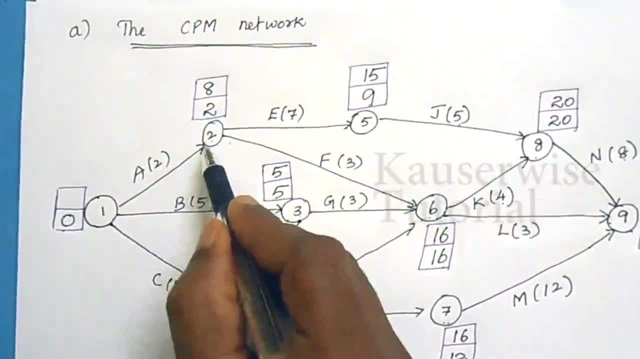 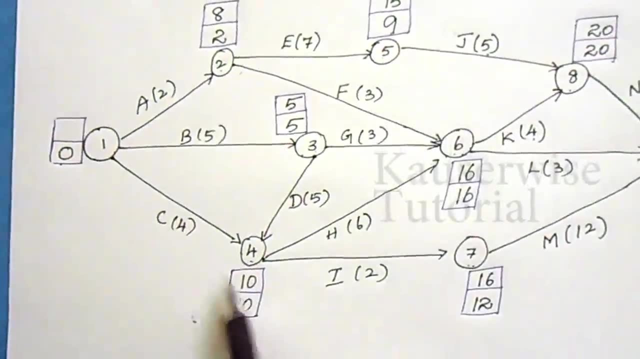 So here you have to find out the minimum value. Just see the first one: 8 minus 2, 6.. 5 minus 5, 0.. 10 minus 4, 6.. So which one is minimum value? 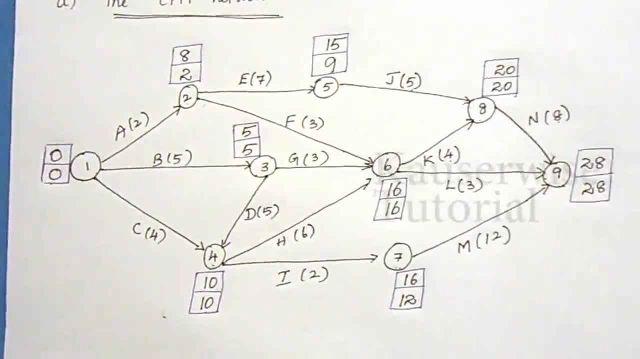 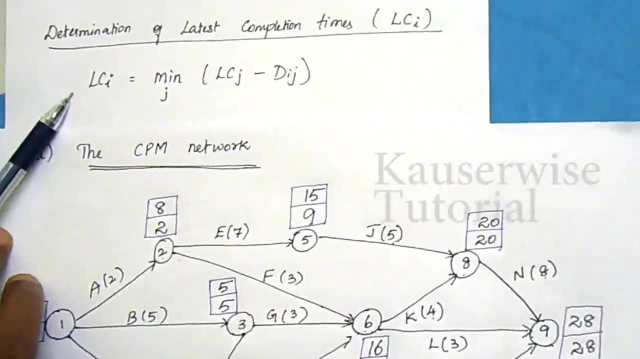 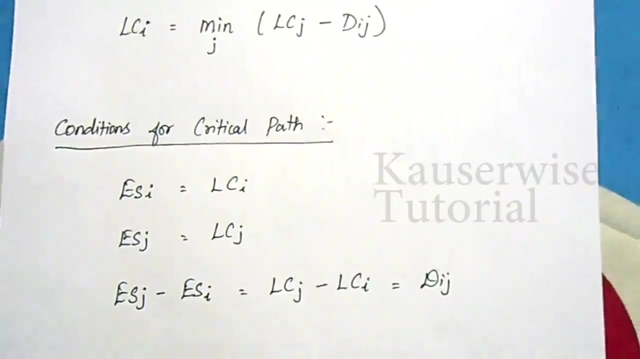 0 is the minimum value. So now we have calculated latest completion time of each and every node according to this formula. Now we need to find the critical path. So in order to find the critical path, we have three conditions. Look at the conditions for critical path. 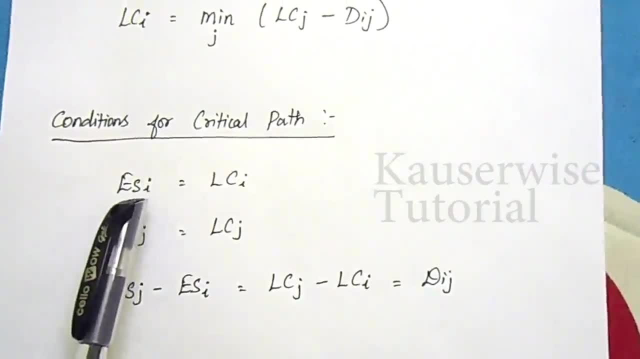 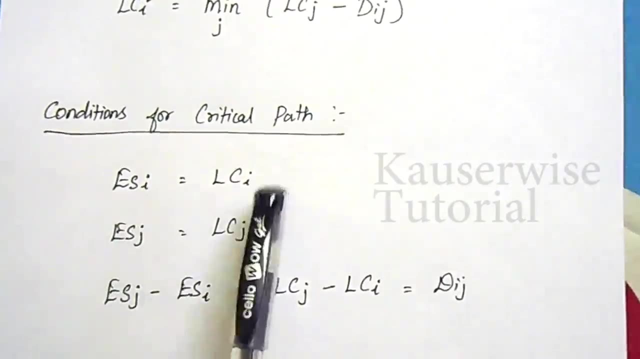 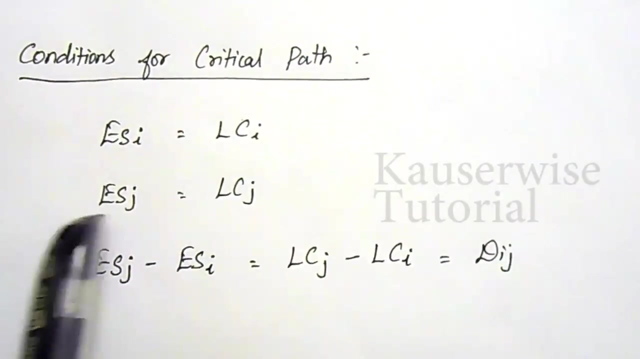 So the first condition is: earliest start time of starting activity is equal to latest completion time of starting activity. So both must be equal In the same way. for ending activity also, earliest start time is equal to latest completion time. This is the second condition. 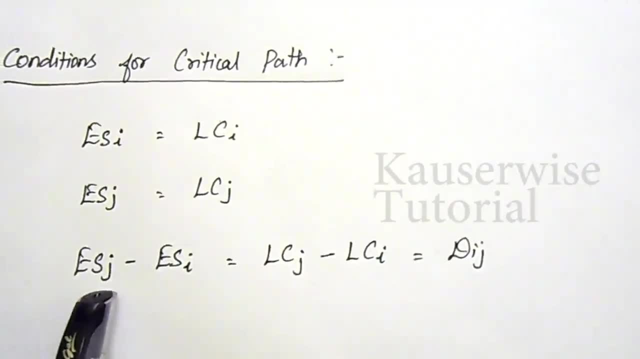 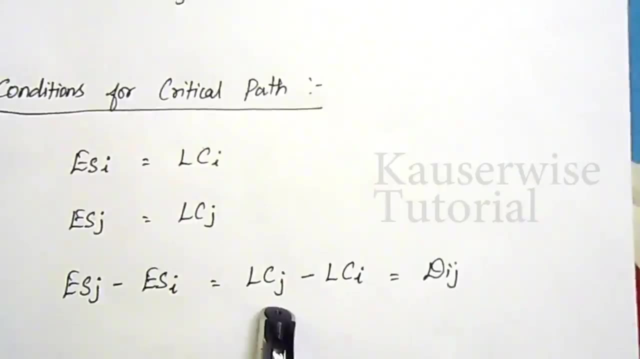 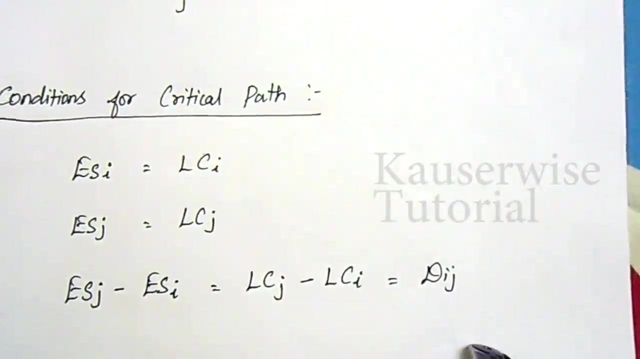 And third condition is earliest start time of ending activity. Ending activity minus earliest start time of starting activity is equal to latest completion of ending activity, minus latest completion time of starting activity is equal to duration. So these are the three conditions to be satisfied in order to 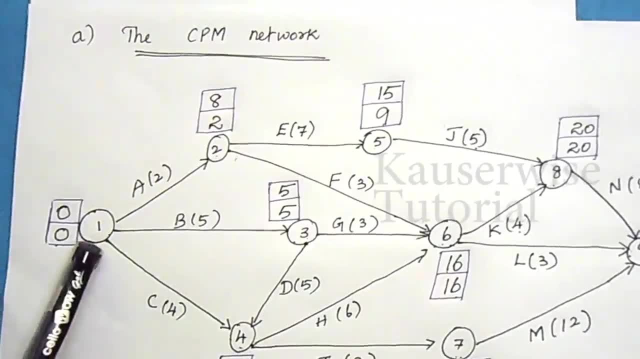 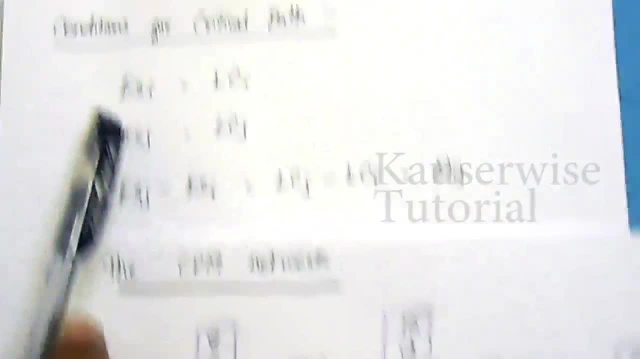 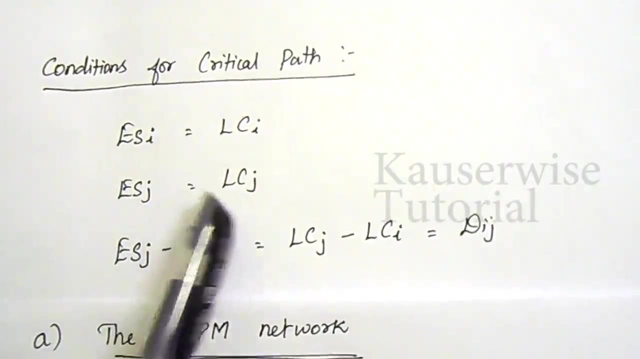 consider a particular activity as critical path. Look at the first node. Early start time is 0 and latest completion time also 0. So first condition is satisfied. Look at the second condition: Early start time of ending activity is equal to latest completion of ending activity must be equal. 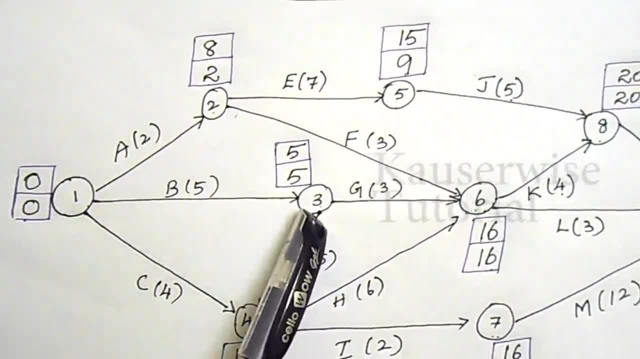 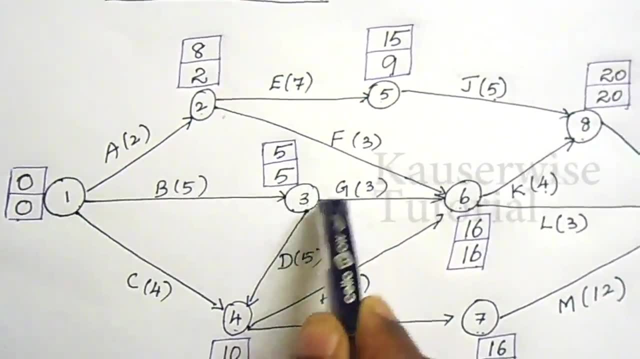 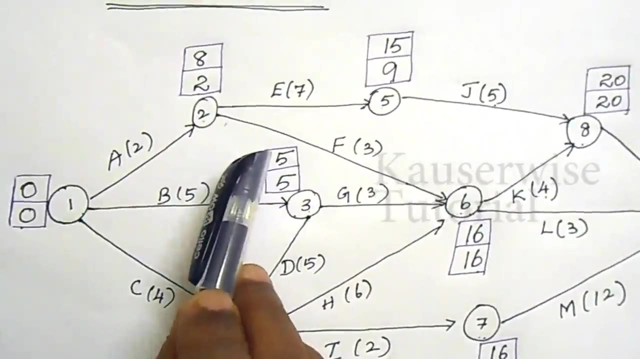 So here starting node is 1, ending node is 3.. Look at this path. The ending activity is 3.. Node 3 represents ending activity. So ending activity earliest start time is 5.. And ending activity latest completion time also 5.. 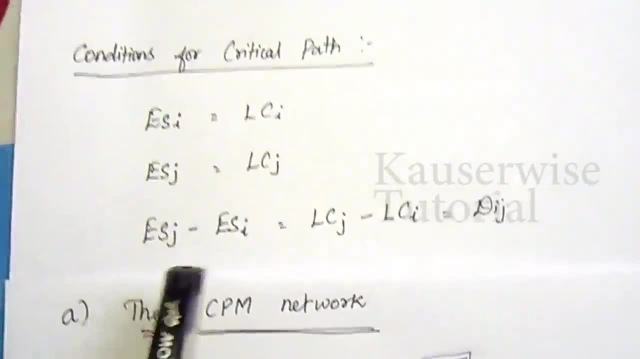 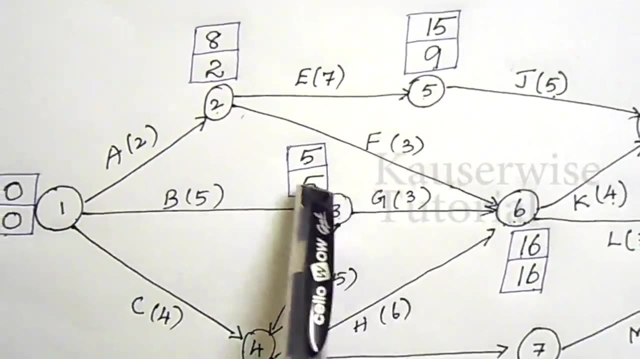 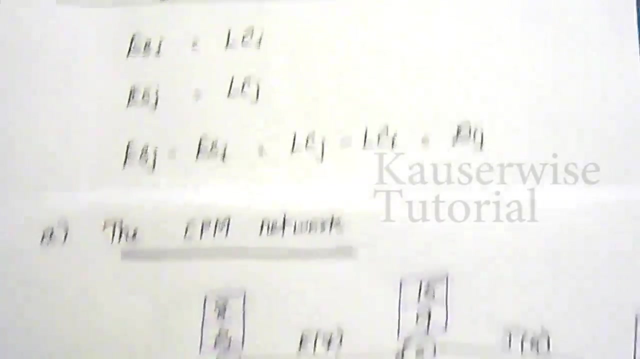 So condition number 2 also satisfied And look at condition number 3.. Early start time of ending activity, That is, the ending activity- is 5.. Early start time is 5.. And early start time of starting activity- Starting activity- is 0.. 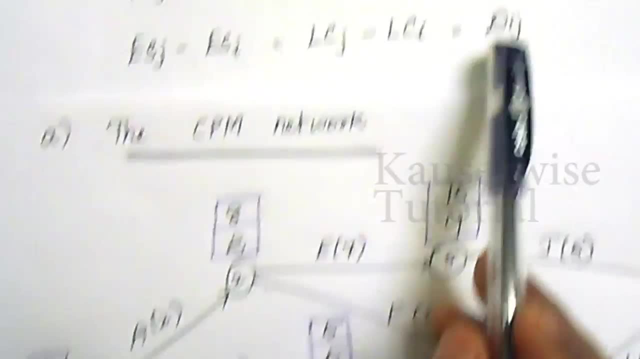 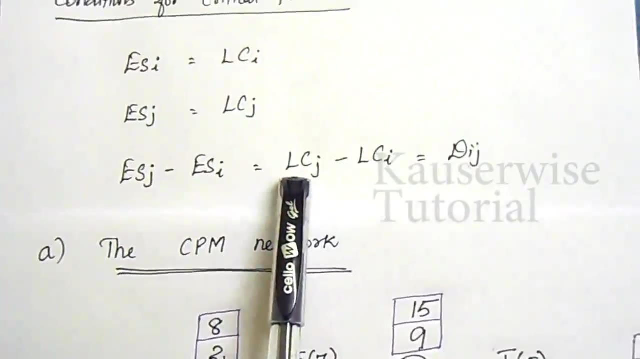 So 5 minus 0 is equal to duration, That is 5.. Okay, in the same way, latest completion time of ending activity. So for the first condition, 0 is equal to duration. So for the first condition, 0 is equal to duration. 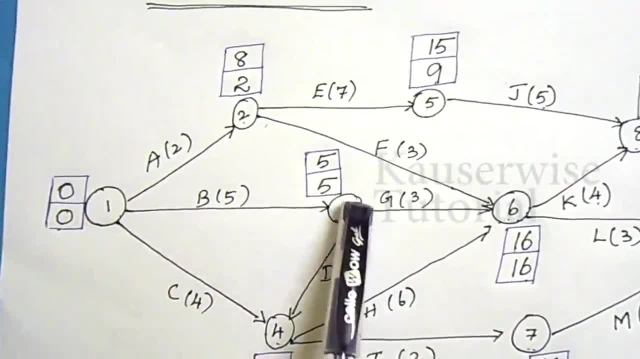 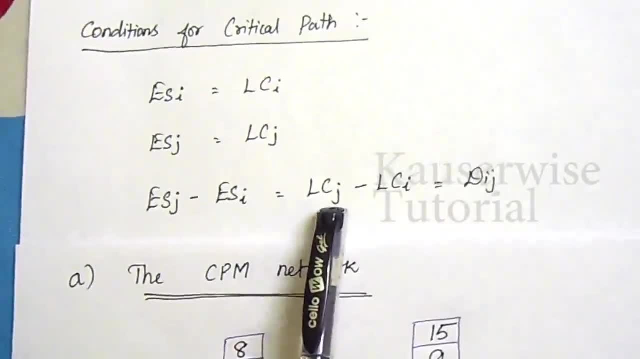 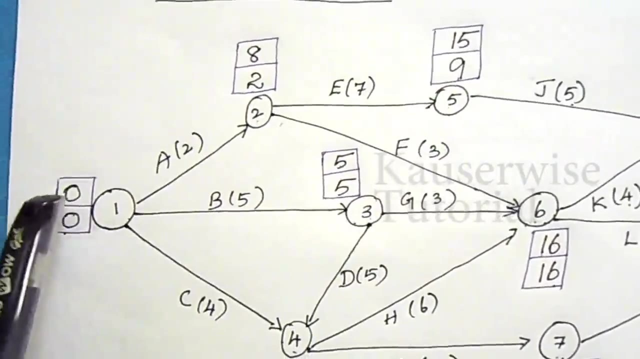 For activity B, then ending activity is 3.. Okay, so for node 3, latest completion time is 5.. Latest completion time of ending activity 5 minus latest completion time of starting node- Starting node- is 1.. So latest completion time is 0.. 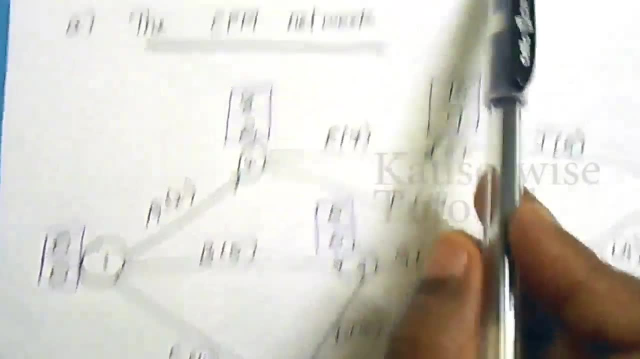 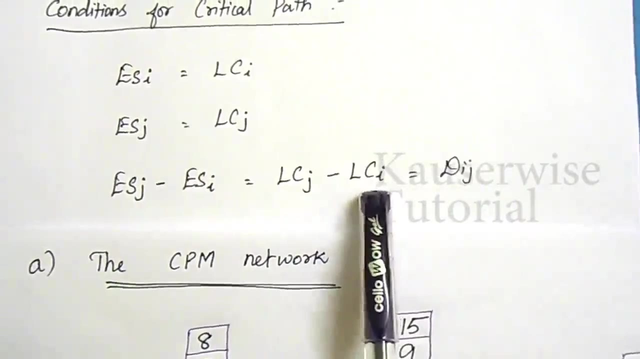 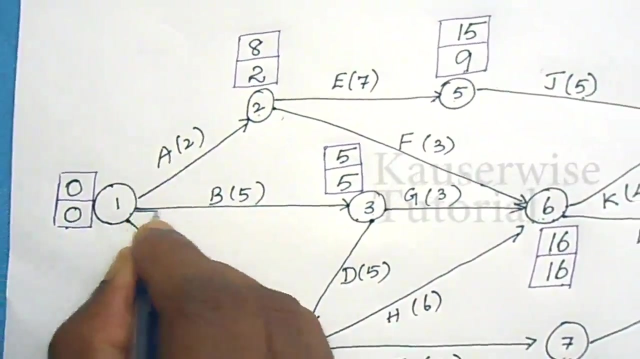 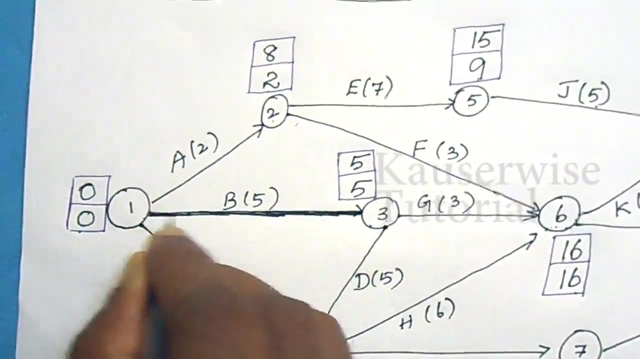 5 minus 0 is equal to 5. That is LC minus That is latest completion time of J minus Latest completion time of I is equal to duration. So third condition also satisfied, Then it will be a critical path. So put one double line to identify, to highlight the critical path. 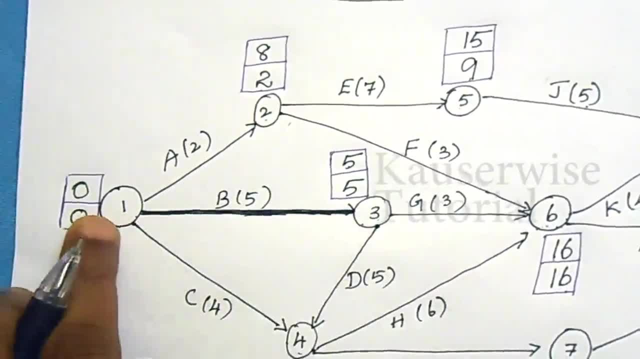 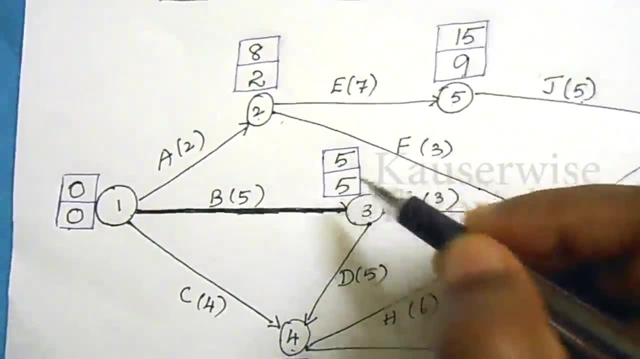 Just darken the line for identification. So 1, 3 is a critical path. Okay, so both starting time and completion time must be equal. Then move on to the next one, from 3 to 4. here 10,, 10.. 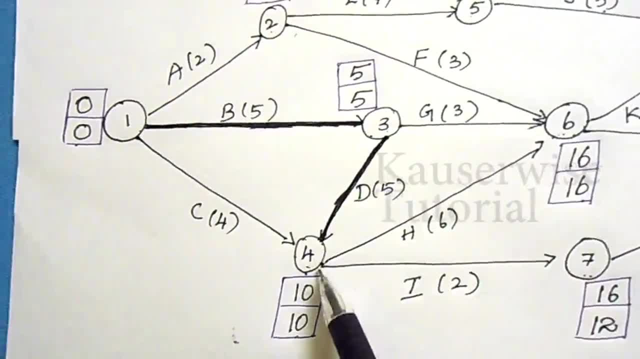 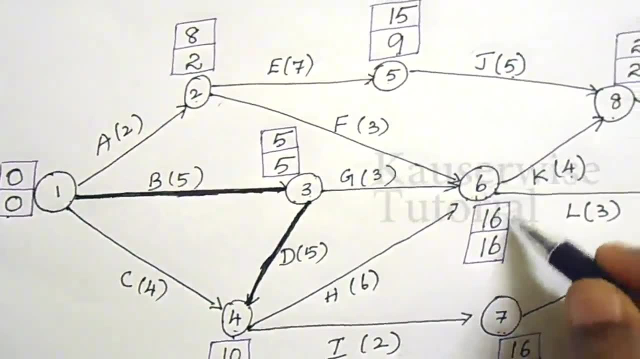 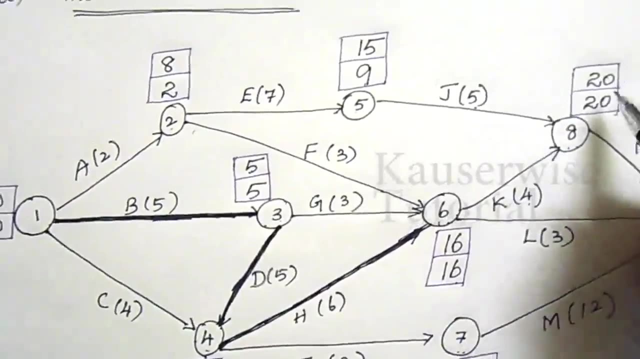 This is also a critical path. Then next here, from 4 to 6.. Here also we have starting time and completion time is equal, So it is also a critical path. Then from 6 to 8, 20,, 20 equal. 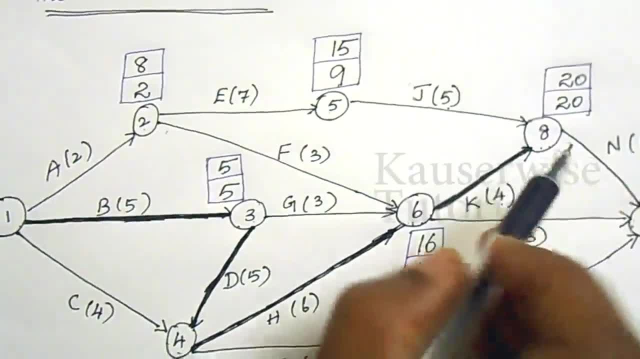 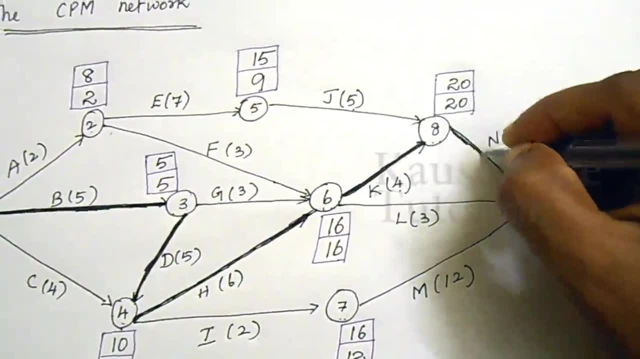 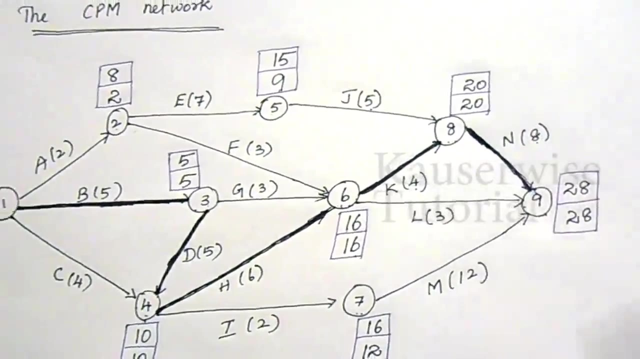 So this is also a critical path. Then 8 to 9,, 28 and 28: equal, So this is also a critical path. So critical path means longest path is called critical path. So each and every node of critical path, that is, starting time and ending time, completion time, will be equal. 0, 0,, 5,, 5,, 10,, 10,, 16,, 16,, 20,, 20,, 28 and 28.. 1 to 3,, 3 to 4,, 4 to 6,, 6 to 8.. 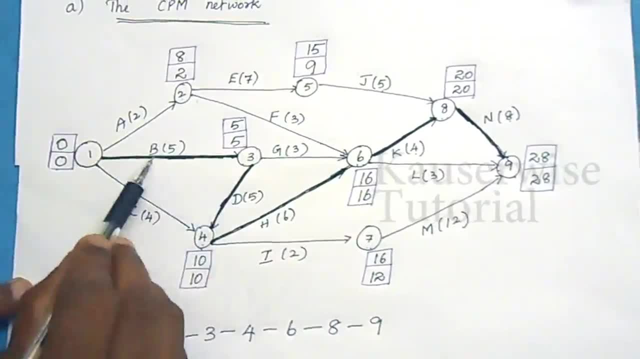 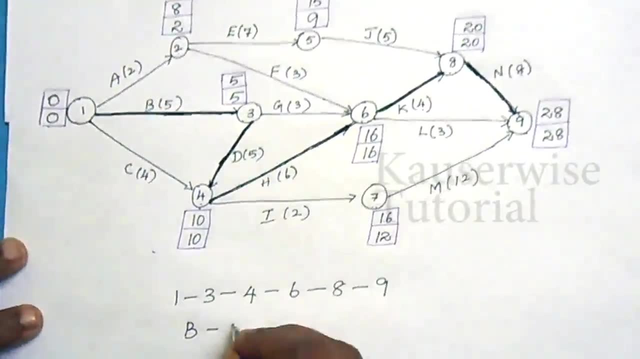 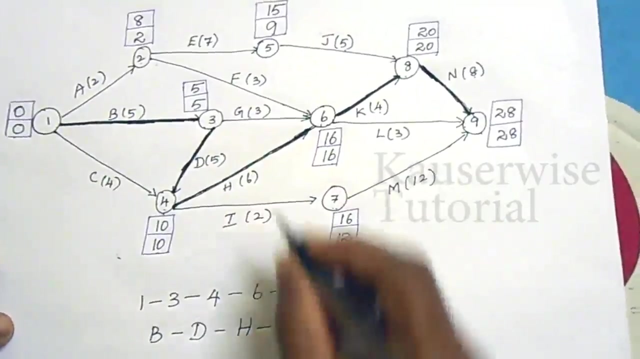 And 8 to 9.. See 1 to 3 represent activity B, So B activity B, Then 3 to 4, activity D, Then 4 to 6, activity H, Then 6 to 8, activity K. 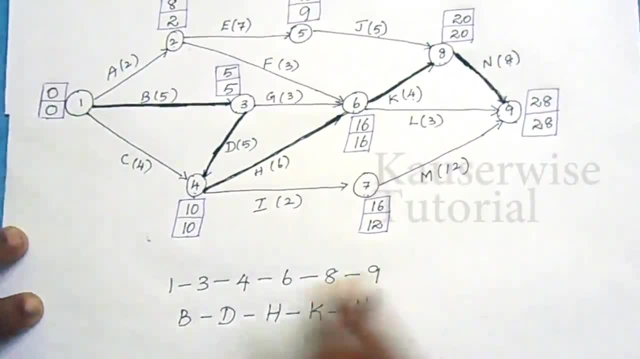 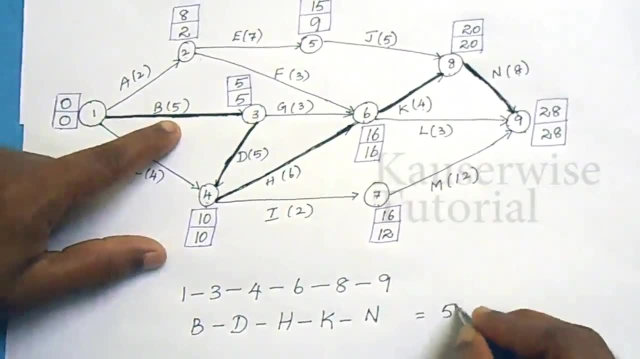 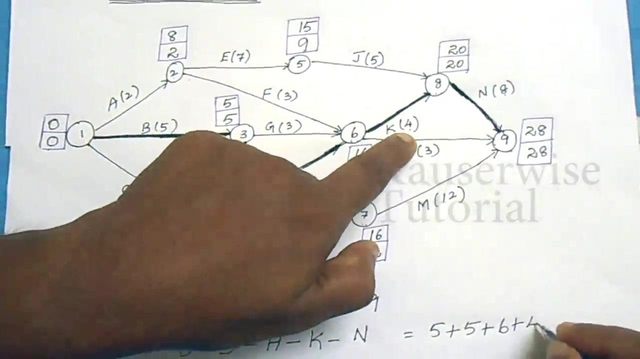 Then 8 to 9, activity N. So this is critical path. Now we have to find out the total duration of this critical path. Duration is 5, plus 5, plus 6, plus 4, plus 8, 28.. 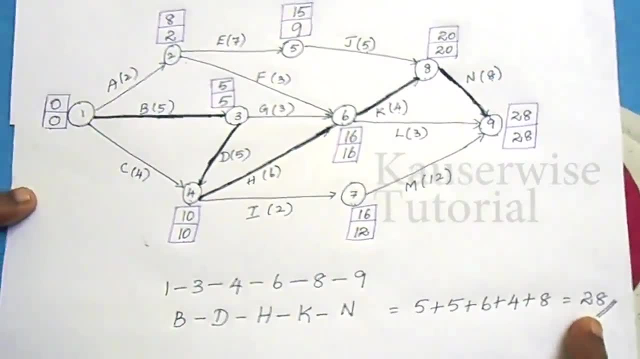 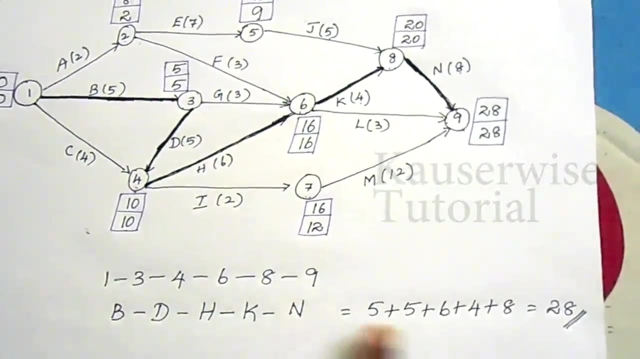 So critical path duration is 28.. This is a critical path, That is, B to D, D to H, H to K and K to N is a critical path And project completion time is 28 months. Look at the problem. So far we have done. 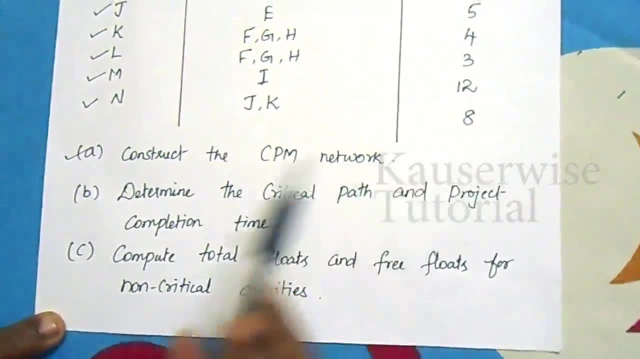 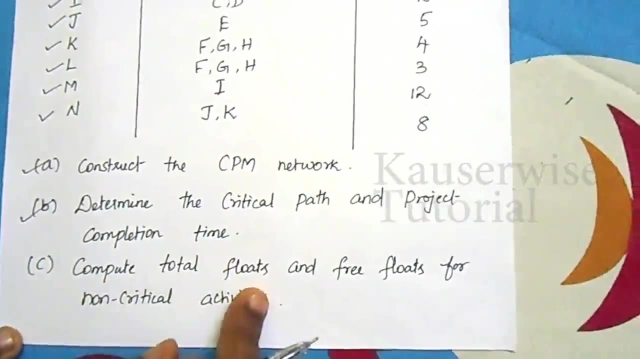 Two things. The first one is: construct the CPM network is over. And second one, determine the critical path and project completion time. This is also over. The last one is compute total float: total floats and free floats for non-critical activities. 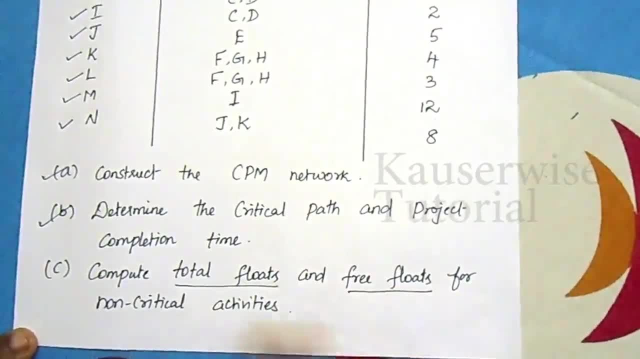 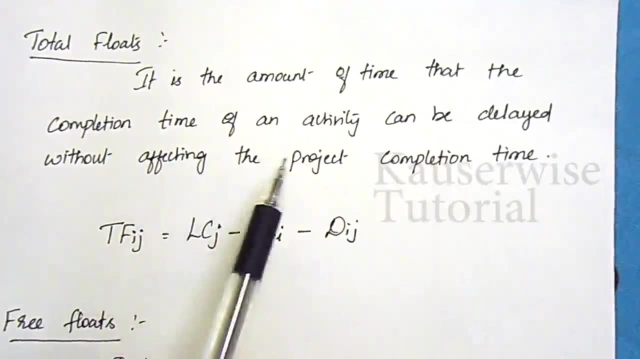 So now we have to calculate the total floats and free floats for non-critical activities. So total float means it is the amount of time that the completion time of an activity can be delayed without affecting the project. So the project completion time is called total floats. 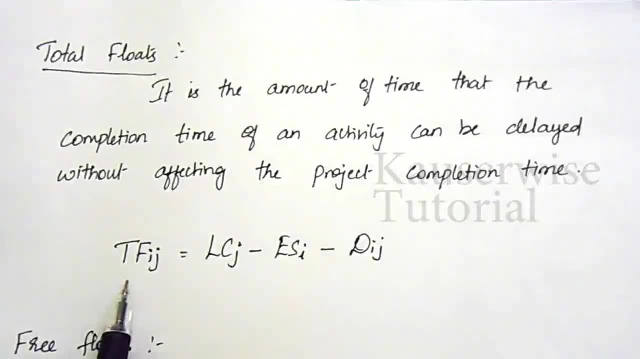 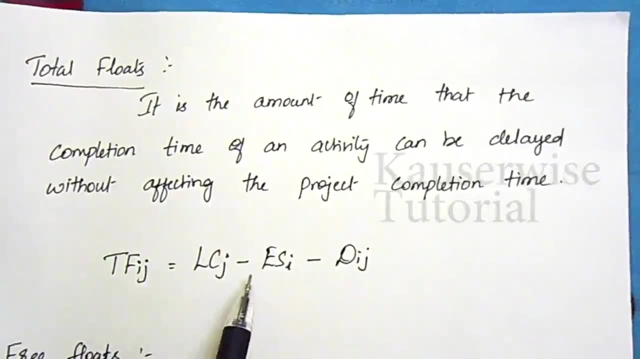 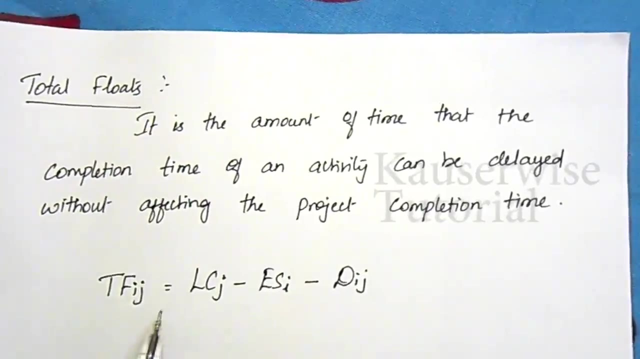 Okay, here we have one formula in order to calculate the total float for each and every activities. This is the formula that is the latest completion time of ending activity, minus the earliest start of starting activity, minus duration of one particular activity. So this is a formula to find out the total float. 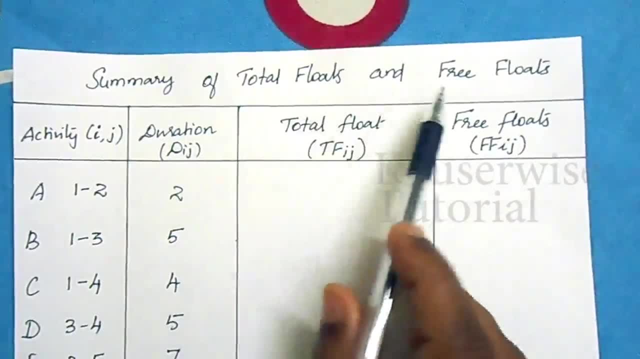 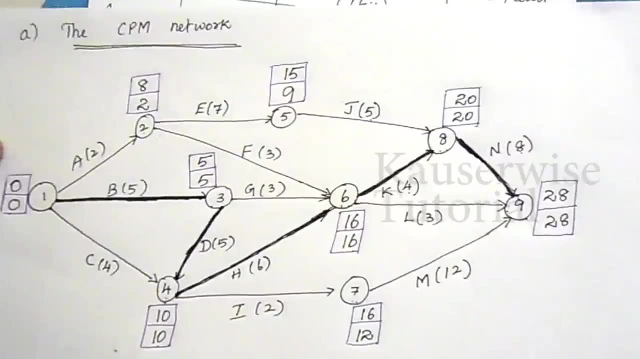 Now look at the calculation summary of total floats and free floats. So first column is activity, That is A, B, C, D till N. Look at the diagram: Activity A, node 1 to 2.. Activity B, node 1 to 3.. 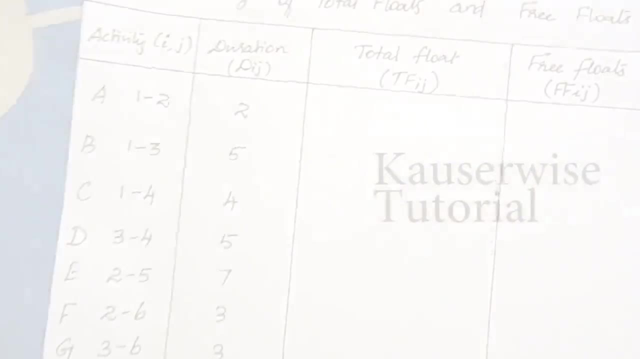 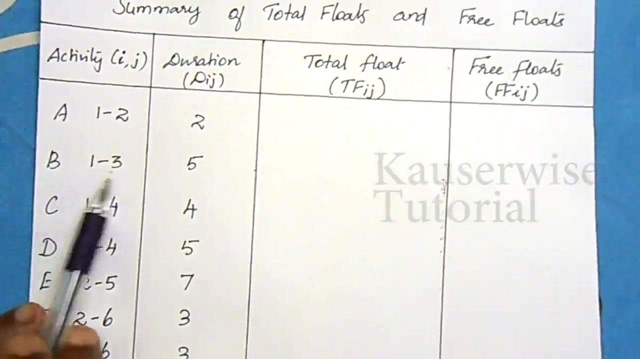 Activity C, node 1 to 4.. Okay, in the same way, I have written the node for each and every activity separately: For activity A: 1 to 2.. For activity B: 1 to 3.. For activity C: 1 to 4.. 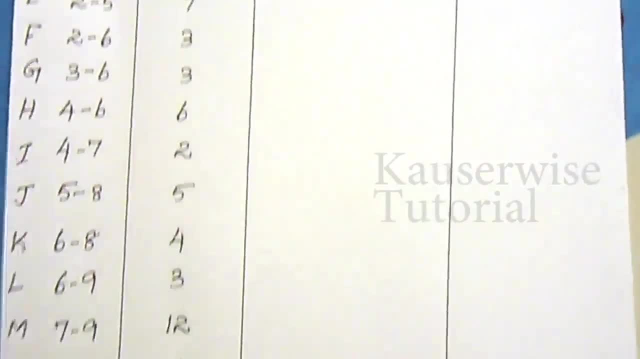 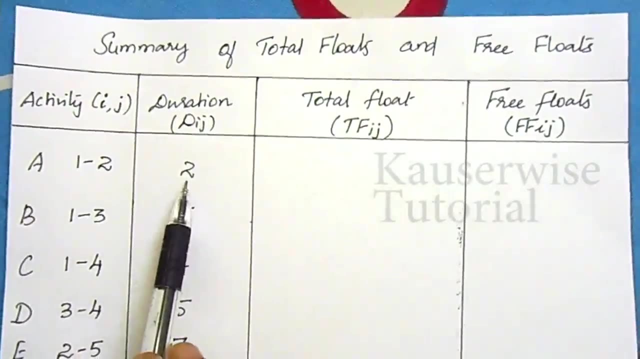 For activity D 3 to 4.. In the same way, I have written the nodes for each and every activity, And this is a Column for duration D, I, J. For activity A, duration is 2.. For activity A: duration 2.. 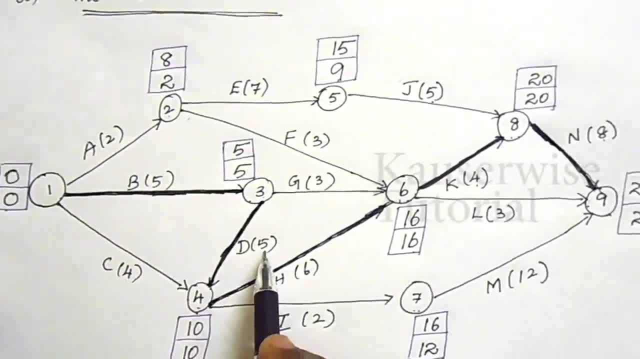 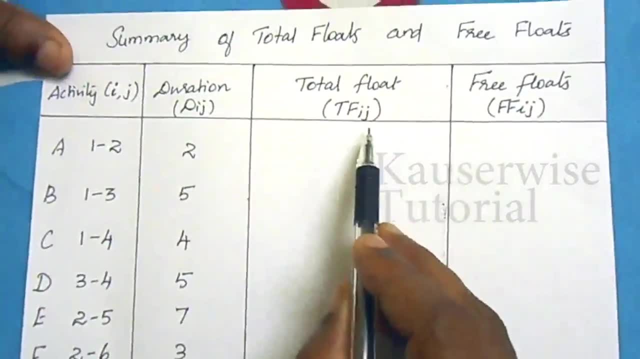 For B, 5. For C, 4. For D: 5.. So this is the duration for all the activities from A to N. Now we need to find the total float with the help of the formula. This is the formula for total float. 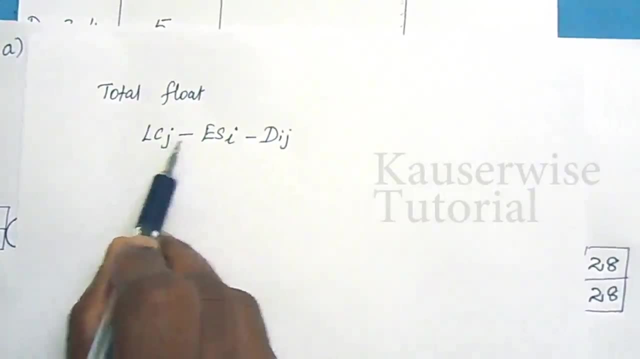 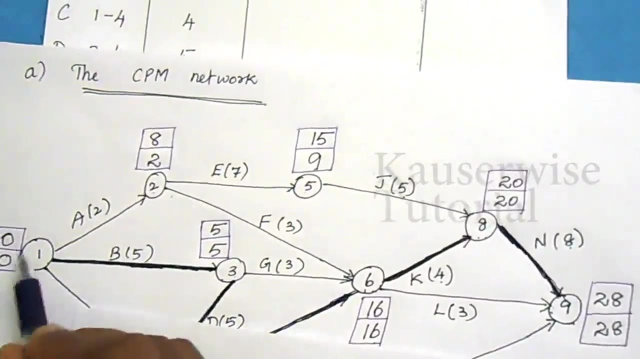 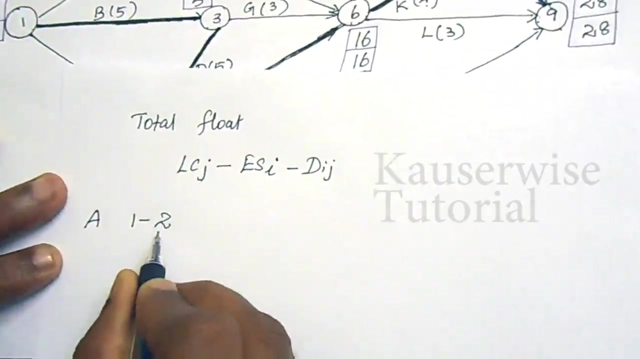 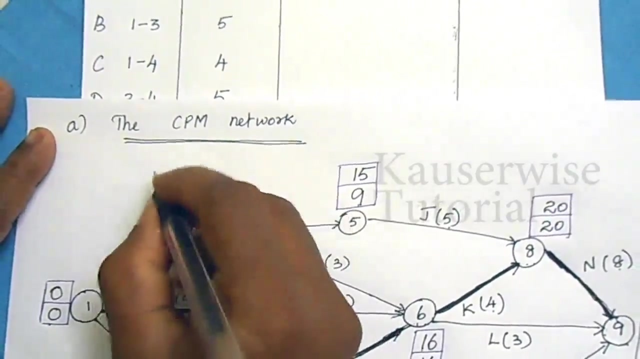 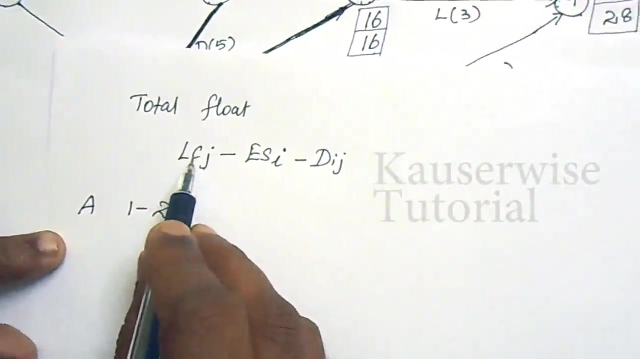 That is the latest completion time of ending activity, minus earliest start of starting activity, minus duration. For activity A: see node 1 to 2, 1 to 2, so latest completion of ending activity. ending activity is 2, see the lower square represent earliest start, the upper square represent latest completion. this is common for all the nodes. okay, so for total float, latest completion time of ending activity for activity A: node 1 is a starting node and 2 is a ending node. 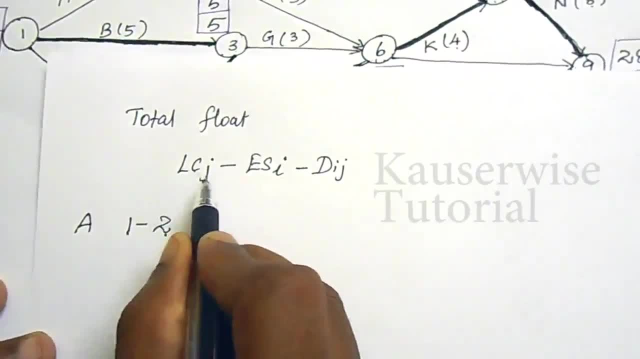 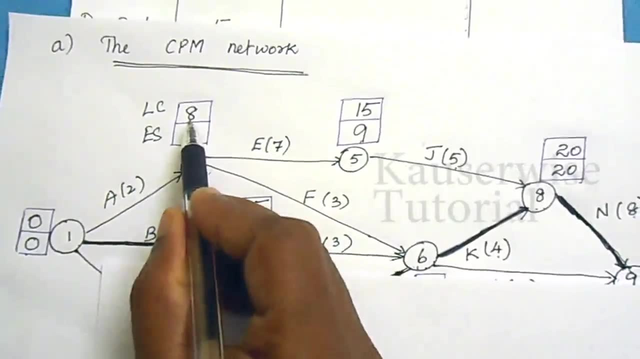 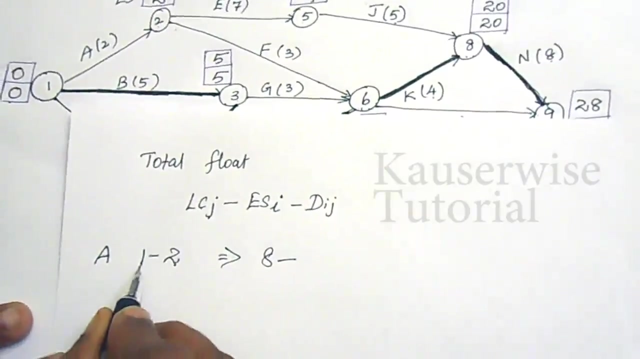 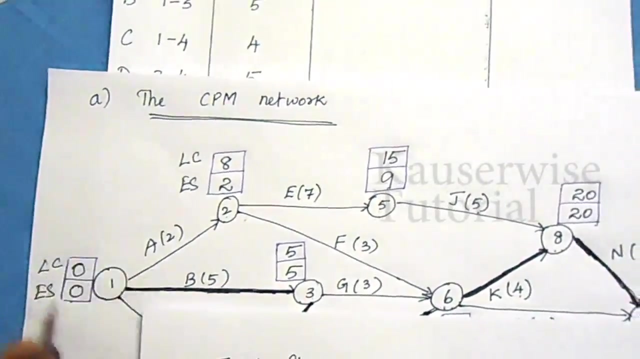 Okay, Okay, Okay. So just apply the formula latest completion time of 2, that is, ending node is 2, no, so latest completion time is for node 2, latest completion time: 8, 8 minus earliest start of starting node. starting node is 1, no, so for node 1, earliest start time. so this one is earliest start and this one is latest completion, so earliest start time is 0, 0 minus duration of ending activity. 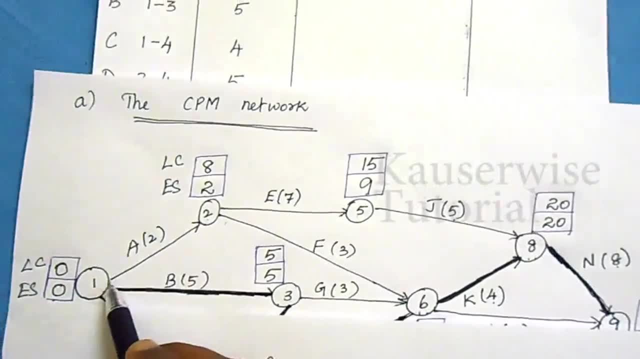 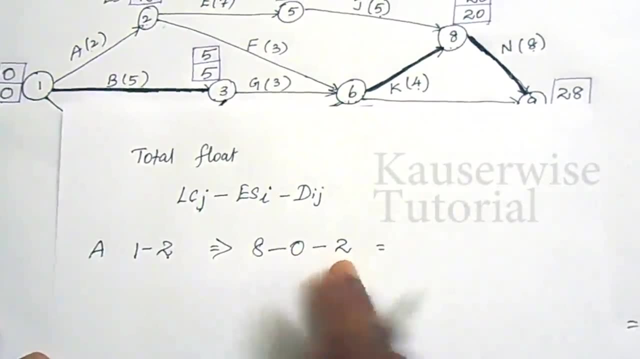 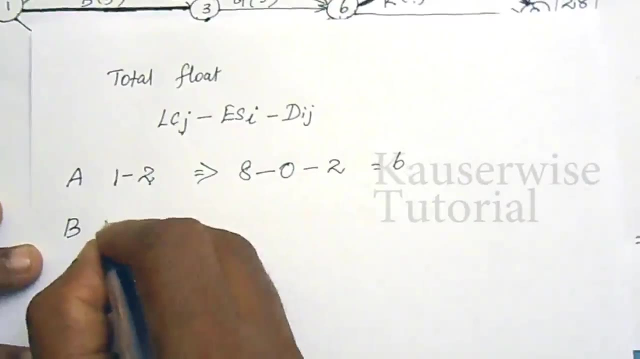 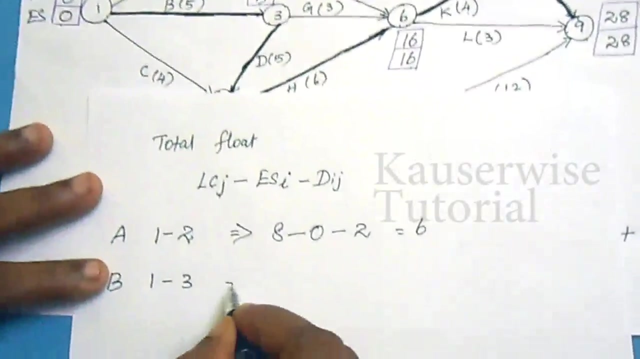 This particular activity 1 and 2, so what is the duration for 1 and 2,, 2, 2,. so answer: 8 minus 0, 8, 8 minus 2, 6,. total float for activity A is 6,. for activity B: 1 to 3, see activity B, node 1 to 3,. okay. so latest completion time of node 3, for node 3, latest completion time of node 3 is 6,. so this one is earliest start of starting node. so latest completion time of node 3, for node 3, latest completion time of node 3, 6.. 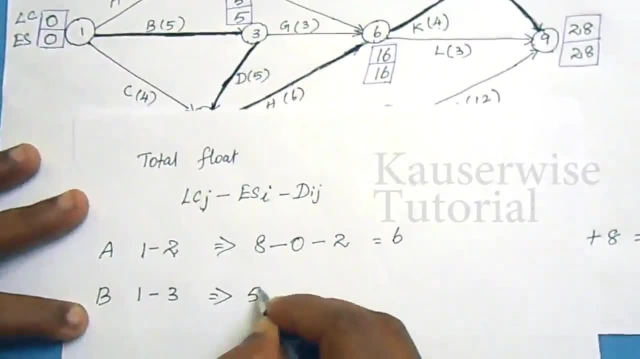 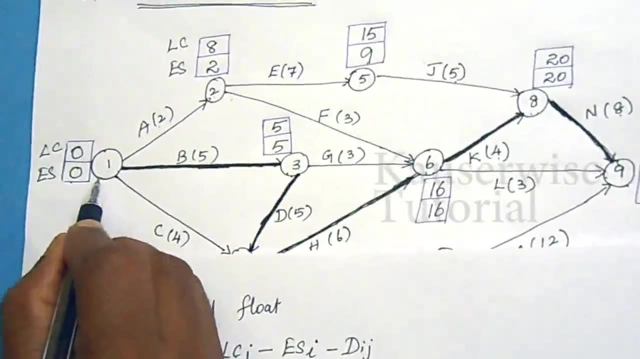 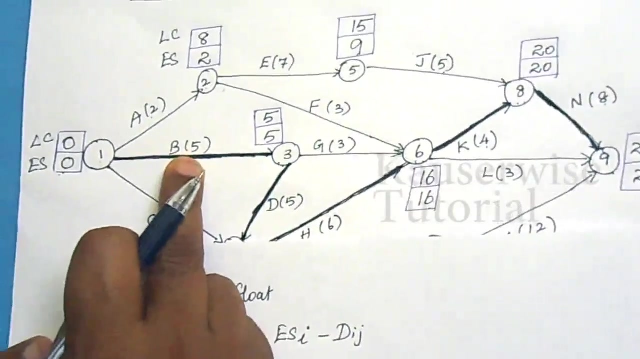 See. completion time is 5, 5 minus earliest starting time of a starting node. starting node is 1 node, so for 1 early start time is 0, 0 minus duration. activity b duration is 5, so 5, 5 minus 0, 5, 5 minus. 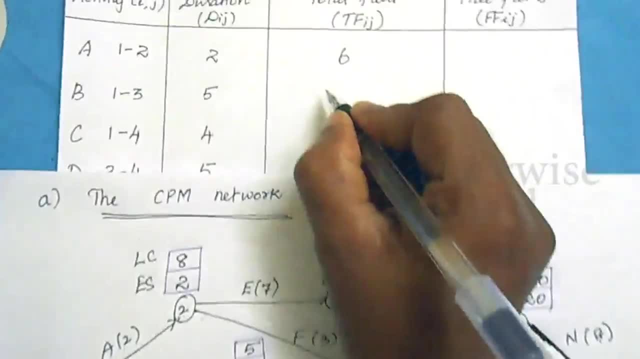 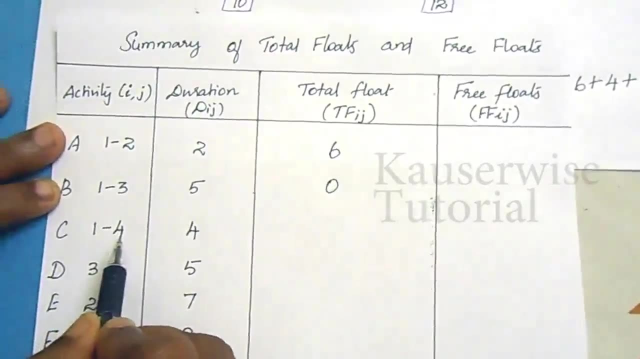 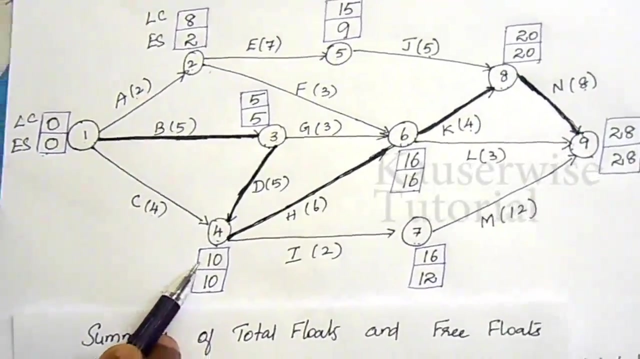 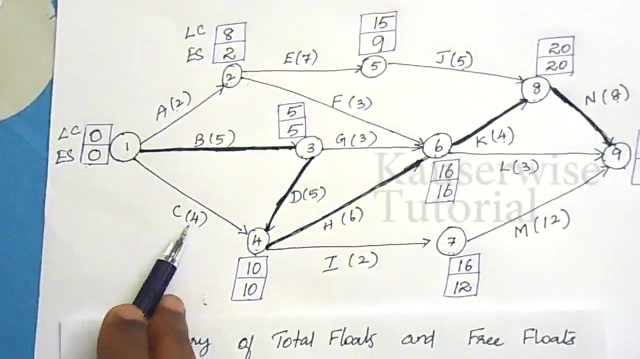 5: 0. okay, for b activity b, total float is 0. for activity c, that is, activity c is node 1 to 4. node 1 to 4. so latest completion time of ending activity is 10 minus earliest start time of starting activity is 0. so 10 minus 0 minus duration, that is 4, is equal to 6. 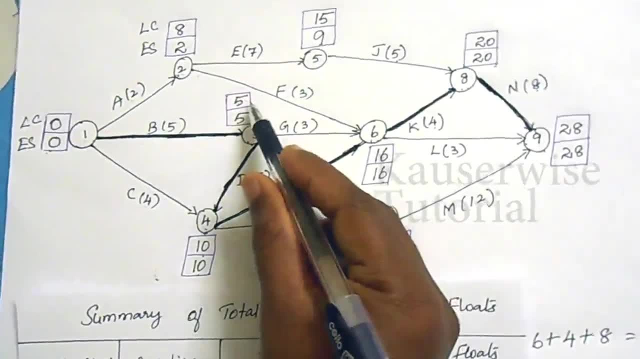 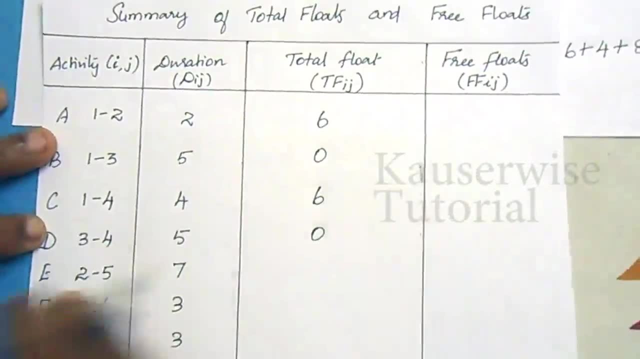 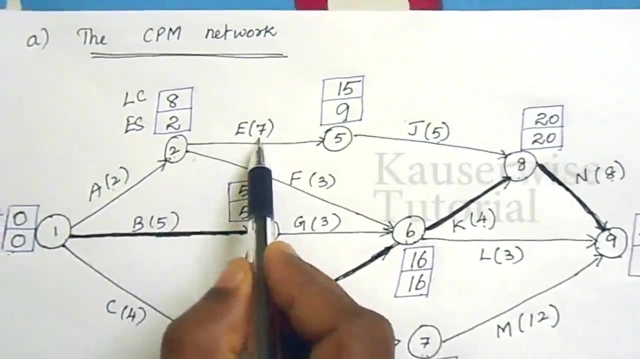 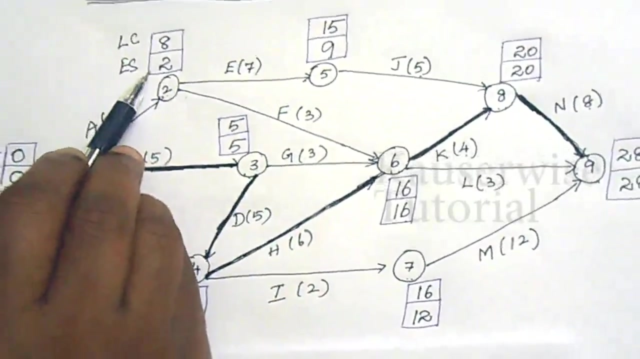 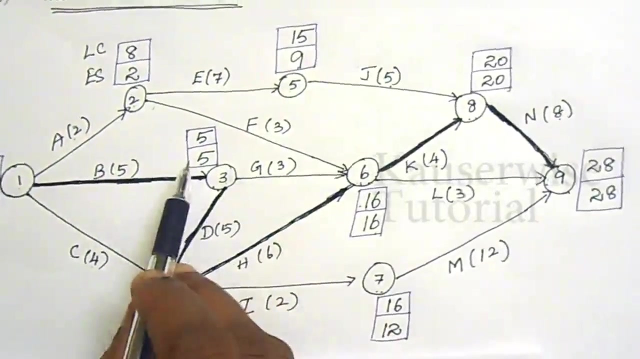 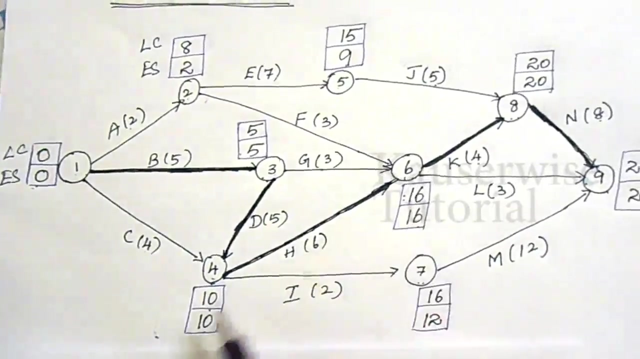 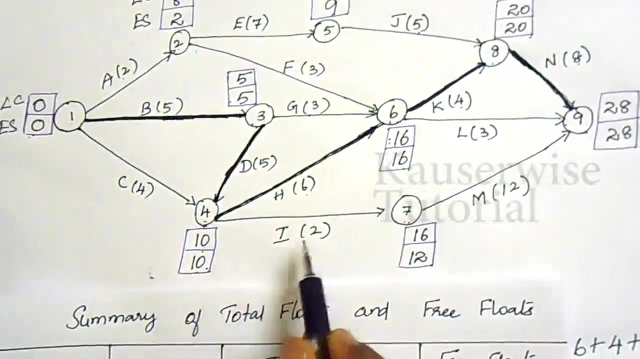 then for d: 10 minus 5, 5 minus duration: 5: 0. then for e for e: 15 minus 2 minus 7. 6. for f: 16 minus 2 minus 3. 11. for g: 11. for g: 16 minus 5 minus 3. 8 for h: 16 minus 10 minus 6: 0. for i: 16 minus 10 minus 2: 4. 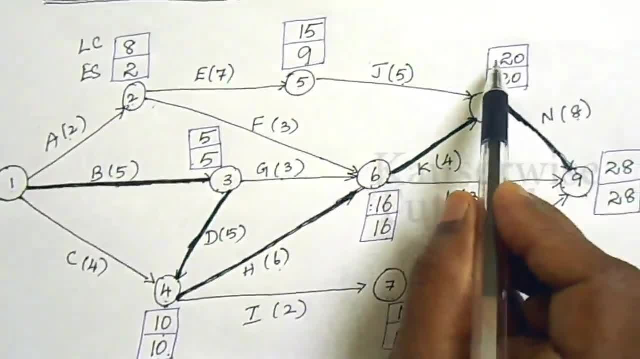 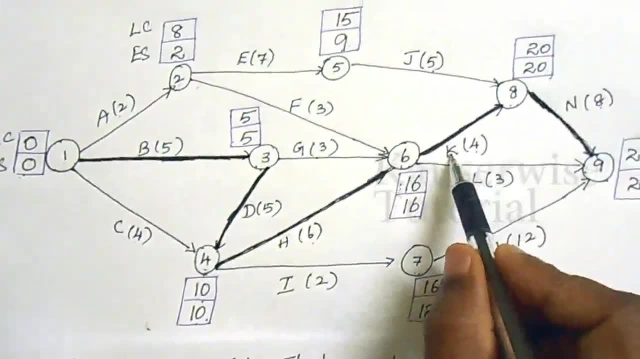 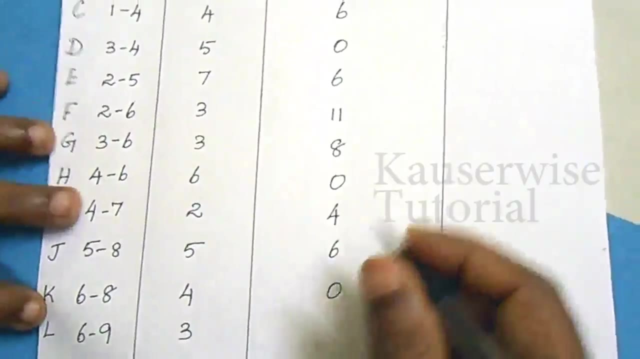 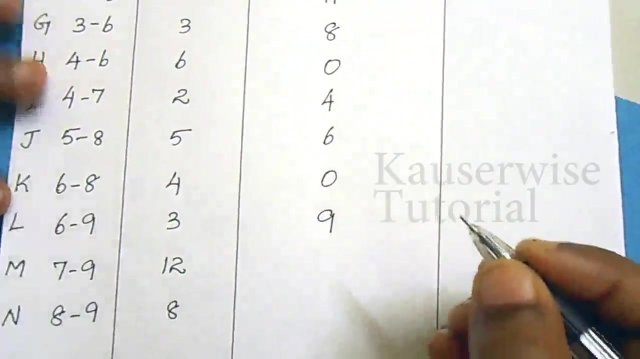 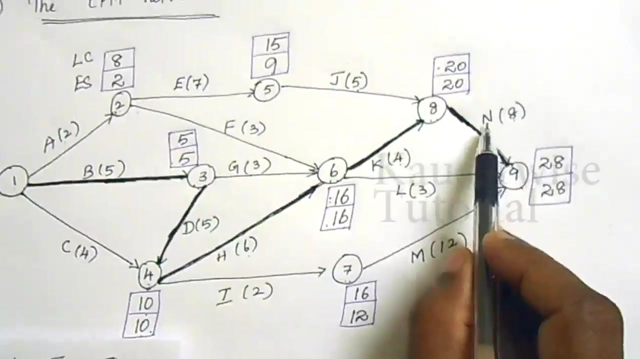 for j. 20 minus 9 minus 5, 6. for k. 20 minus 6, 16 minus 4: 0. then for l. 28 minus 16 minus 3, 9. for m. 28 minus 12 minus 12: 4. for n. 28 minus 20 minus 8: 0. 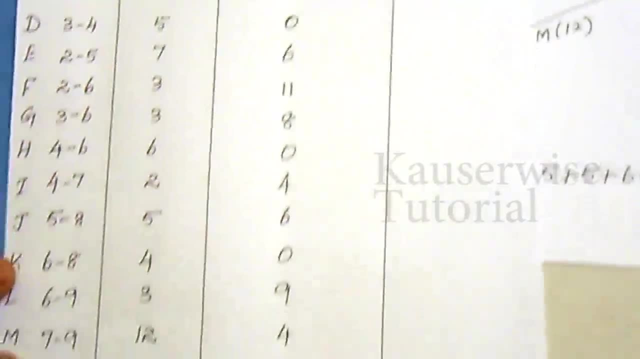 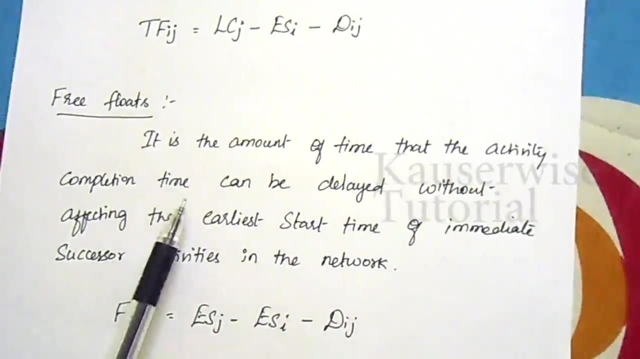 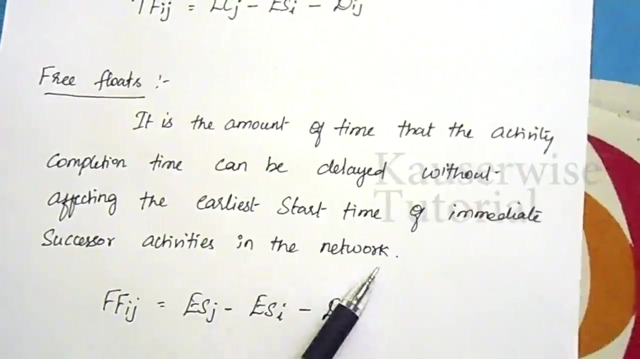 these are the total float for all the activities. then the next one is free floats. free floats means it is the amount of time that the activity completion time can be delayed without affecting the earliest start time of immediate successor activities in the network. so this is the formula to calculate the total float that is the earliest start time of ending. 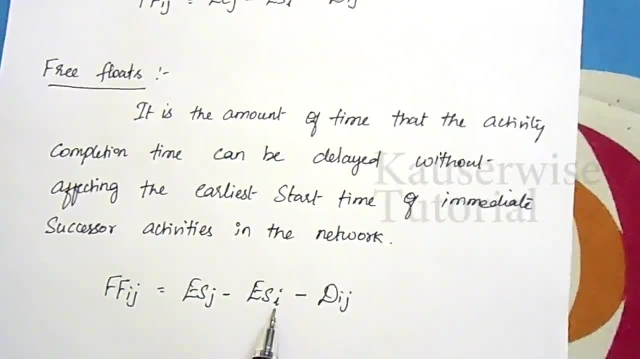 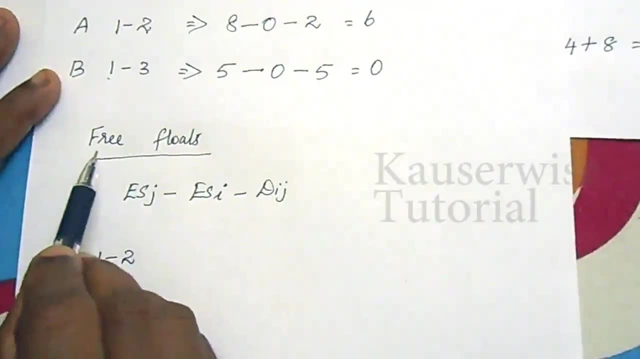 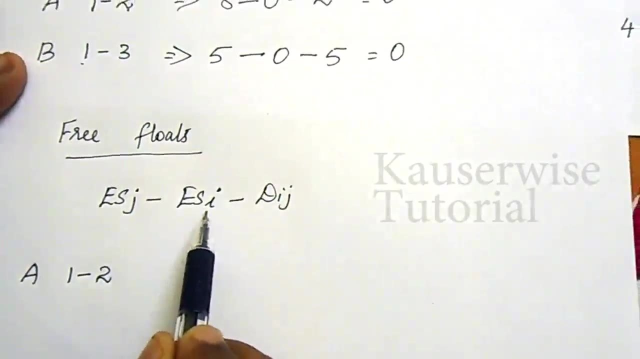 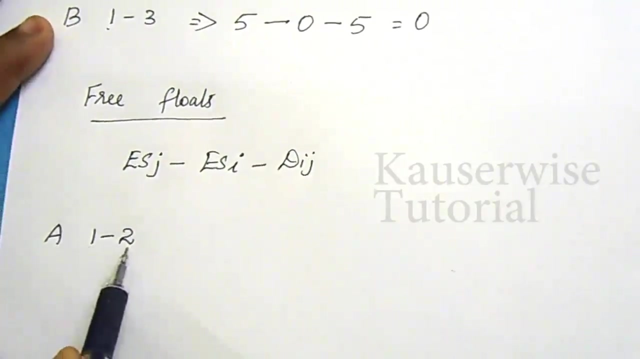 activity minus earliest start of starting activity, minus duration of that particular activity. now i'll show you how to apply this formula. okay, now calculate. the free float. formula is early startingỊrdsby the last node. then you add a new beginning election activity that is appeared when first node is chunked. 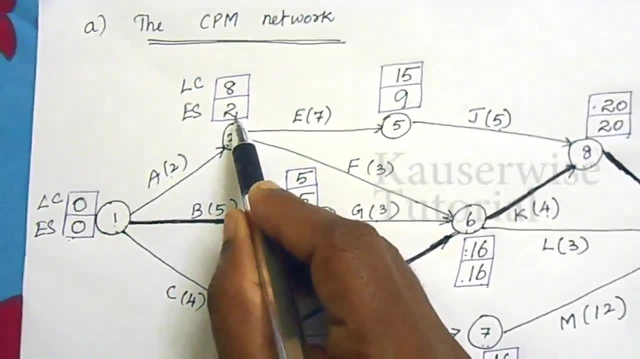 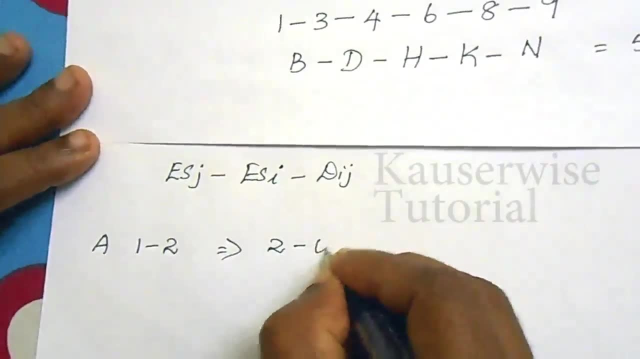 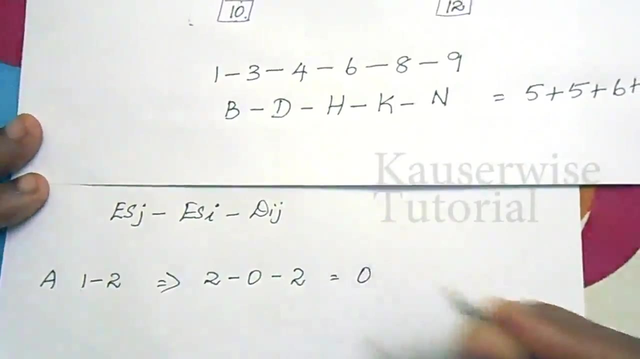 so this is the before node and the after node are summed up to 0 from a total float in the next code. Putting these all together, this will give you t01, which is the early start. lo with initial time. So activity A duration is 2, minus 2, you will be getting 0. 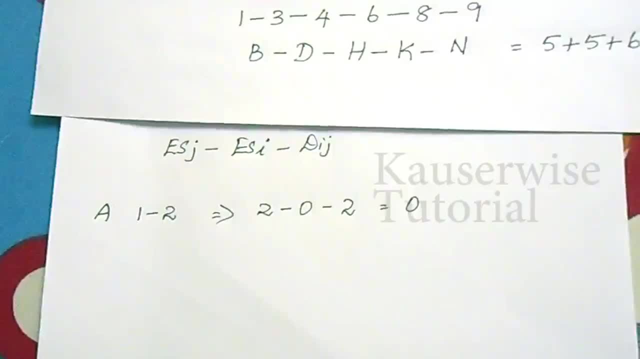 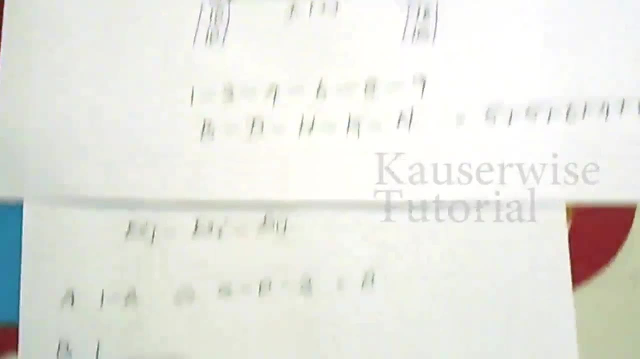 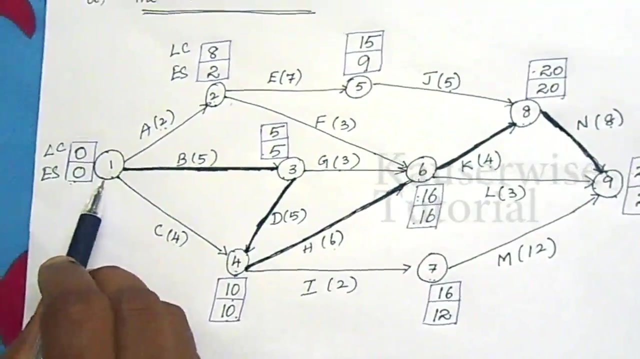 For activity A, free float is 0.. For activity B: starting node 1, ending node 3, 1, 3.. For ending node earlier start time is 5 and for starting node earlier start time is 0.. 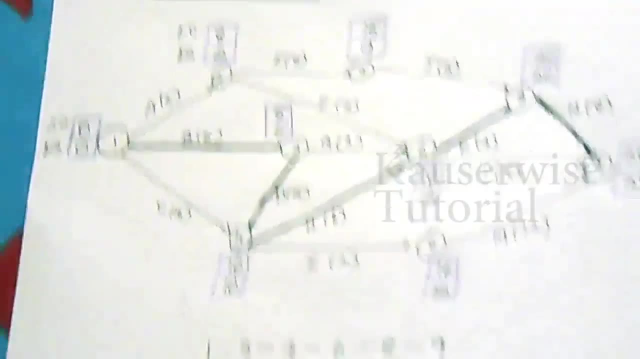 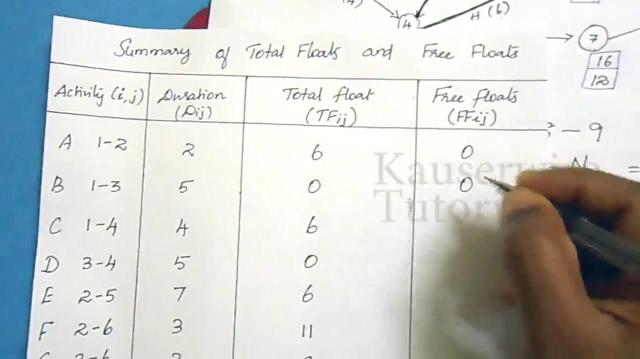 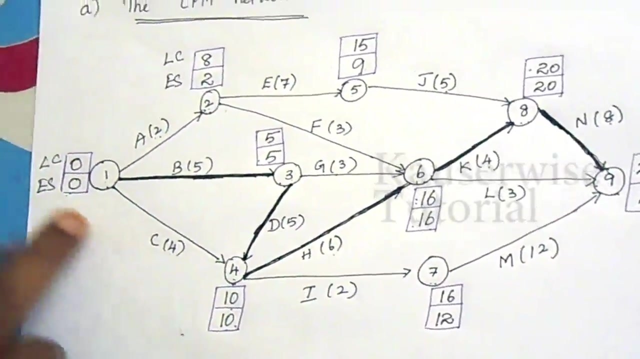 So 5 minus 0, minus duration 5.. 5 minus 0, minus duration 5, you will be getting 0.. For activity C: 10, that is early start time of ending activity- is 10.. 10 minus 0, minus 4, 6.. 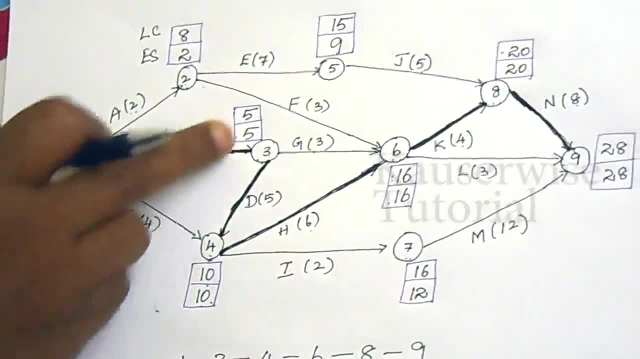 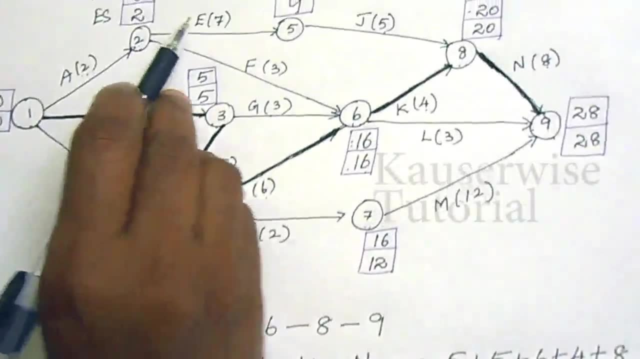 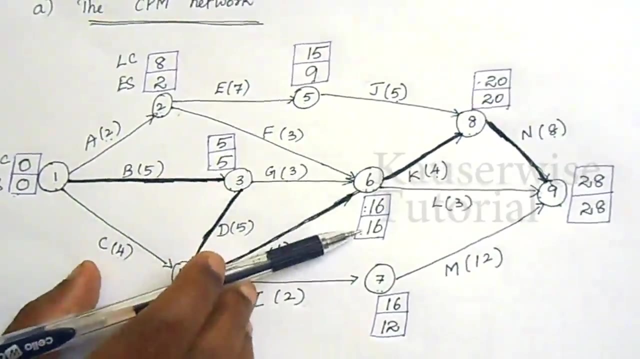 For D: 10 minus 5, minus 5, 0.. For E: 9 minus 2.. For E: 9 minus 2, minus 7, 0.. For F: 16 minus 2, minus 3, 11.. 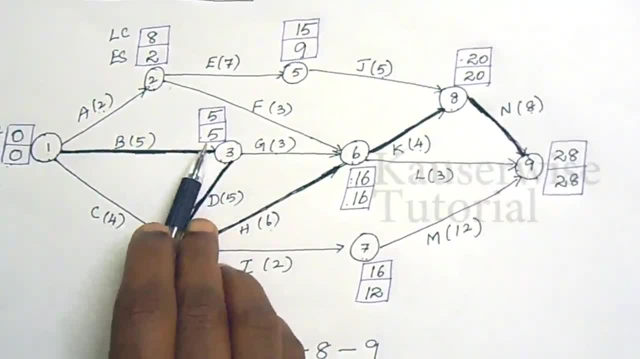 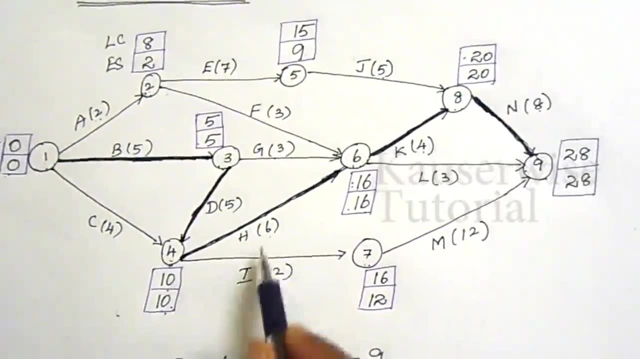 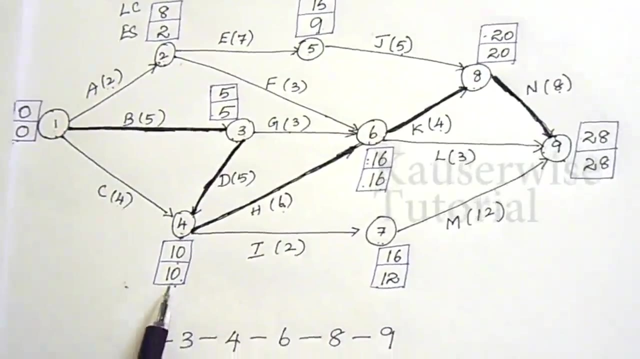 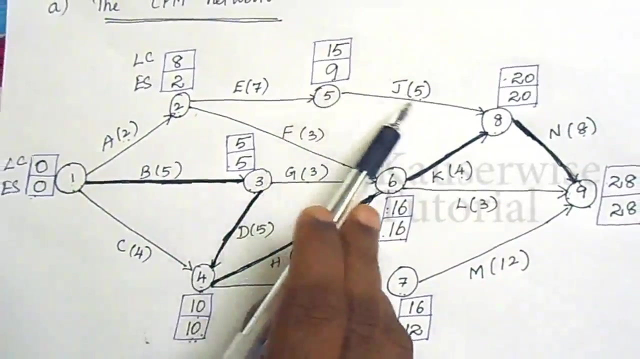 For G: 16 minus 5, minus 3,, 8.. For H 16 minus 10, minus 6, 0.. For I: 12 minus 10, minus 2.. For J: 20 minus 9, minus 5, 6.. 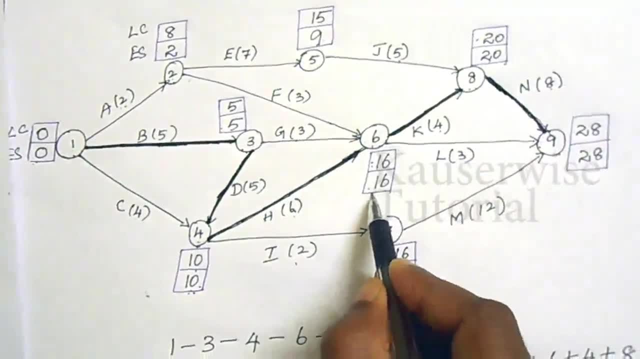 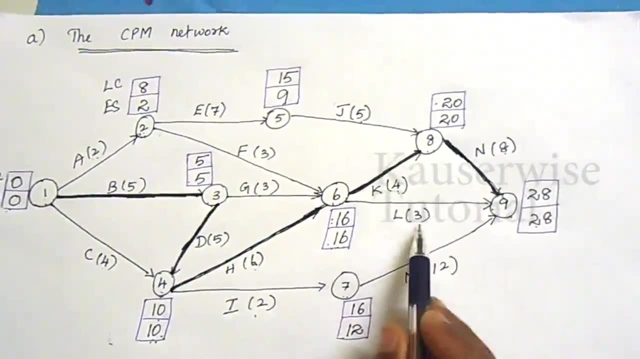 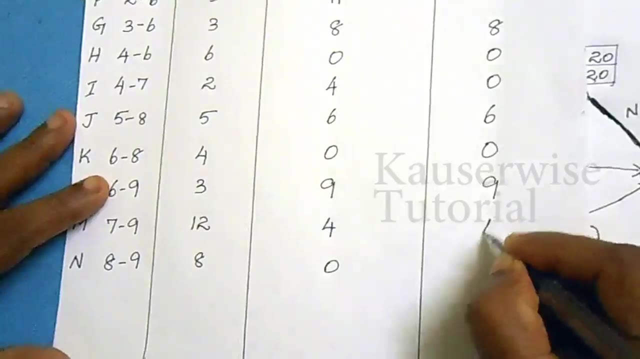 For K 20 minus 16, minus 4, 0.. For L 28 minus 16, minus 3,. 9.. For M 28 minus 12, minus 12,. 4.. For N 28 minus 20, minus 3, 9.. 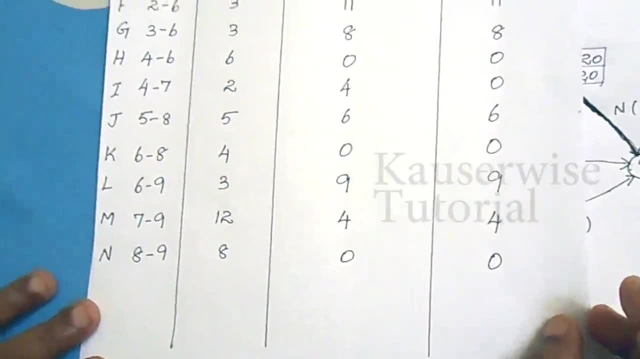 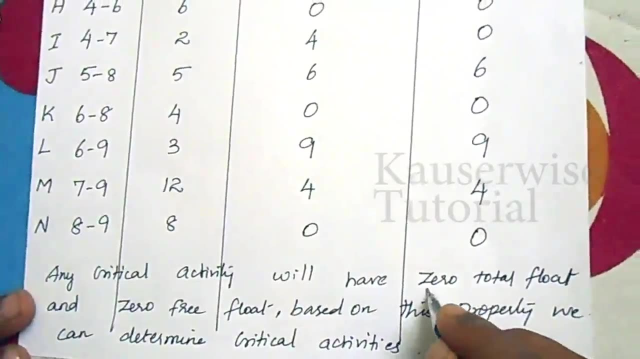 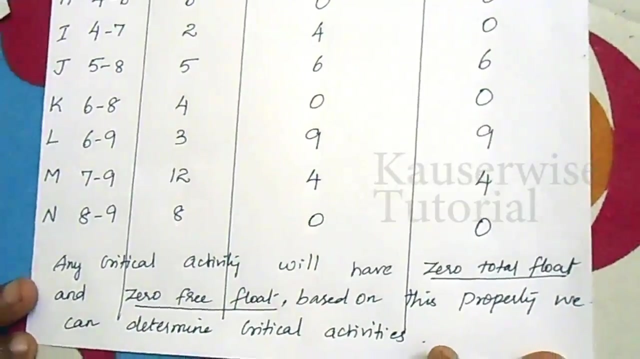 For W 28 minus 8, 0.. So now we have calculated free float for all the activities. See, any critical activity will have 0 total float and 0 free float. So based on this property we can determine the critical activity. 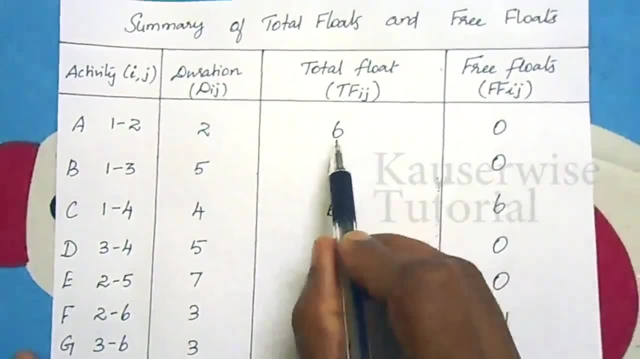 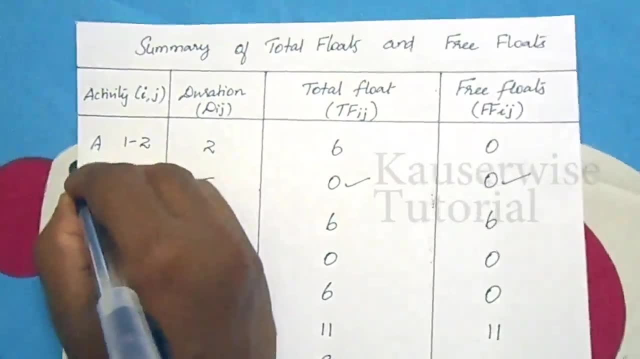 Just see the total float and free float: Here 6 and 0, it is a non-critical, And here 0 and 0.. So B is a critical activity, Then 6, 6, 0, 0.. 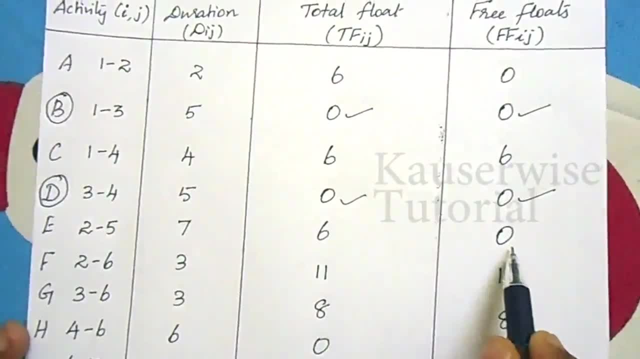 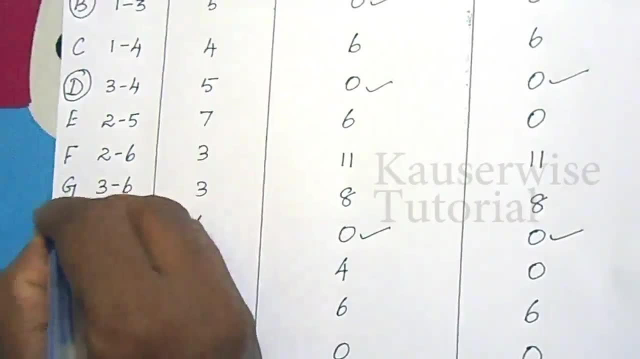 So it is a critical activity. 6 and 0, non-critical 11 and 11, non-critical 8 and 8, non-critical 0 and 0, so H also critical path, Then 4 and 0, non-critical. 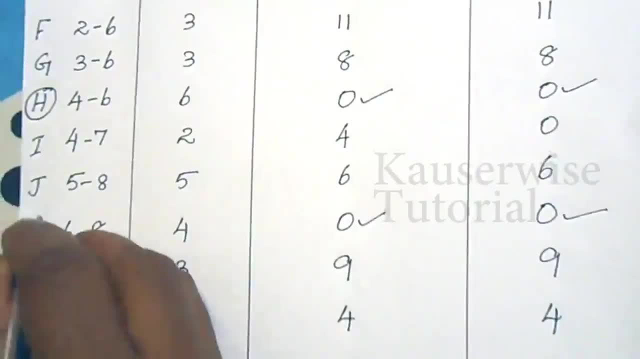 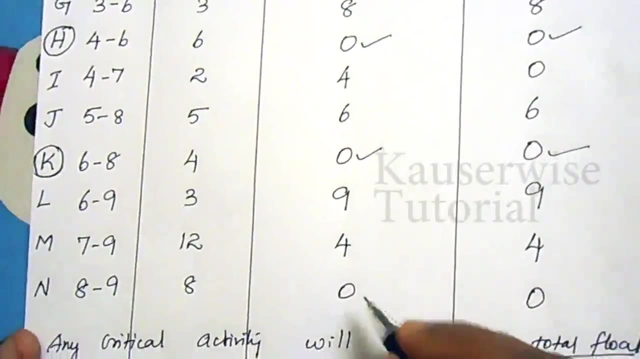 6 and 6, non-critical: 0 and 0, K also critical. Then 9, 9, non-critical: 4, 4, non-critical: 0, 0.. 0, 0, critical.